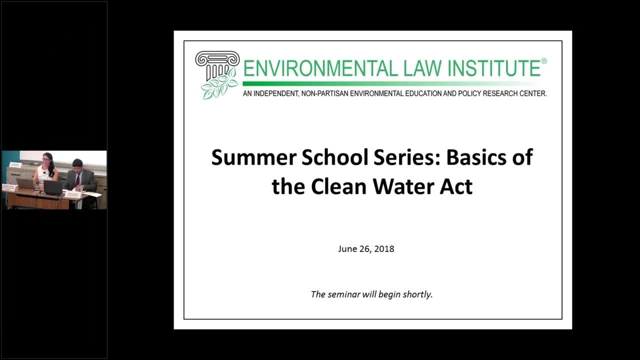 Welcome to the Environmental Law Institute. I'm John Pendergrass, Vice President for Programs and Publications at ELI. You've joined us for our Basics of the Clean Water Act, part of ELI's summer school series, and very happy to have everyone who is here in person. but 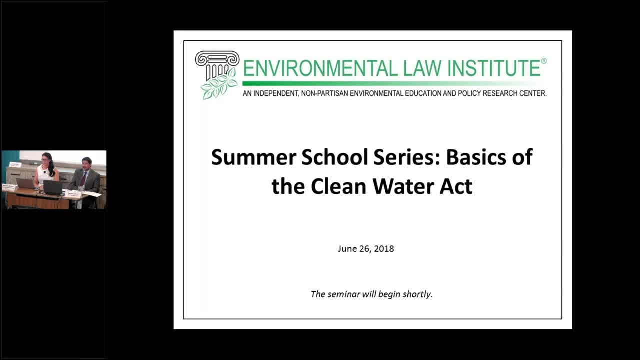 also joining us via webinar And I encourage you to follow our events page on our website, eliorg, for future events, particularly the continuing series, summer school series And for the members that are on the GoToWebinar. we encourage you to join us. 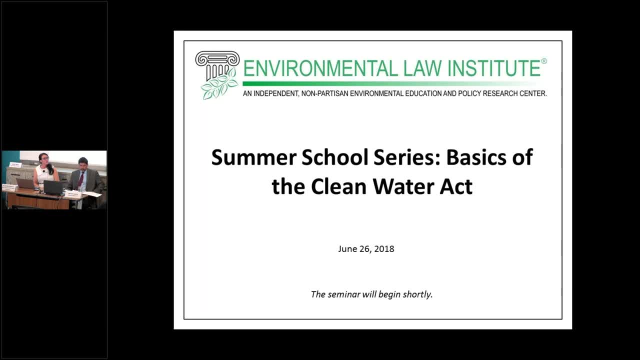 And we encourage you to ask questions, and you can do so in the question box on GoTo And, for those of you on the webinar, you don't need to hold them. As soon as you have a question, go ahead and put it into the question box, and then they'll be queued up for us. We really 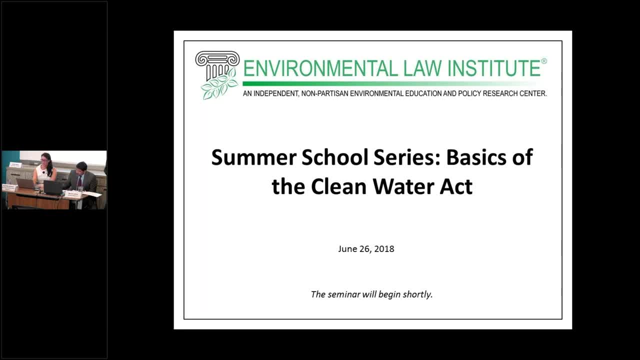 appreciate getting questions both from the audience in the room but also those on the webinar. We will have microphones for those of you in the audience. These are not – they're so that people in the webinar can hear you. They don't amplify just like the one that 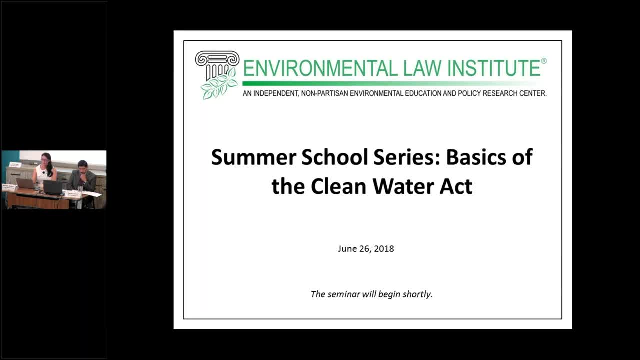 I'm wearing is for them to be able to hear. So I'd like to thank our wonderful panel for being here today to teach the basics of the Clean Water Act. This will be recorded. It'll be available, along with the PowerPoints, within the next. 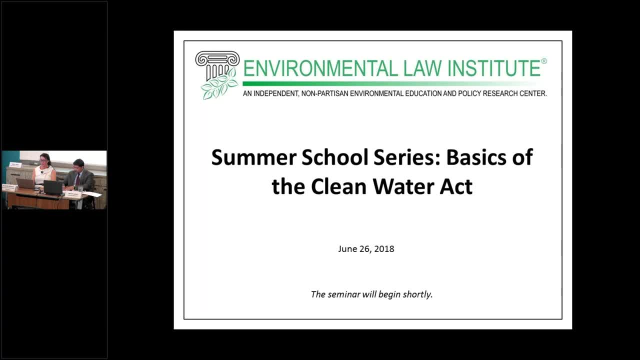 week And I encourage you to look at the full speaker bios that are on the website. But briefly joining us remotely, we have Elizabeth Andrews, professor of the practice of law at the University of Michigan. She's going to talk a little bit more about the Clean. 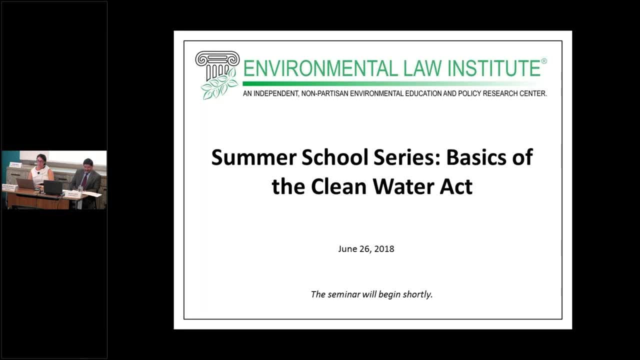 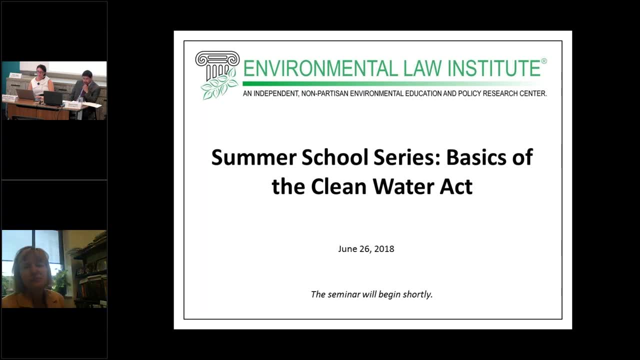 Water Act. Elizabeth Andrews, professor of the practice of law at the University of Michigan and director of the Virginia Coastal Policy Center at the Marshall Weith School of Law College of William & Mary, and Kathy Robb, principal at CyPaget and Rizel. both will be online. 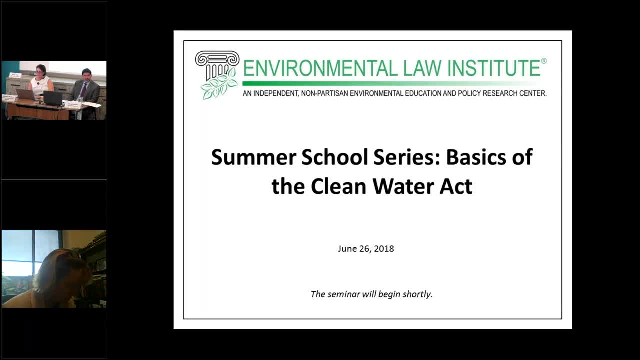 So thank you both. And in the room next to me, David Lastra, regional criminal enforcement counsel, EPA, Region 3.. And Amanda Waters, general counsel at the National Association of clean water agencies. thank you both for being here with us. so with that, we'll start with david. 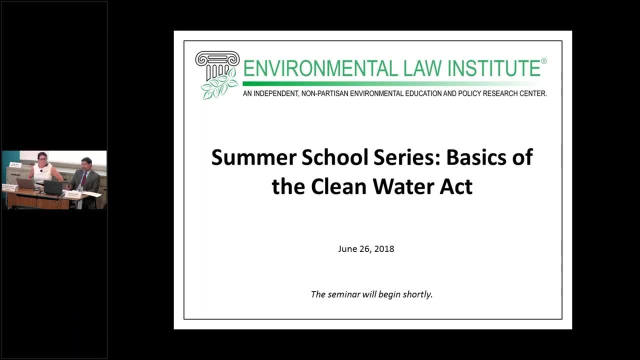 all right, thank you again. my name is david lastra and it's a pleasure to be here. thank you to the environmental institute for having me here. i was actually. i'm actually substituting for a colleague of mine who was unfortunately not able to join today. the presentation that you will see is his. 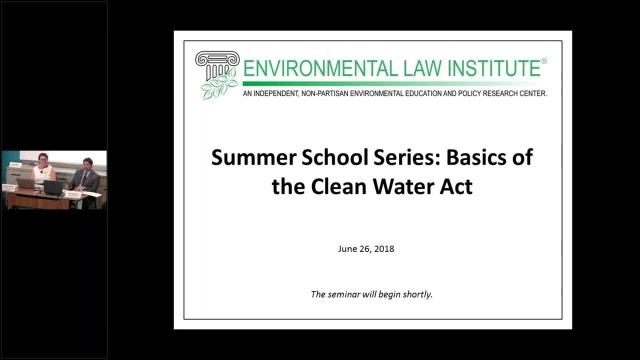 urn, and so basically, it is a rogue a uh, but what that means is that we work with the mpi and our staff, and we are working with the mpi on many different aspects of the project, and we are working with the mpi on several purposes, but all the credit goes to me and i'm always starting to get credit for somebody else's. 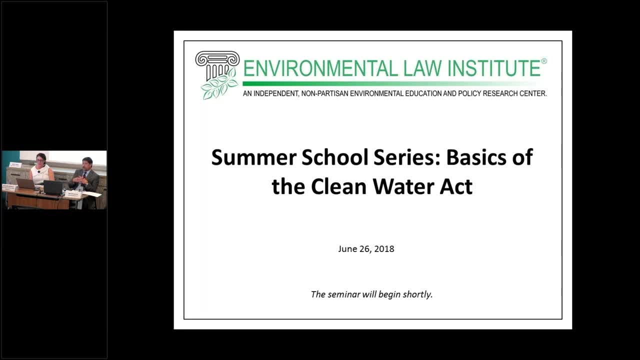 cases to the Department of Justice. that's what I do. I'm not an investigator. I'm an attorney that supports the criminal investigation division. it's a fun job. it's a an incredible opportunity to protect the environment. the criminal investigation division, of course, is dealing with the most egregious. 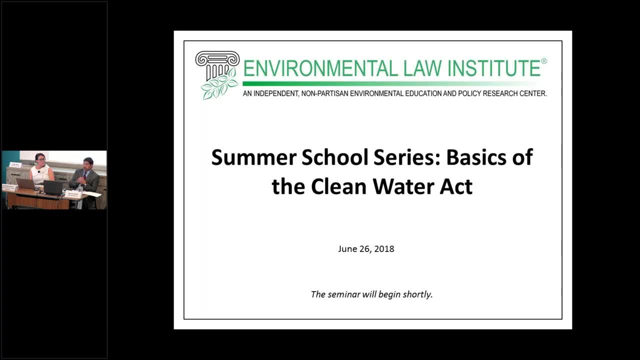 violations. a great part of my job is dealing with the Clean Water Act. do enforcement. the presentation is more of an overview, so I'm going to give you an overview of the act, but I'm also going to talk a little bit about the enforcement side, which I think is kind of fun. I would say that the Clean Water 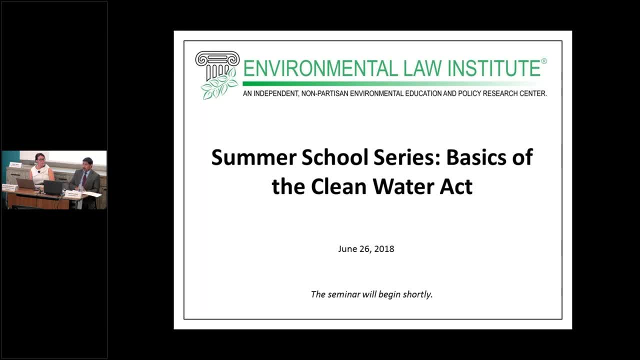 Act is probably one of our most powerful statutes. if you are thinking about violating the law in terms of the environment, I would advise you not to do it. not to do, you know? mess up with the water. it's interesting, as humanity has an incredible affinity for water. we all love it. we all like to swim. 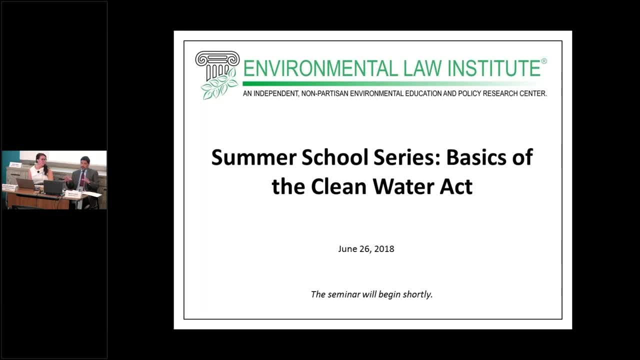 recreate the water- we love it. the environment, we love it, the environment, fish, and I think that's part of sort of the reasons why we have such a powerful statue. we'll talk a little bit about the history, how it was created, and again, this would be more basics. if anybody have questions about it, please you can. 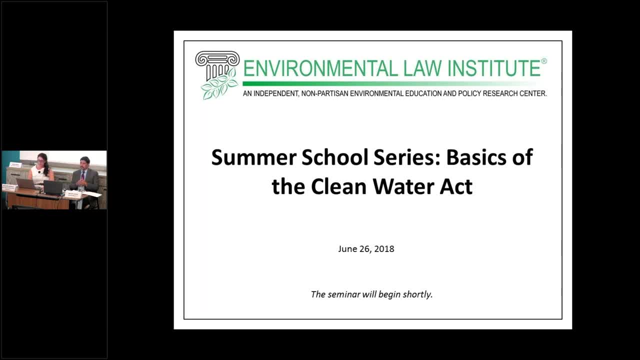 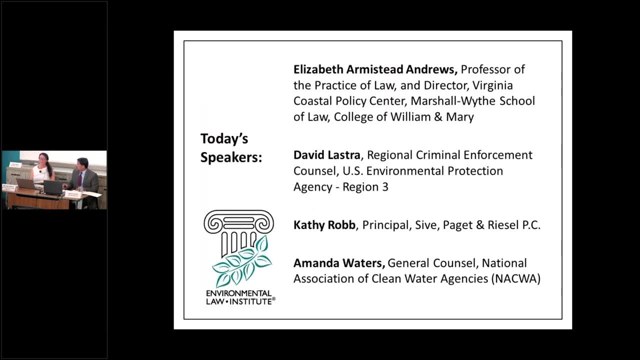 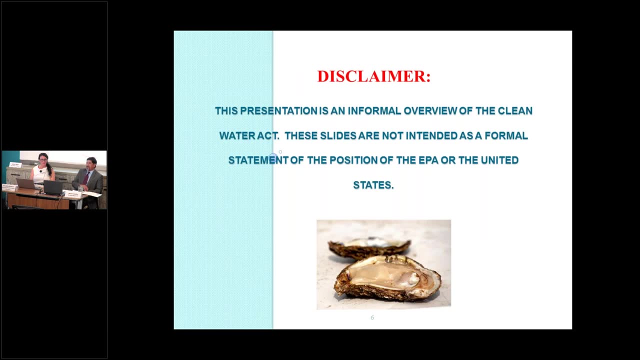 interrupt me now or while I'm doing the presentation, or write your questions and we will address them at the end. okay, so, having said that, all right. again this presentation. I have to read this: it's informal overview of the Clean Water Act and the slides are not intended as a formal statement of the position of the 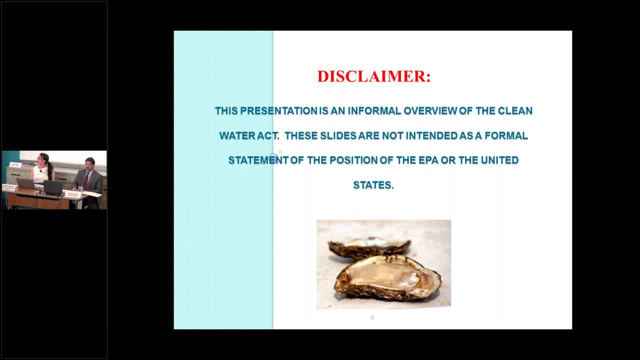 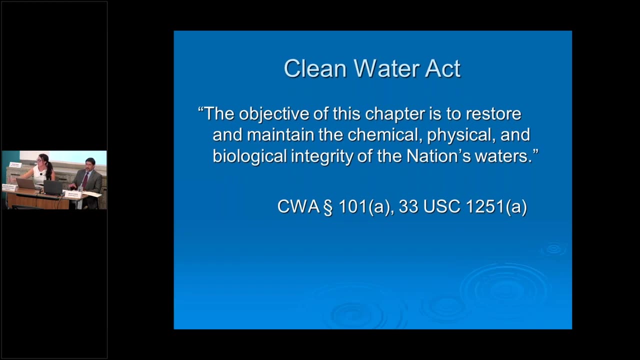 EPA or the United States. I'm required to say that, even though I'm here basically in my official capacity, I am an attorney, I represent the agency. it's a great job and I really enjoy it, and you'll get to see some of that. so how do we start? so if I go in the area 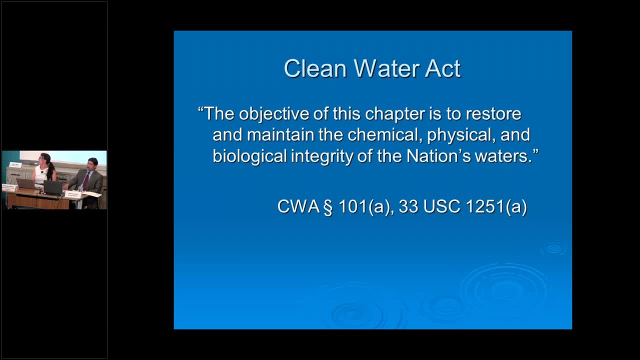 of enforcement. this is one of the critical things that you will learn today. what is the objective of the statute? why is it that we created the Clean Water Act? this is going to be our focus throughout all the slides, throughout, all through all the things that we're going to be talking about. 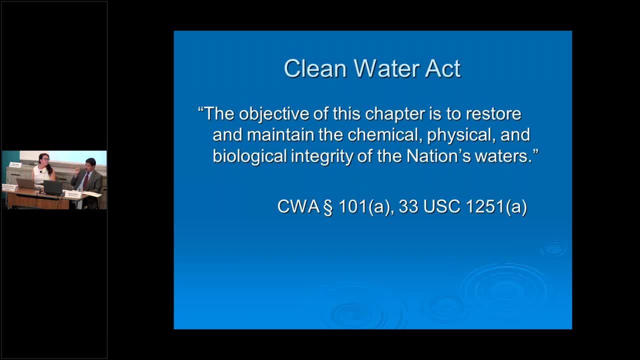 today. I can tell you that they're based on this particular objective, which is to restore, restore and maintain the chemical, physical and biological integrity of the nation's waters. now we'll see how that relates to water quality standards, to criterias, to anti-degradation policies. so how do we address that as a effective and more practical? we'll address it a little bit. 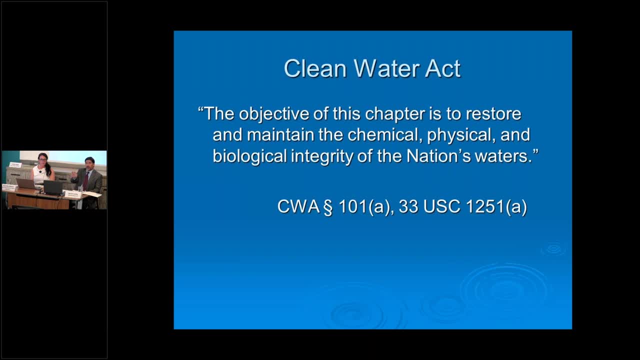 but this is sort of your aim if, um, i think one of the important lessons here is: what is it the objective? and that's going to be your focus when you're dealing with cases regarding the clean water act and if you see particularly indictments or complaints that epa files against individuals. 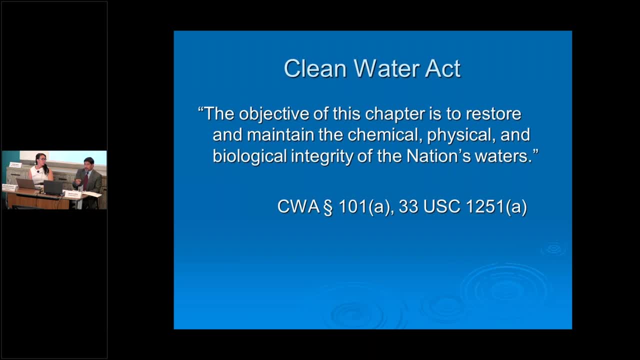 or corporations. this is one of the first allegations, so you may have an allegation about jurisdiction. the second or third allegation is going to be: what is the objective of the clean water act, because that's our focus. does that make sense, right? uh, this is sort of the structure. how. 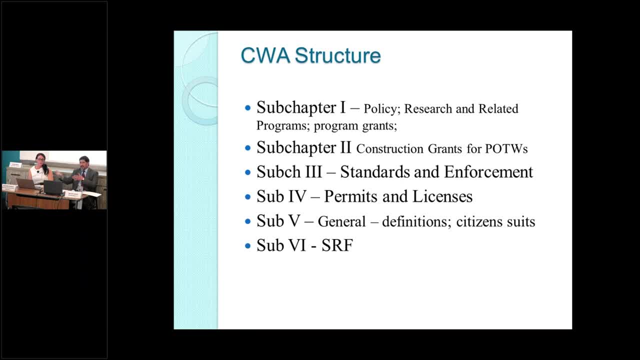 we divide into chapters. uh, it's called titles. if you look at the um codified version of the queen or argue, we're talking about section 309, for example, or 304 or 302, uh, and the title word will be 33, usc, section 1301. let's go. 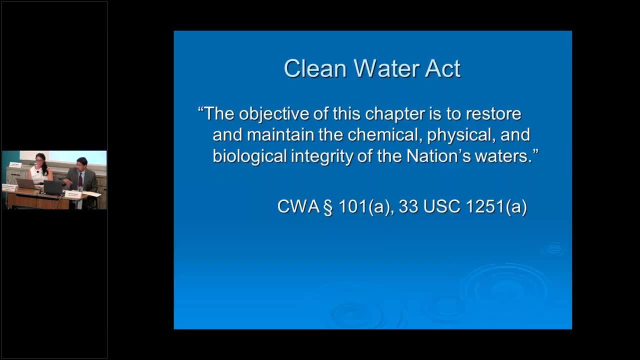 back to that one. so you see, the codification will be under the chapter 33. uh, the us code section 1251 is the first one and you go from there all the way into section 302 where it says we typically in the in the practical world, we use the: 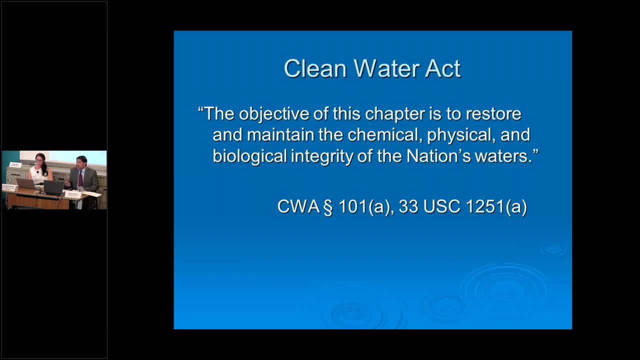 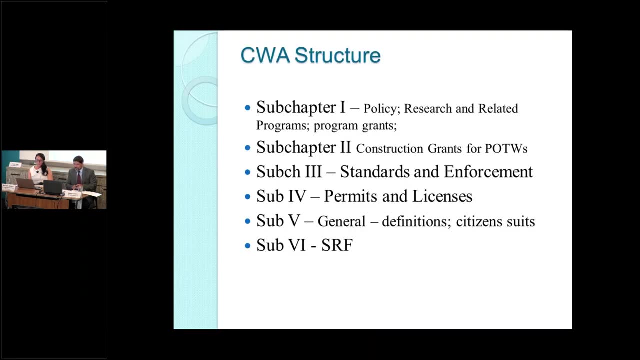 us code sections. uh, instead of you know you will see in some some of the slides what is section 302, you will need to look at section 3, 11 i believe, or 312, 13th problems. but anyway, going back to the subchapters, the first one addresses sort of policy, how to do research. what are the 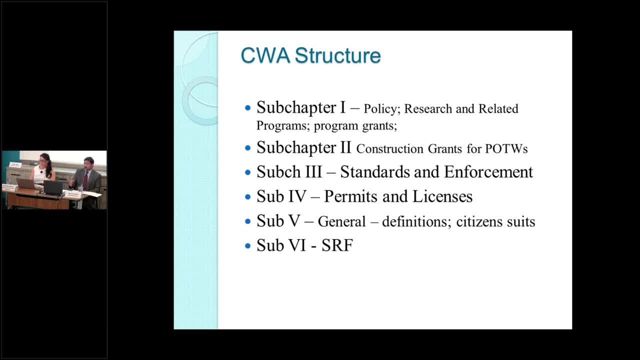 program grants. the second chapter was a big chapter on in the environmental world, in the clean water act world, the construction grants for potws. that has been phased out and is now what we call the sub chapter. uh six, which is the srf, and i'll talk about that in in a second. uh, the standards and enforcement is what i do most of the time. 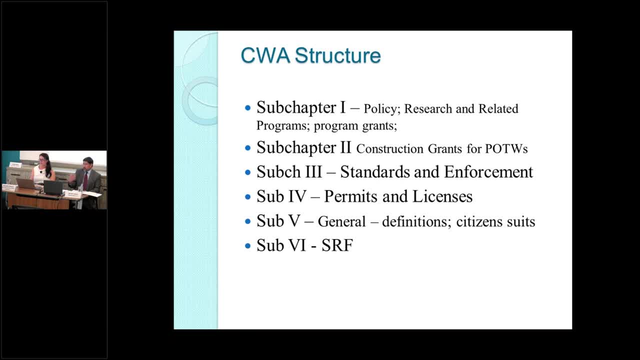 enforcement, um of this, that this you know, particular provisions of the clean water act, permits and licenses- i think amanda is going to talk about uh. and then, of course, we always refer back to the general definitions, like what are waters of the united states, which are not necessarily well defined in the statute. what is a point source? what is a non-point source? 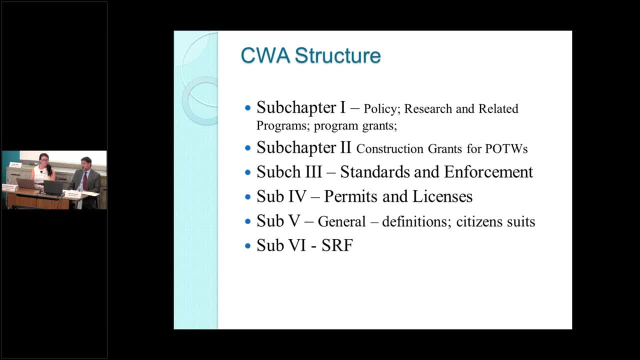 discharge. uh, what are pollutants? um, and i can tell you, in the clean water act, a pollutant is basically anything that is something other than water. so if you're discharging water, that's not a pollutant. if it's just charging anything, even water, that is. 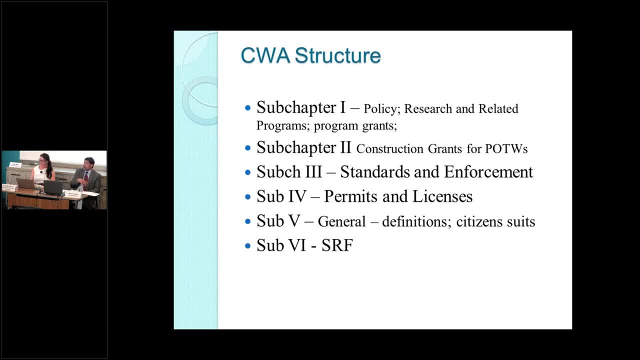 warm, you know, to a certain degree, or water has a particular ph, or oil or sewage, those are all pollutants. so it's a very strong um, very um helpful, i would say. definition of pollutants. uh will address some of the other definitions that are more problematic later. all right questions about that. just the general structure. 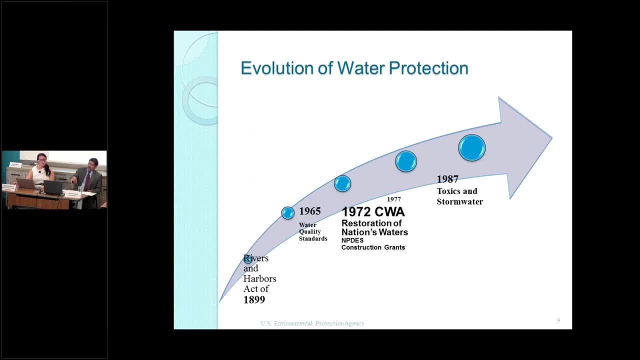 all right. so how did we start? so it's neat because the first environmental statute in the united states was the rivers and harbors act of 1899. it actually has criminal provisions, as you might be surprised. in fact, i have prosecuted several individuals using the rivers and harbors act. it's still good law. it carries a mandatory 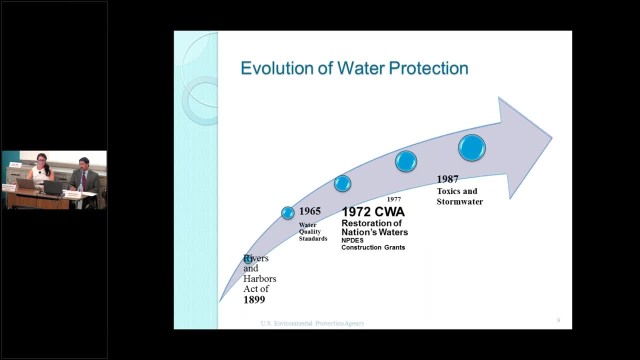 term of incarceration of 30 days, which is unusual for somebody to address, that they are thinking: wait a second, and one of the neat things about it is strict liability. so if you um mess up with the rivers and harbors act and we can prove that you uh did it, and we'll talk a little bit about what it. what is uh, what it constitutes uh. 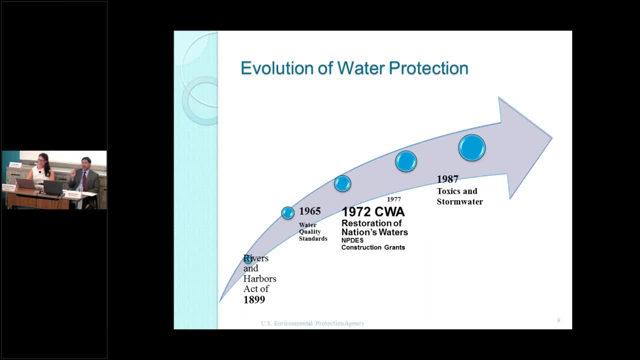 a violation of the rivers and harbors acts, but the neat thing about it is that it was the first environmental law statute. it does provide for criminal. it's a misdemeanor. uh, so it carries a term of incarceration of up to a year, but it does. there's a term in the statute that reads: 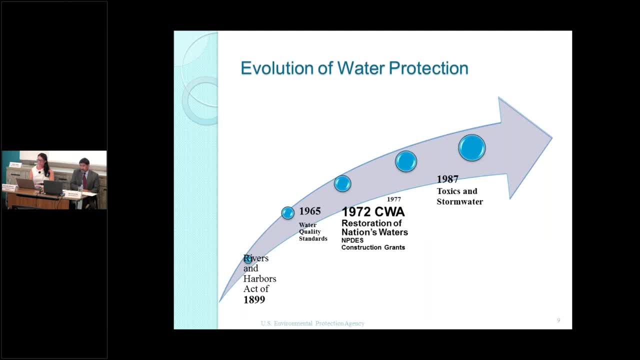 a minimum term of 30 days, and i have actually been successful in doing that. so has epa and other conflicts. from there we go to 1965, which was the first environmental law statute, and i have been successful in doing that. so has epa and other conflicts. uh, from there we go to 1965, which was 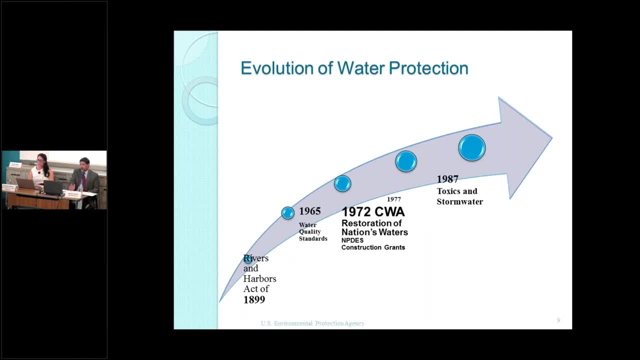 the first water quality. it was the first federal water pollution statute that addressed that directly- the water quality standards directly. it really did not have that much teeth. it wasn't that useful in terms of enforcement. it's not until 1972 that we talk about the more critical aspects of the clean water act, which are 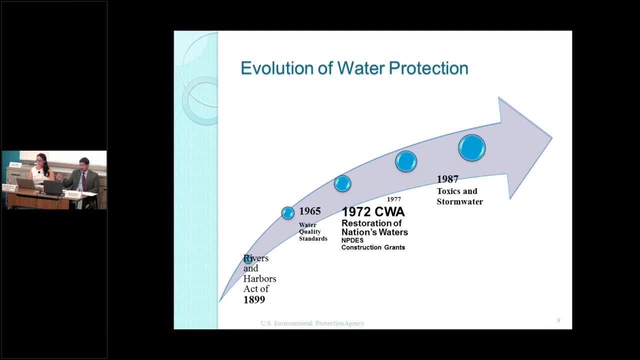 pollution, the discharge and dealing with pollution, discharges. right. that starts in 72, right in 77. there are amendments in 87. there's amendments as well to address the toxics and storm water, which is, i think, amanda's going to talk about. all right. 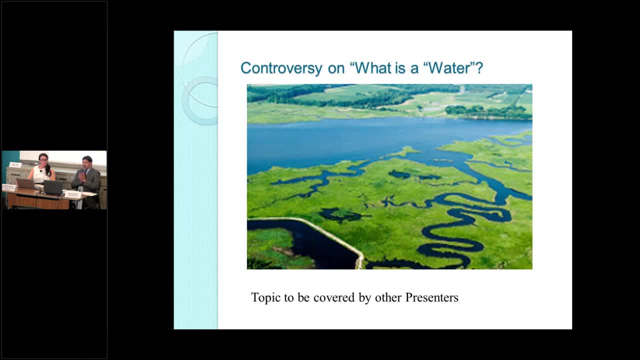 so one of the bigger controversies that you'll hear about today is: what is a water? so, for example, one of the things that i do is that, like, if somebody is discharging a pollutant from a point source into a water of the united states without a permit, they're committing a felony. 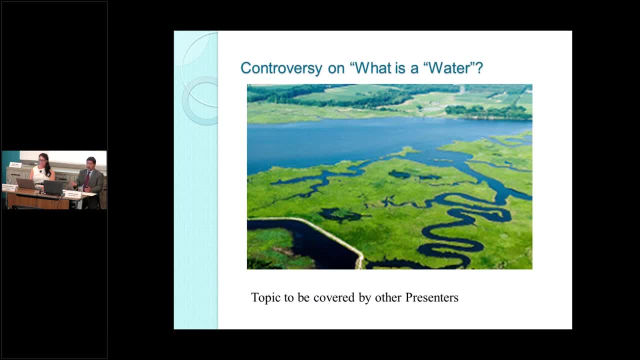 as you know, the knowing discharge so intentional, not as a result of a mistake or an error or an accident, but if you're knowingly discharging a pollutant from a point source- and we'll talk about what point sources are- um into a water of the united states without a permit, you are committing. 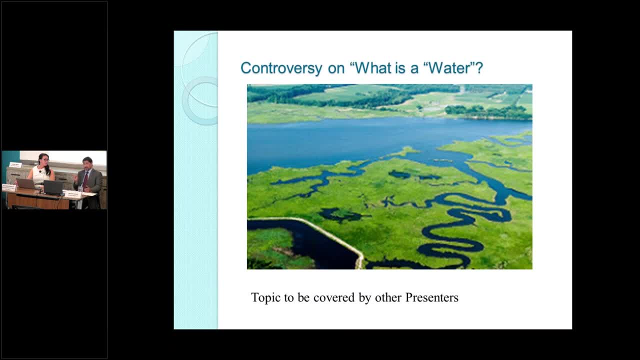 a felony. now, what are waters of the united states is something that has been the subject of much controversy. uh, very recently, uh, starting with several cases, then went to rapanos. uh, we will talk about what rapanos, the rapanos uh supreme court case, talks about, and it's a question. 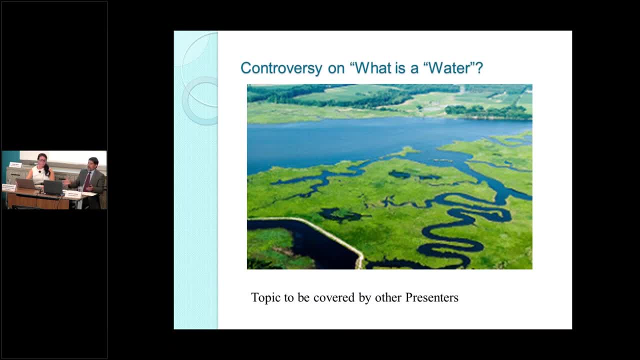 about the nexus between the navigability of a water and the water that you're dealing with. so if it's a small creek and there's not not necessarily a significant nexus between that creek and a navigable water, uh, and navigability means that you can put a boat and sort of go. 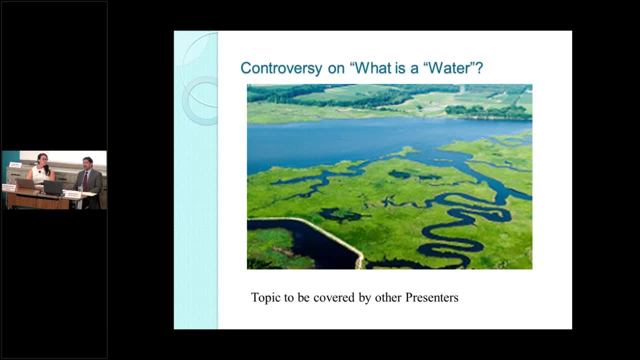 around or a kayak. i guess you can say: uh, so if there's not that nexus, then you may have a problem of showing that we're talking about waters of the united states. uh, and then somebody else is talking about this as well. right, okay, okay, kathy, that's on you. um, all right. 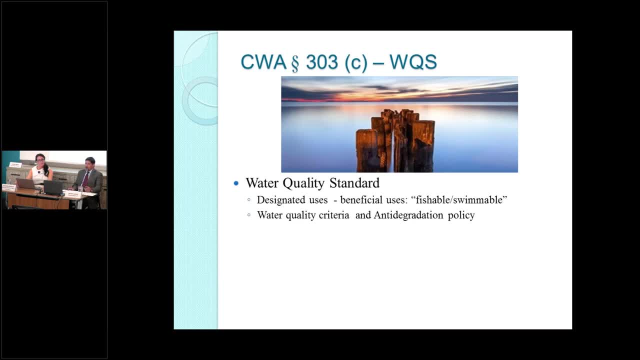 so water quality standards? um so the clean water act is a neat statue because it defines. one of the aims is to address the water quality standards of our waters. right, so how do we address the water quality standards is by three criteria's. one is the designated use. the second one is the water quality criteria. that 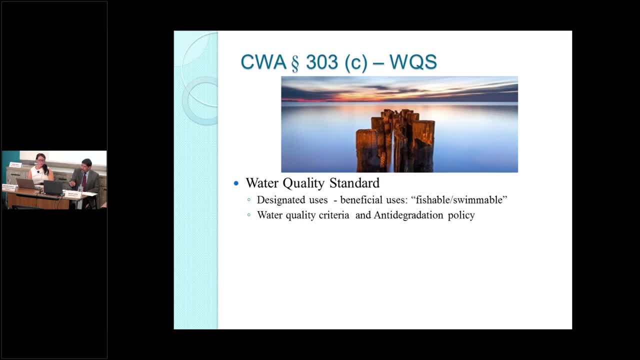 would address how we qualify the, how clean the water is in order to be used for that designated use. and if the water quality is really high, then we have certain provisions to make sure that is not degraded. and that's what those are, what we call anti-degradation policies. 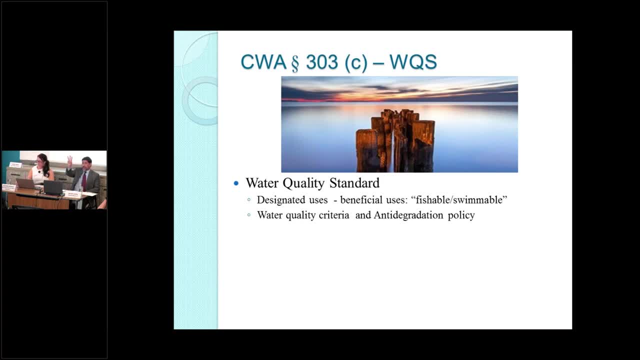 so, again, we measure our quality standards by three things: designated use, for example, we say we're going to be able to swim in this particular creek or lake or river. we want people to be able to fish in there. and once we designate- and these are the states that are typically designating- 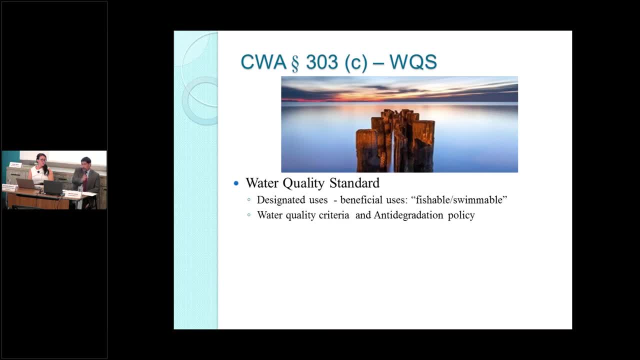 these uses, then we, the agency and with in conjunction with the states, develop water quality criterias. that would be a measure of how clean this particular water is in relationship with the use. so we may establish certain ph values, we may establish toxicity values, we may establish how many discharges can go into that particular water, water body, based on the designated use. 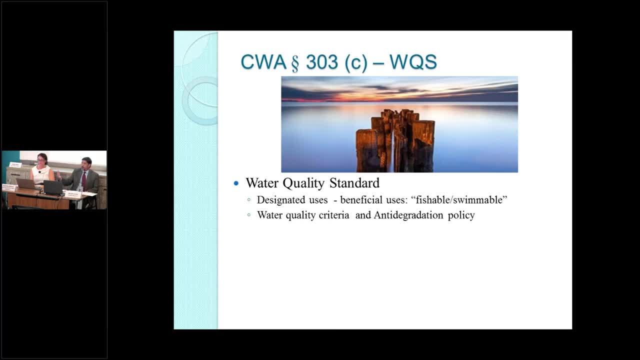 everybody following me. it's a very straightforward way of doing it and, if you think about it, how else can we measure whether or not we're being effective in protecting a water? it's, that's the idea. the idea is, you have to have effective, objective criteria in order to 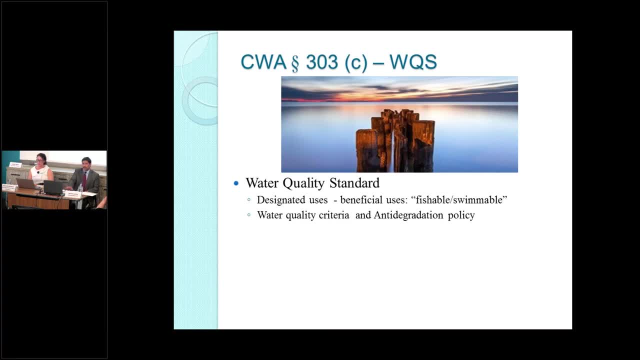 decide whether or not this particular water body is cleaning, if you will, and that's how we do it, and this is a true not only about the clean water, but other statues in the environmental world- the states have really the primary responsibility to address and develop this water quality. 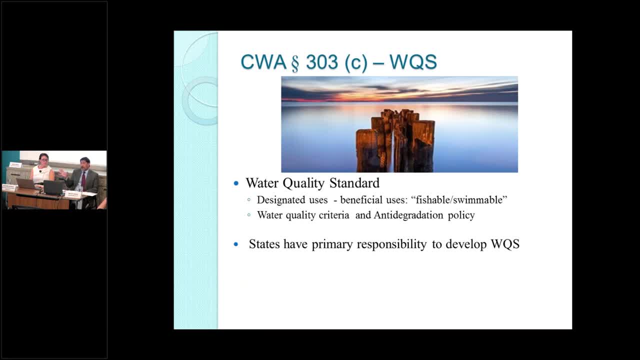 standards. now the epa still has the enforcement authority to make sure that the states are actually following with what they say, but it's really the states who are primarily responsible from doing for doing it. and we provide grants. the epa provides grants, provides, uh, the ability and 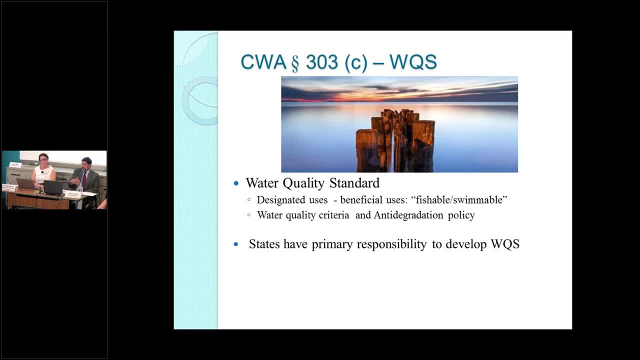 you know, sort of oversight to the states. uh, one of the ones that we're going to be talking about is the chesapeake bay, is a great example how we address a particular problem and we're extremely successful, in my opinion, on, uh, restoring the quality of the chesapeake bay. so 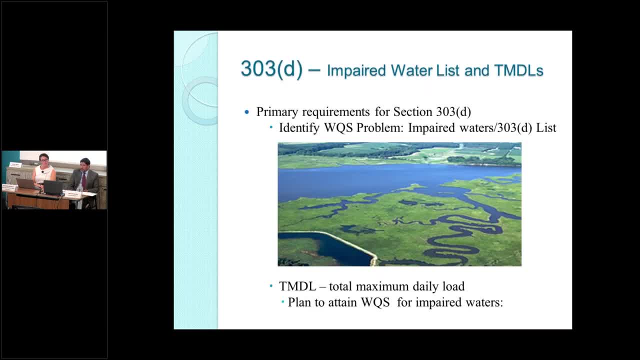 all right. um, i think i covered this already, so this, um, let me go back to the total maximum daily loads. it's one of the ways that we address, uh, the clean water. is somebody else also talking about this, or talk about it a little bit? okay, so, 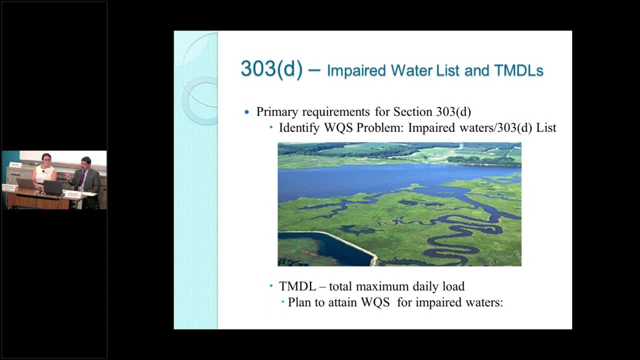 basically, we identify areas that are problematic in terms of water quality standards and we decide which one of those waters are impaired and we generate the list, and when i say we mean the states and epa. we generate a list of those areas that are impaired and we address those with a 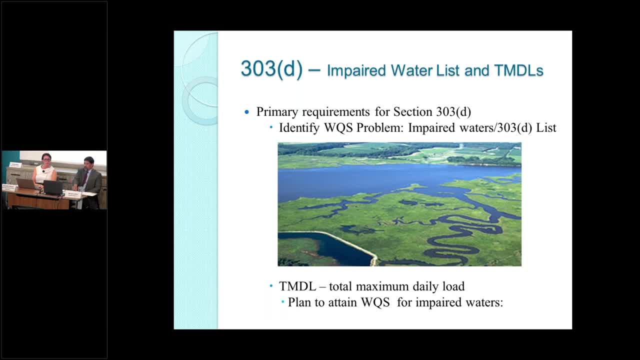 particular tool. we call this tmdl, the total maximum daily loads, and that is just a way to address: how many pollutants are we going to allow to go into this particular water body? based on the quality, based on the quality standards, based on the uh- the designated uses um- and based on the 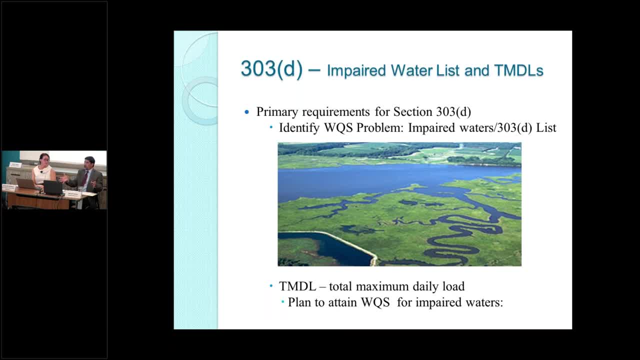 sort of like the circumstances particularly surrounding this particular water body. um, and this is actually a picture of the chesapeake bay. it's a beautiful. as you know, we're epa has a huge initiative regarding the chesapeake bay. i was part of it. it's amazing. uh, we have had 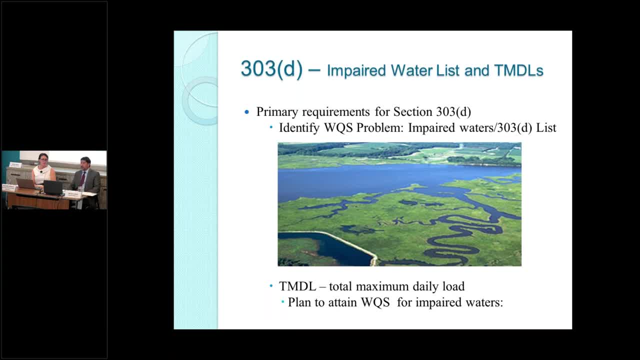 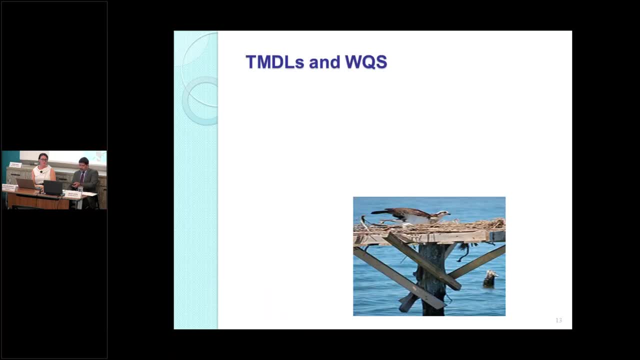 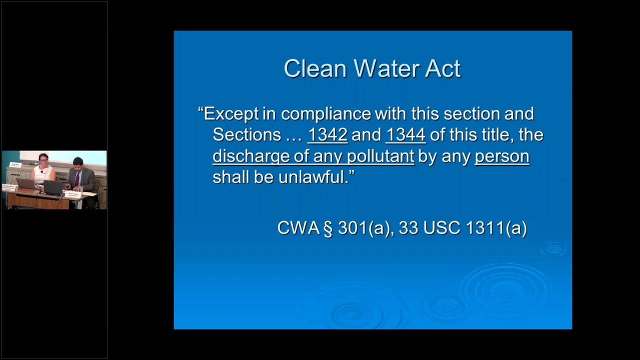 a lot of enforcement in that area, both civil and criminal, uh, and we're really very uh, protected of the chesapeake bay. next one, all right, so how do we calculate this? let's see if we can go back to the cover that and wait a second. i apologize. 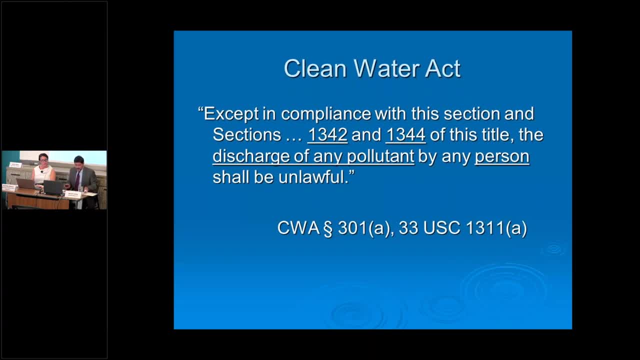 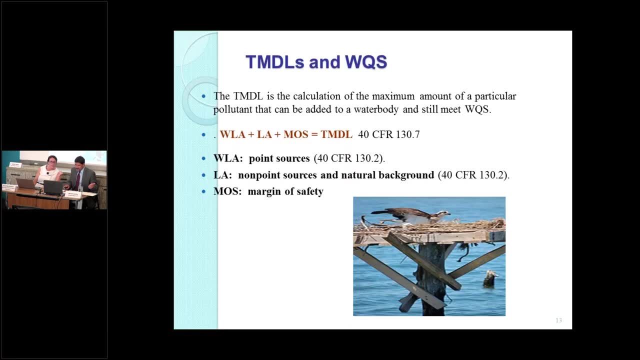 um, um, i don't have my cleaning glasses. that's why i'm: oh, did i went far, or okay? so it's a calculation of certain particular criteria. so tmdl, the total maximum daily loads, are calculated by you know mathematical formula, which um is uh. discharges from point sources discharges. 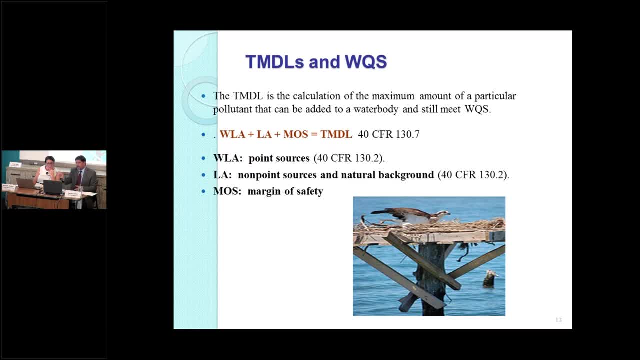 we add and then we have what we call a margin of safety. so this is a very technical, scientific way of determining that we, while we can decide what are they known, the point sources and non-point sources discharge that are coming to this particular water body. we also need to address 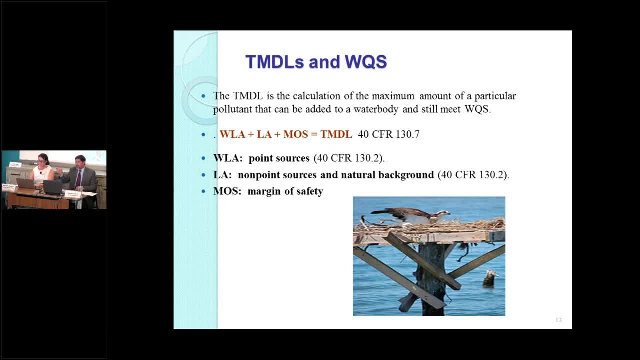 a potential sort of uncertainty that is addressed in the. you know the way that discharges go, the way that the water body, the way that the hydrology works, uh in all many other scientific uh elements that go into determining what is this maximum amount of a particular pollutant that can be added to a water body? and we still are meeting again. 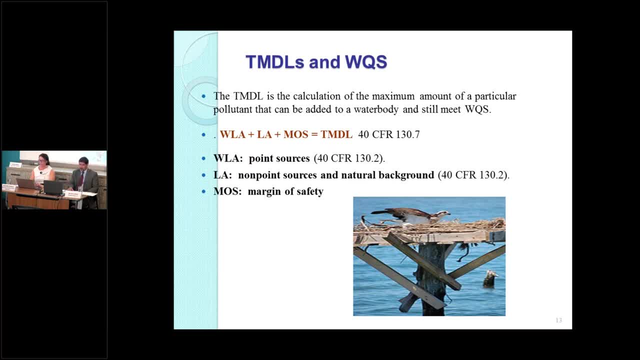 the water quality standards, remember that right. and those are addressed in the 40 cfr. for those of you who are like want to go to sleep, uh, started reading all these 130.7 and it's this long. regulations are extremely complicated. they're actually not as complicated. 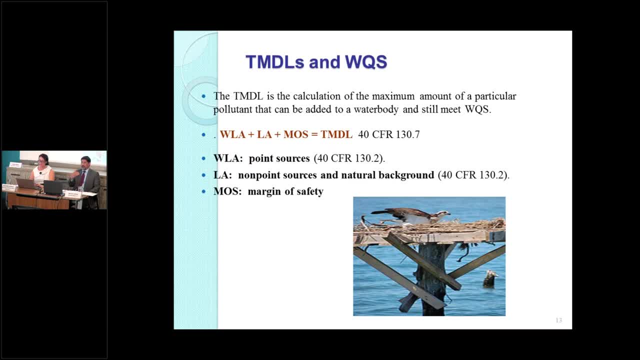 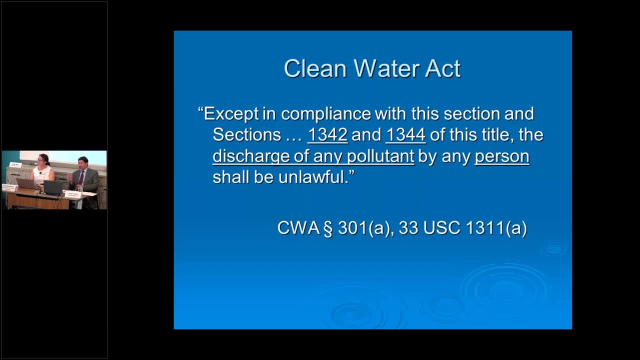 as one more thing, but they are narrative description of what i just told you. it's not easy if you're not a scientist to go address those. these are some of the complications that we have when we're enforcing these provisions. all right, um, this is one of the other neat things that we have. 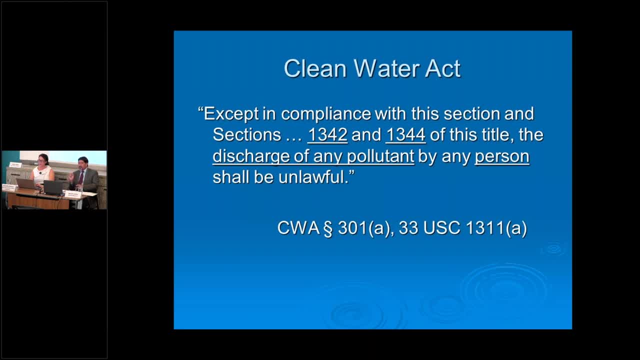 and this is why this statue is so powerful as well. uh, one of the first prohibition is that it reads: except in compliance with this section and section 1342 and 1344, which are the uh point source and the permits that are required under the court of engineers for dredge material, if 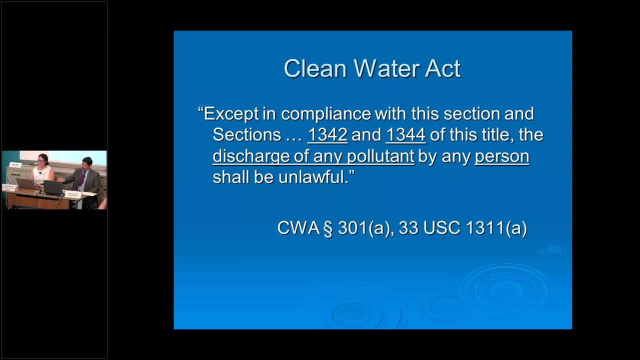 you're dredging, you're filling out a wetland, uh, you would need to have a permit. if you are discharging, uh, from a point source, you will need a permit. but the important thing here is that the discharge of any pollutant by any person is unlawful unless you have a permit right, and that is. 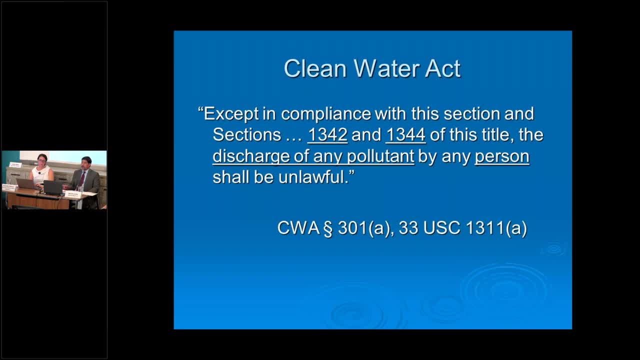 extremely powerful. that is extremely helpful when you're doing enforcement, because nobody can say, oh, i didn't know that i didn't need a permit. you actually need a permit for everything that you do right pretty much, so it's a great provision. uh, it's there for you to review, um. 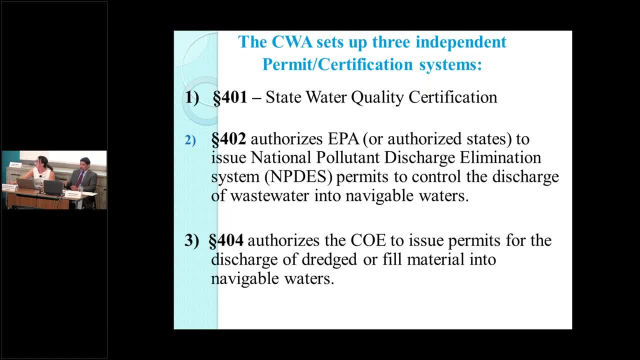 these are going to go quickly because i think amanda's going to cover this, but they are three independent permit or certifications that are required. the first one is section 401 talks about the state water quality certification. these are uh issues that are addressed at the state level. when you are trying to address 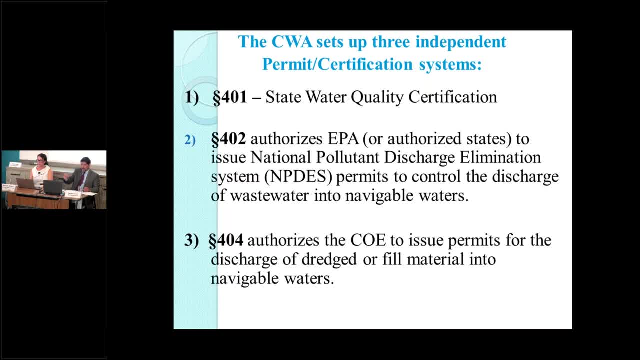 discharging into a water body, but only on this at the state level. section 402 authorizes epa to issue what we call the national pollutant discharge elimination system permits, and those are the ones controlling the discharge of wastewater into navigable waters. so these are the typical uh potws: the wastewater, wastewater treatment plants discharging after they. 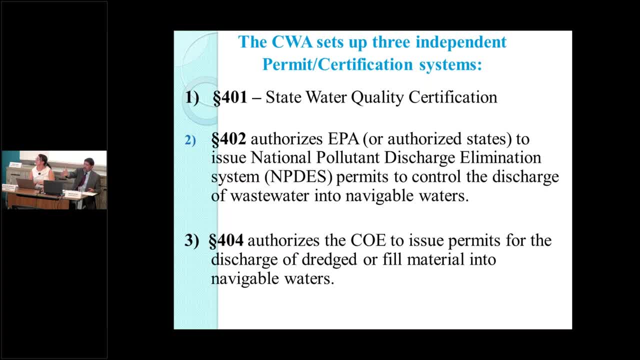 they collect the sewage, they treat it and then discharge into a water of the united states. uh, they need a permit in order to do that, and we call that an mpds permit, section 404, while epa has jurisdiction as well as well, it's really a court of engineer issue. 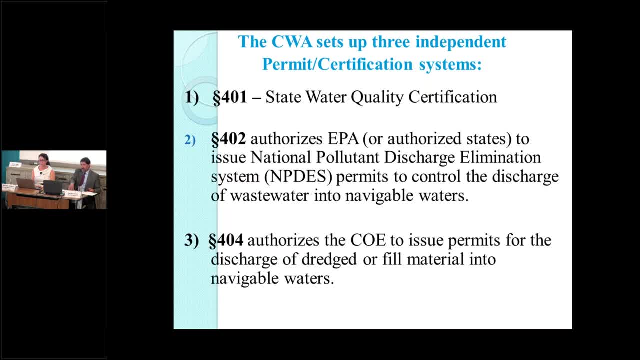 and in that the court of engineers are one response- the agency responsible for issuing permits regarding the discharge of dredge material or fill material into wetlands. uh, there's been a lot of great cases associated with the discharge of fill uh material in the wetlands. uh, in fact, one of the rapano's case is one of those where 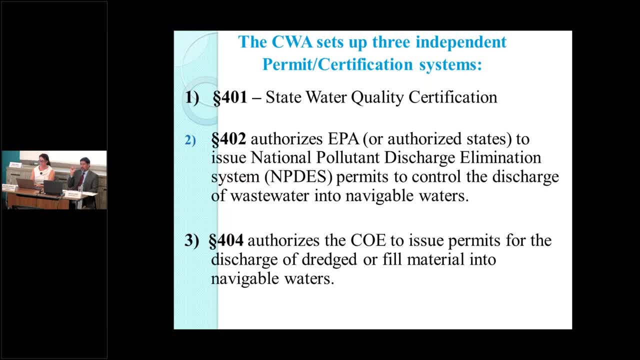 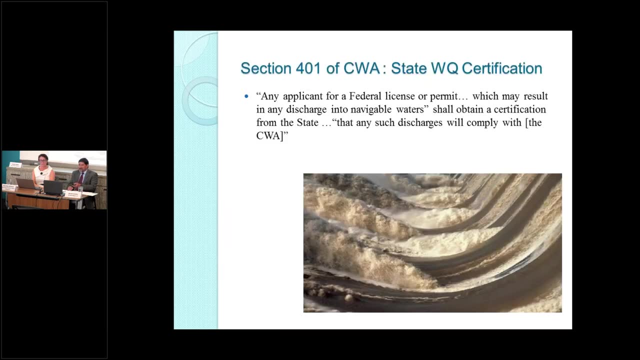 the individuals, i think, put sand into this area. it was litigated for more than 20 years by another, resolved to the agreement or disagreement of the agency. um, i know, leave it at that and somebody else will talk about it. all right? um, so, any applicant- this is the first one- 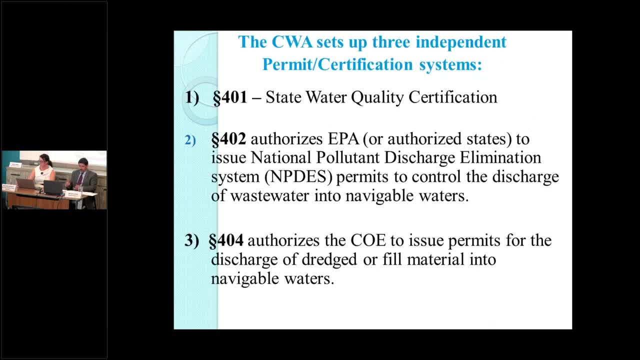 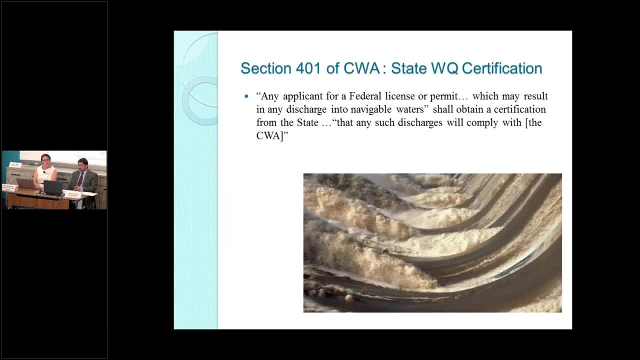 so the out of the three, if we go back 401, 402 and 404, you'll find it here. all right soul are the main provisions that we're talking about. so section 401 is a state water quality certification. if you are an applicant for a license or permit, that may result in a discharge. 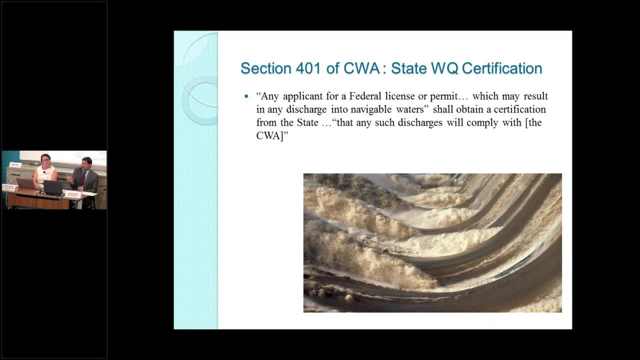 into navigable waters, you need to obtain a certificate, basically from the state that allows you to do it. so it's sort of like a way of indirectly dealing with projects that may not are causing direct discharges but as they develop, you can, they may have an impact in terms of 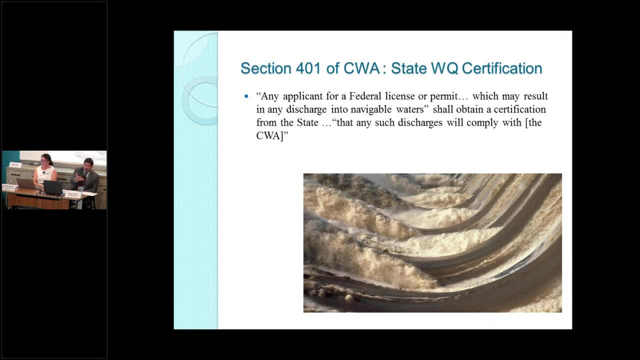 discharges, but it's not necessarily a wastewater treatment plan which is obviously going to discharge into water. the united states, it may be a project related to anything that you can, mining perhaps, uh or other major projects. right, any experience with that? or the 401? yeah, i've got. 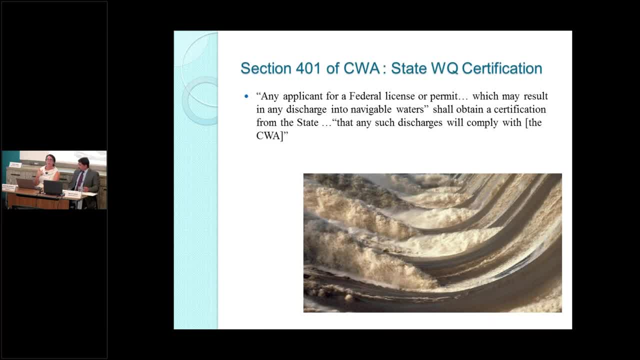 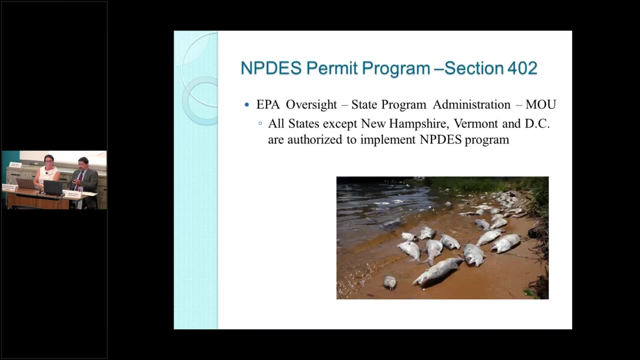 that a little bit about that, my presentation. um, so this would come up in states that do not have delegated authority. where the epa is issuing the npds permit, there would have to be a corresponding state for one water quality certification. that's right, thank you. um so um, the mpds permit program is. 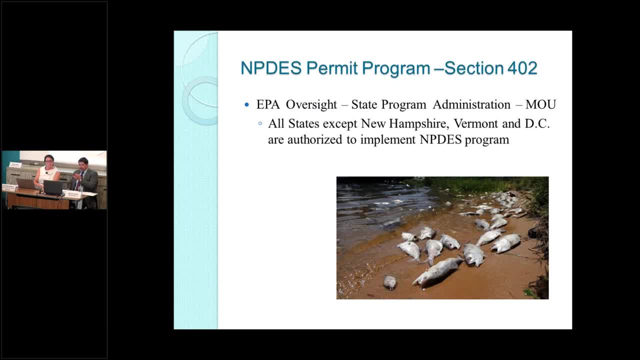 for the one i explained. i think all the states. i think this is still true- that all the states that said new hampshire, vermont and dc are authorized to implement the mpds program. so it's really a state agency who is providing the permit to the particular discharger. 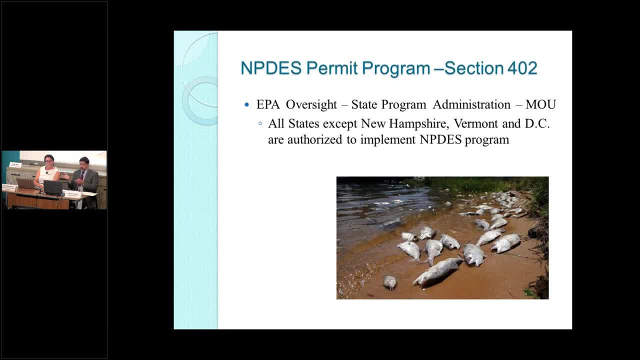 and this could go into different categories of discharges from the agenda: wastewater treatment plants. it could be industrial users that are discharging into a sewage. it may be required to have pre-treatment, um, a pre-treatment of the waste before it goes into a pwd. all those are addressed through here, um, and i think um, and those are. 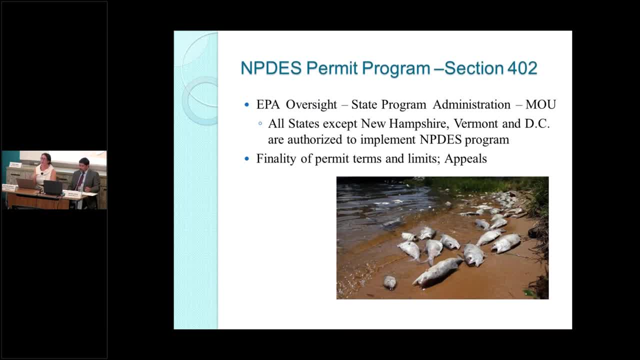 okay, it makes sense for me to throw it in here rather than bring it up um later, but so right now it's um. it's new hampshire, massachusetts, new mexico and idaho that don't have the permit to do that. they have delegated authority. other states don't have full delegation, so they'll have authority. 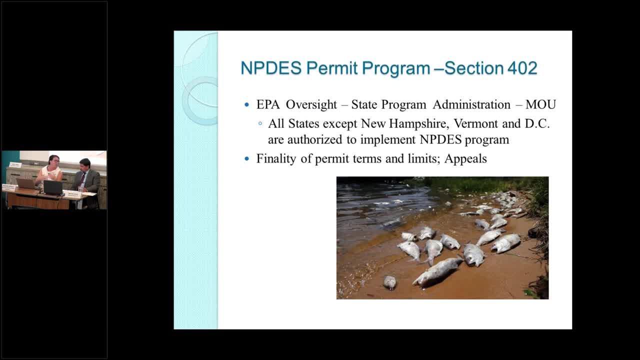 to administer the mpds program, but perhaps not biosolids or pretreatment idaho. just on june 5th their program was approved by epa, so as of july 1 of this year they will start issuing uh municipal uh mpds permits and then they're on a schedule to uh to issue other things like. 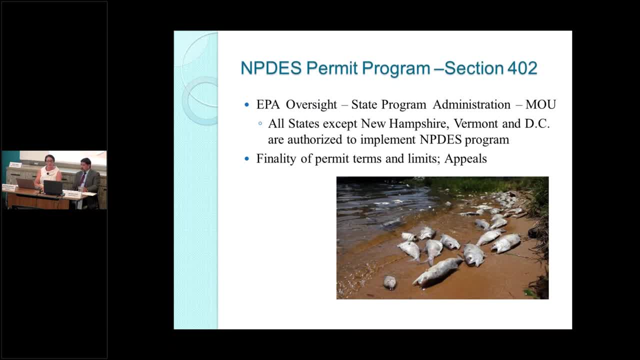 on a yearly basis start to ramp up and what they, what they actually administer. massachusetts is in the beginning stages of looking at delegation. they have to have legislation, so they've been working on that. uh, so no application has been filed in massachusetts. okay, and you can go into the. sorry, there's important distinctions between what the mpds. 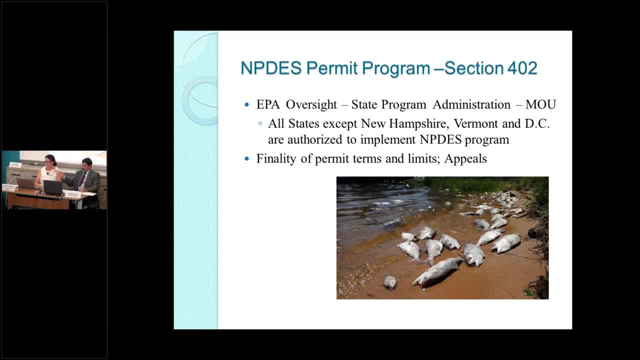 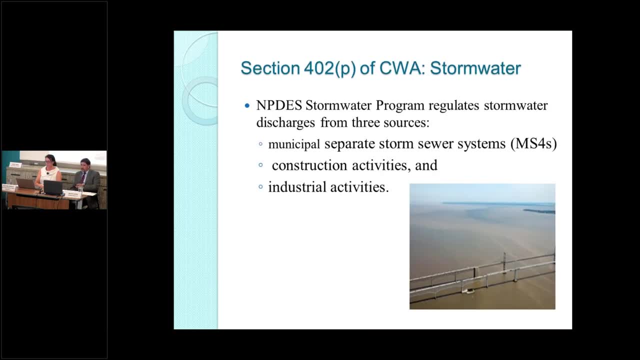 program is the pre-treatment program, uh, in other discharging uh, and we'll address those, i think, later. or we can address some questions right, um, so the mpds program- actually it's right here now like, um, it's a storm water program, so it's um discharges from three different things: municipal. 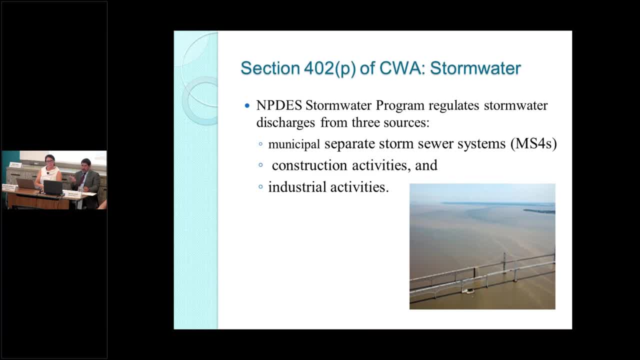 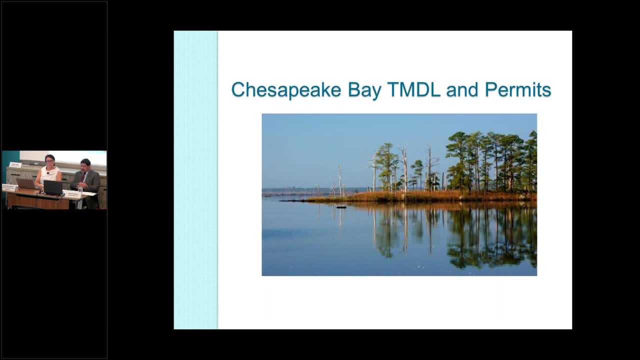 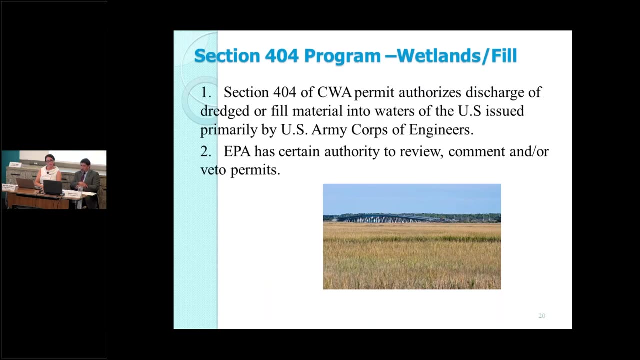 separate storm sewer systems and construction activities and industrial activities. right um, and i think somebody else is talking about the chesapeake bay total maximum daily loads and the permits. i'll leave it at that, um, and then again, section 404 program is regarding wetlands and the field wetlands, which we already covered. 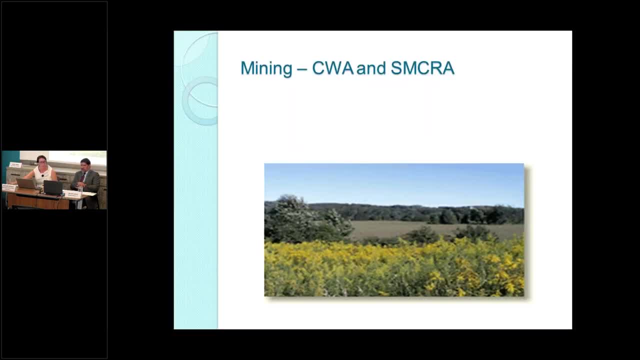 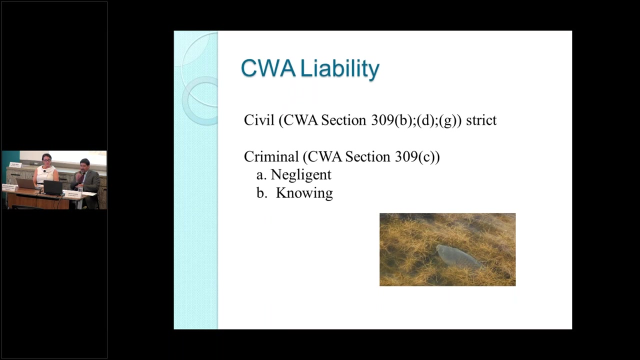 um, all right, mining. um, there is a good connection between the clean water act and what we call one minute, okay, um, uh, this, uh surface mining, uh control act, i think it is. um, and since i only have one minute, we'll talk about it, uh, perhaps in the questions i want to address. 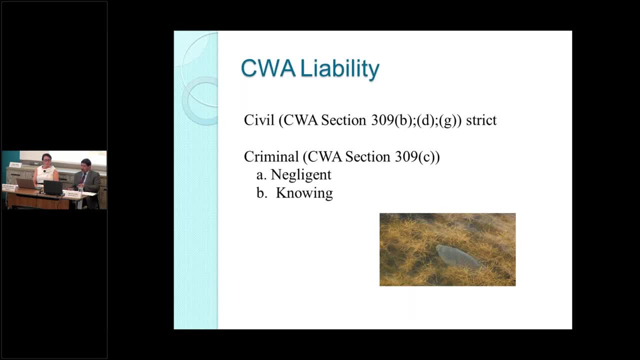 the enforcement of the clean water act has um a good connection between the clean water act and the civil liability, which is basically strict liability and has strict or criminal liability for negligent discharges and knowing discharges- and negligent discharges would be a misdemeanor- and knowing discharges, which are 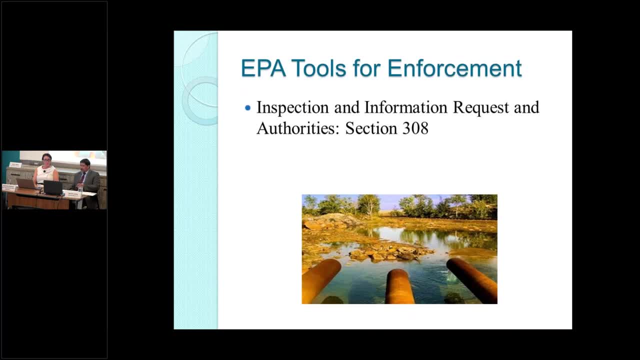 intentional would be a criminal violation, and they're great tools for enforcement. uh, it's my bread and butter every day. of most of my cases i couldn't water my case, i would say the current majority. um, and other tools of enforcement, of course, include inspection. uh, we can send information requests to uh, for example, wastewater treatment plants that may not. 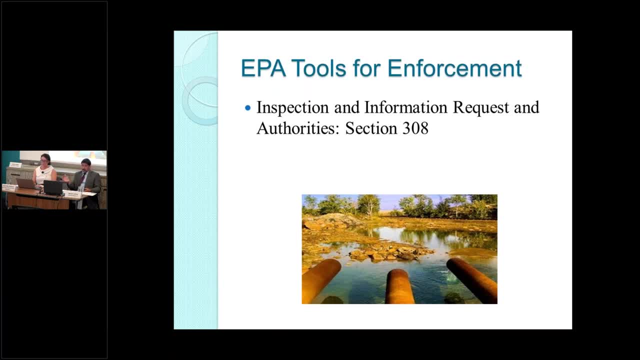 be complying with their particular permits are having difficulties with uh doing certain things. we have certain instances where they have bypasses and while they can do that in certain circumstances they may not notify the agency. that's a problem, uh. so we have a way of doing that. we also have 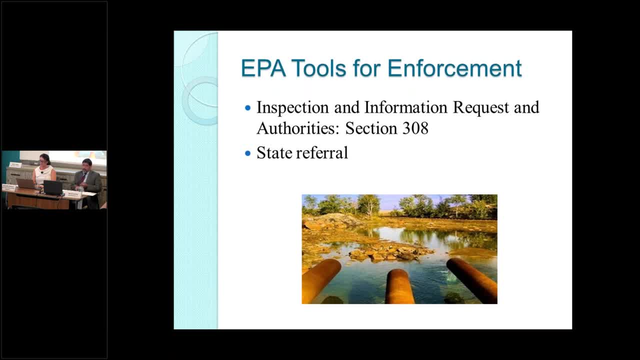 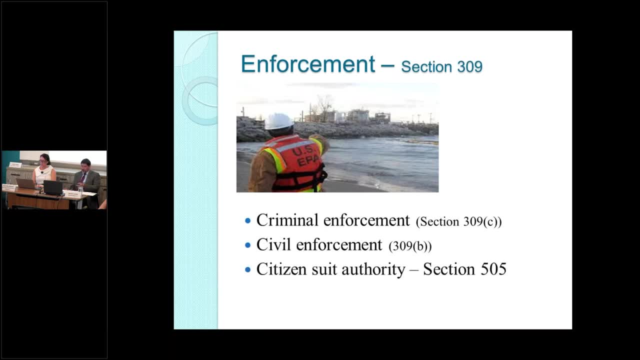 the ability to refer our cases to the state for state enforcement, as opposed to federal uh, and then we also review those permits by the state as well. so that's the way to go, for example. for example, if we want to do a design for a city, um, so if we're a city, no matter what, we're going to go through this process. 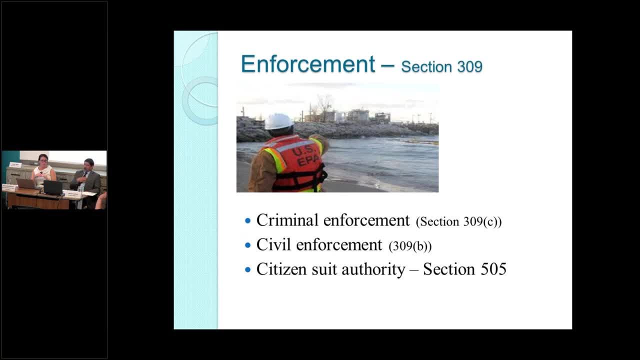 the city can provide us with some legal action to help us make sure that we can do some of those things, uh, or that that we can support our agency to do the things that we like, uh, and then we'll probably have the ability to go and do a little bit more. 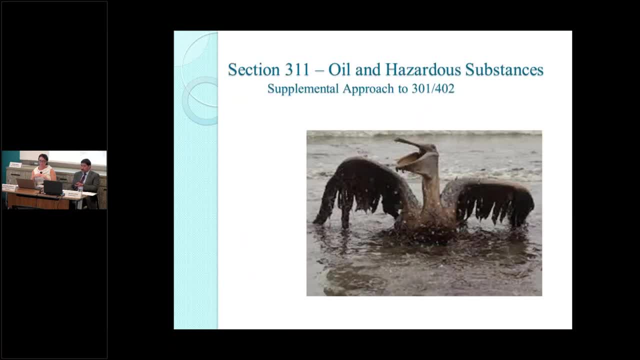 and now i'm going to just talk a little bit about the current legal procedure for law enforcement. so what i want to share with you, uh, when you apply for legal action, is not what will bring you a criminal charge. the legal action is what you need to Chairman. 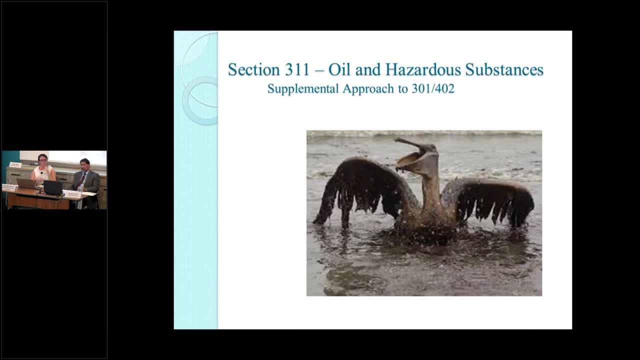 If you're discharging oil- and this is a result of the Exxon Valdez- there's specific provisions of enforcement regarding the discharges of oil into waters of the United States, And that's a separate provision from the Section 4302, which would be the one, the regular one. 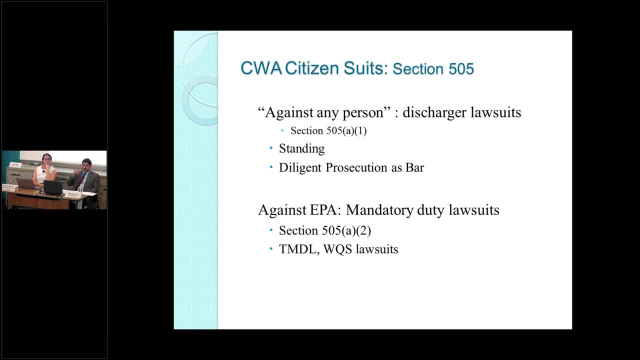 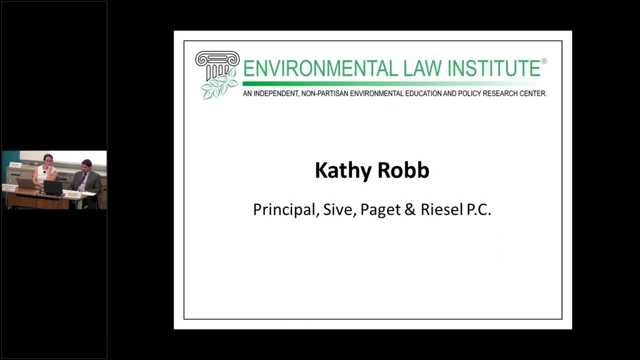 All right, And with that, I think I'll leave it with. yeah, Kathy, is that you? That is I. Hi everyone, This is Kathy Robb. I'm a partner at Saad Pajan and Rizal in New York City, practicing environmental law. 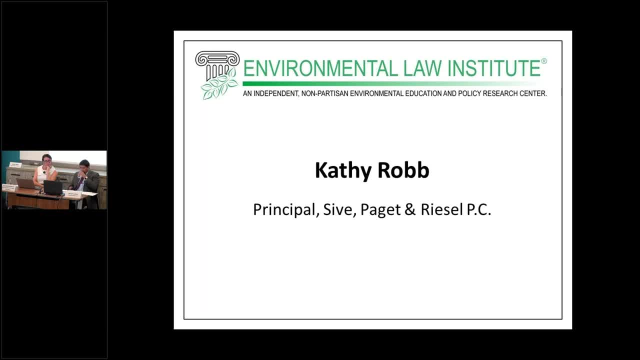 And I want to thank ELI for asking me here today and joining on this terrific panel, and to all of you for joining us. As David said, the Clean Water Act has been a successful and powerful statute. Today, I'm going to be talking about what navigable waters, or waterways, 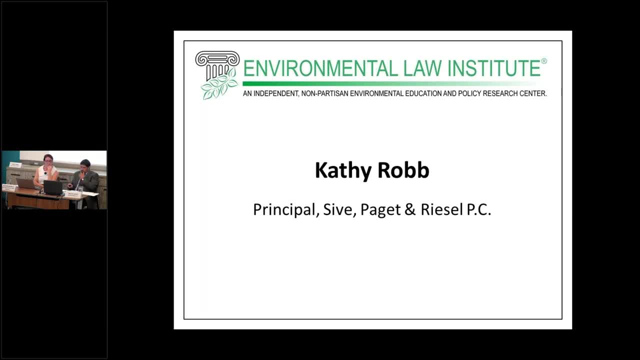 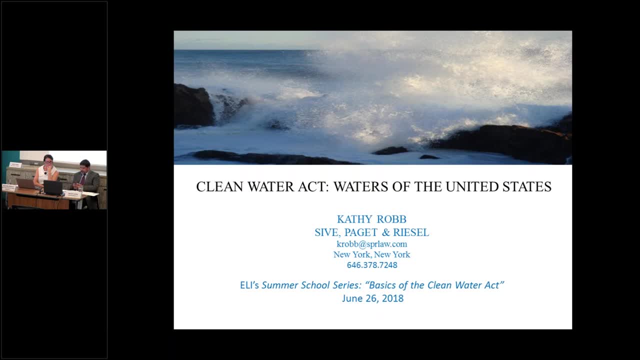 Waters of the United States, the jurisdictional waters regulated under the Clean Water Act, may mean, And you all will see my slides and hear me, but you are not going to be seeing me, So don't worry that your screen is not working properly. 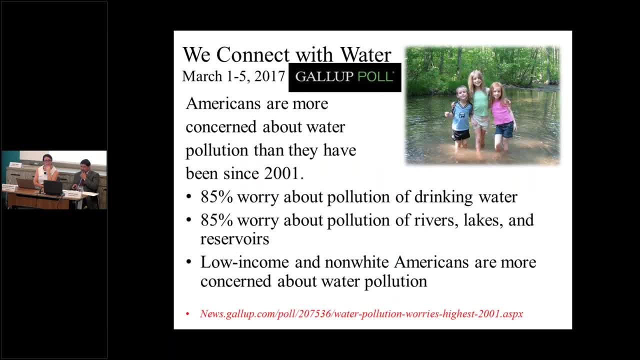 Next slide, please. Water is more on everyone's minds than ever, no doubt in part of as a result of the water quality Issues in drinking water which have been highly publicized and reported from Flint, Michigan and other cities over the past three or four years, which involved lead and Americans. 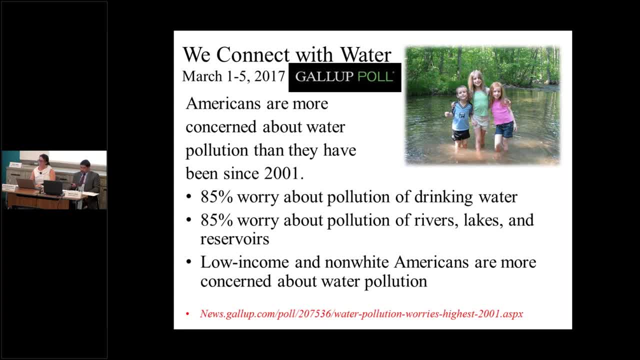 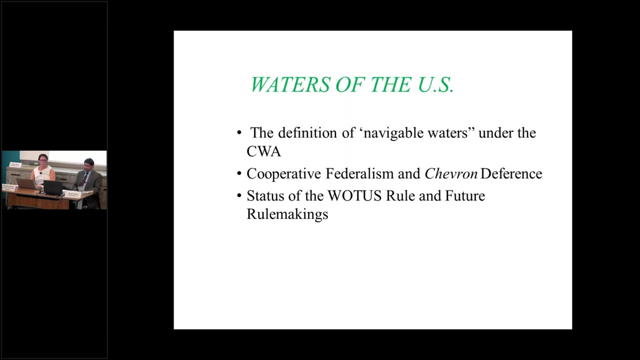 The Gallup does a poll every year about Americans views about various environmental issues, and Americans are expressing that they're more concerned about water pollution than they've been since 2001.. So this is an important area. Next slide, please. The Clean Water Act is 45 years old and counting and we're still grappling with its jurisdiction and what cooperative federalism means under the act. 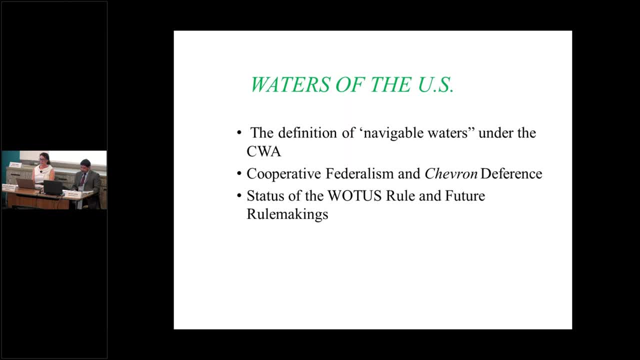 Today I'm going to focus on the definition of navigable waters or waters of the United States, which we also often refer to as WOTUS. It's the cornerstone Of the Clean Water Act. I'm also going to briefly discuss cooperative federalism and Chevron deference, and the status of the 2015 WOTUS rule and subsequent developments that are ongoing about the jurisdictional definitions. 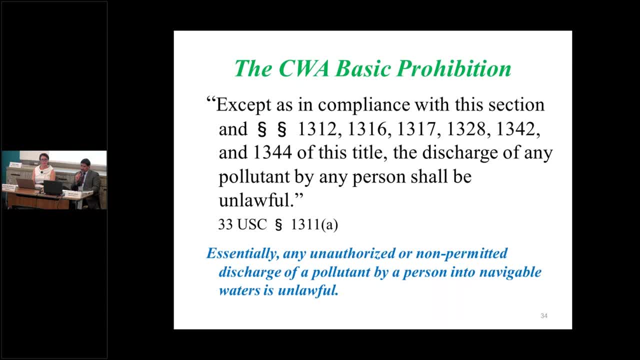 David showed you the basic prohibition for the Clean Water Act. EPA and the Army Corps of Engineers administer the Clean Water Act And discharge into navigable waters is prohibited unless it is permitted, as David mentioned, and each of those terms is a term of art that has been defined in the statute, the regs and also case law. 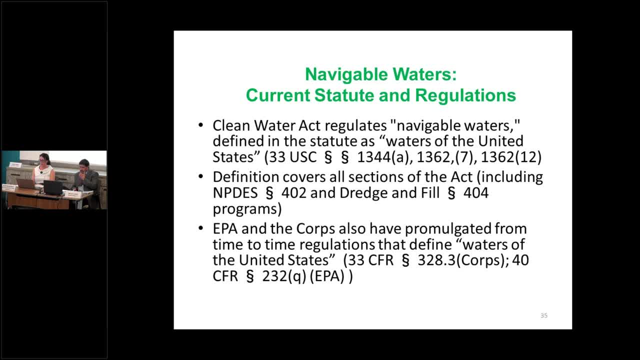 Next slide, please. Under the statute. in the statute itself, Navigable waters is defined as water, And the definition of water is the water that is in the waters of the United States, and we're going to use the terms interchangeably for our purposes here today. 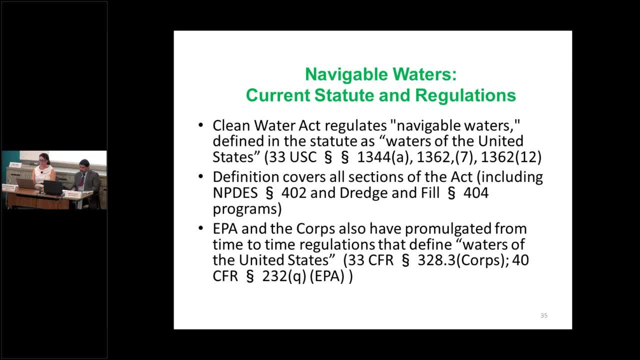 The definition covers all sections of the Clean Water Act. Regulations also have been promulgated for most of the sections of the Clean Water Act. There's an outline in your written materials about waters of the United States under the Clean Water Act from the beginning. 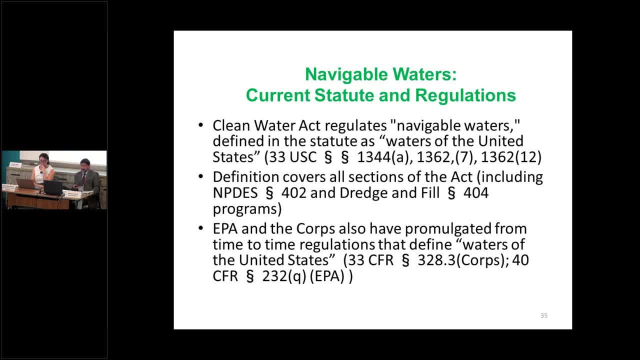 To the 2015 WOTUS rule. If you want to take a deeper dive and look at citations and definitions and deeper descriptions of the rules and regulations as they've evolved over the years, then we can do today in our program, Next slide, please. 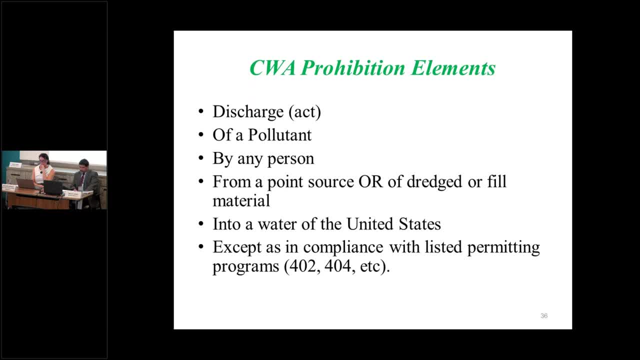 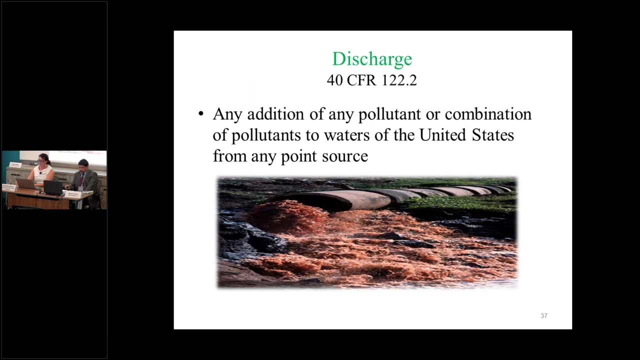 So these are the prohibition elements of a Clean Water Act violation. You cannot have navigable Waters Discharges Except as in compliance With the particular permitting program that applies to your activity. Next slide, please. All these terms are going to be discussed further by Amanda when she talks about the permitting program. next, 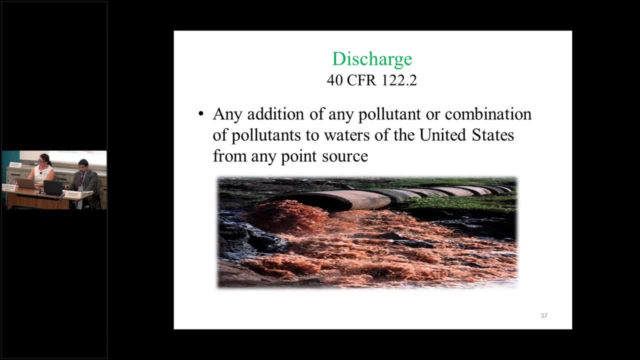 But for the context of our discussion, It's very easy to see here That the muddy red water coming out of a pipe is going into a waterway, And this is a photo of a discharge from a classic point source Into jurisdictional waters. 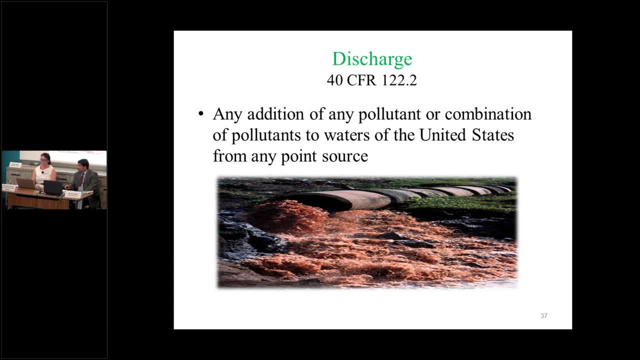 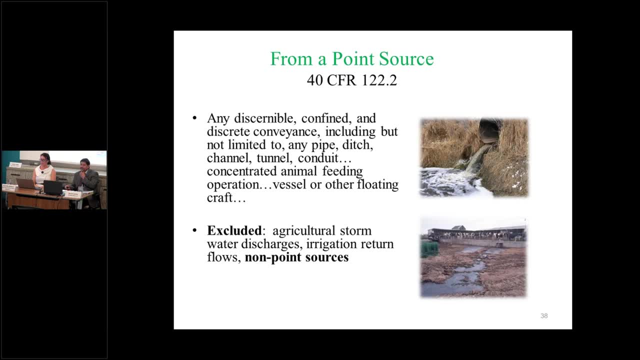 And is regulated under the Clean Water Act. Next slide, please. Non point source Is run off that has no discreet confined conveyance and more diffuse flows, And these are photos of that, and excluded On the left and right Are The items listed on the slide. 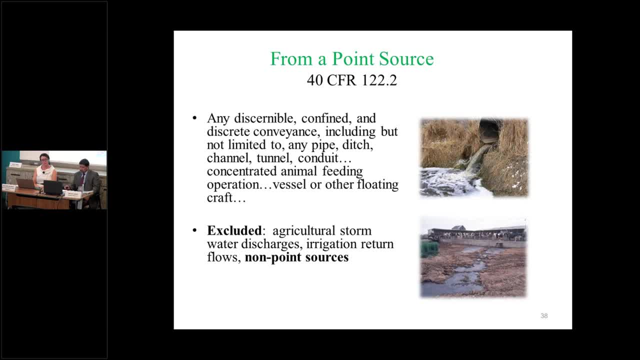 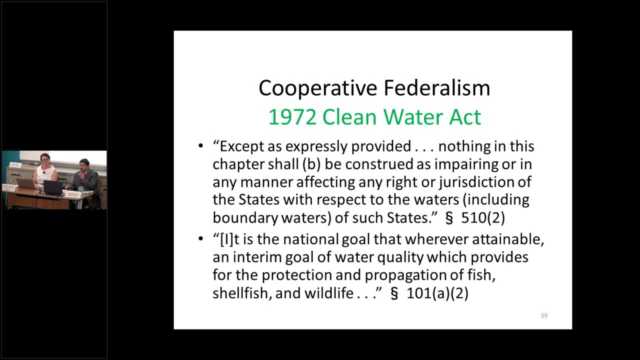 This is through the regulations. Next slide, please. The modern Clean Water Act Statue Began in 1972. And Clean Water Act Authority at the federal level Is under the. as a result of the Commerce Clause, Most states Own. 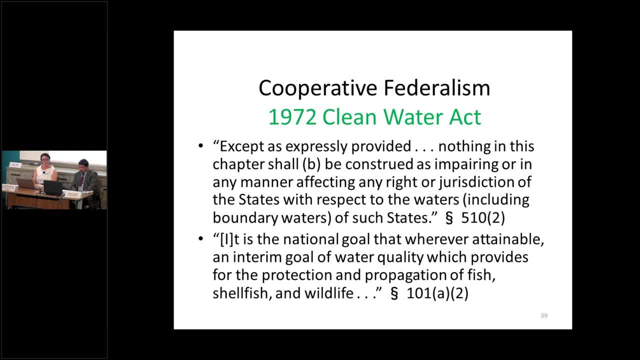 own water. The statute reiterated in 1972, and the language is there on your slide- that the federal regulation does not affect states' rights or jurisdiction over waters. This is known as cooperative federalism, which applies to the Clean Water Act as well as some of our other main. 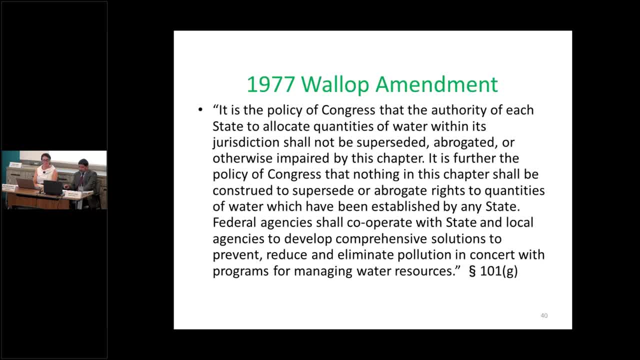 environmental statutes. Next slide, please. In 1977, the Clean Water Act was amended and cooperative federalism was reiterated, stating it's called the Wallop Amendment after the senator that put it into the statute state jurisdiction is not to be impaired, and 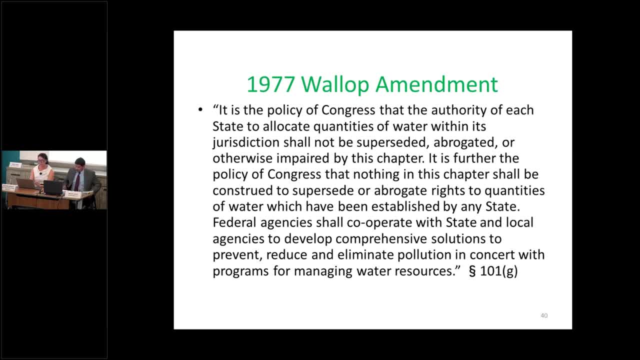 federal and state governments shall cooperate with each other on the Clean Water Act, And this colors everything that goes forward under the Clean Water Act. There's a lot of discussion, give and take between the federal level and the state level regarding water. Next slide, please. 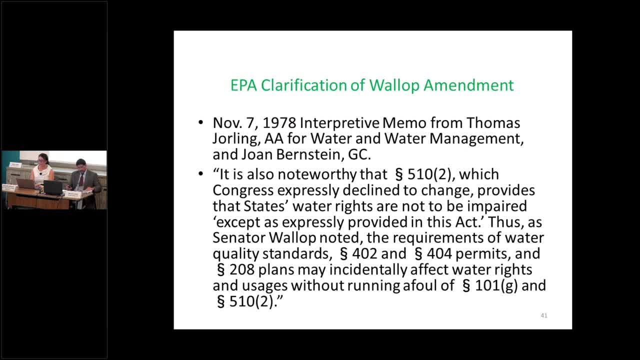 Just so you know, there was also a 1978 EPA legal memoranda that weighed in on cooperative federalism and stated that the statutory language meant that the state's rights are not impaired except as expressly stated in the statute. Next slide, please. So what is the struggle about? what navigable? 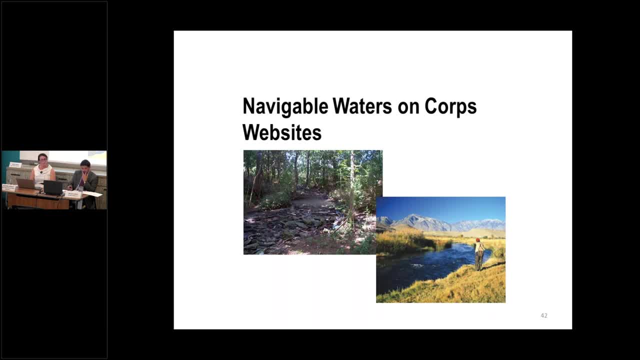 waters or waters of the United States means for jurisdiction under the Clean Water Act. Water is an area where one picture is often worth a thousand words, And here is a photo of traditional navigable waters. It's surface water, it flows and we could all agree by looking. 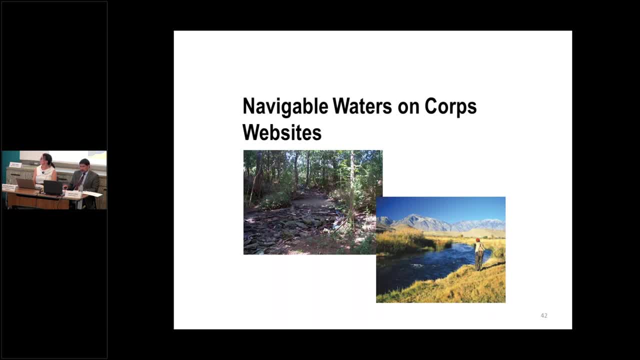 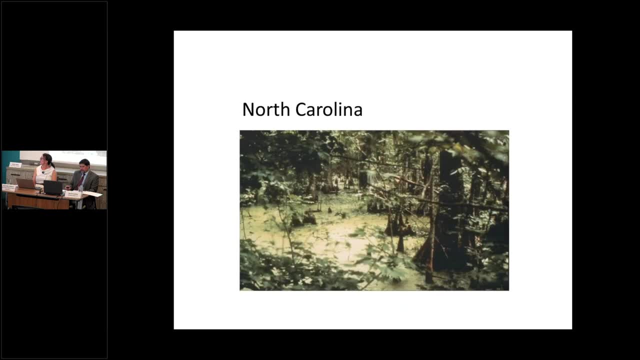 at the photos that you could float a boat on it. Next slide, And there are the boats. traditional navigable waters- Next slide, please. Over the years, many other areas have also been characterized as waters of the United States subject to Clean Water Act jurisdiction. They include wetlands, which is 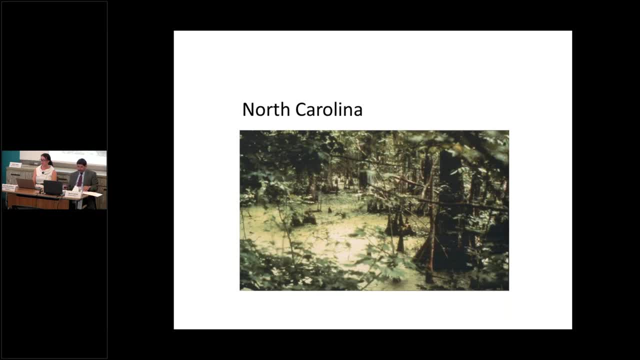 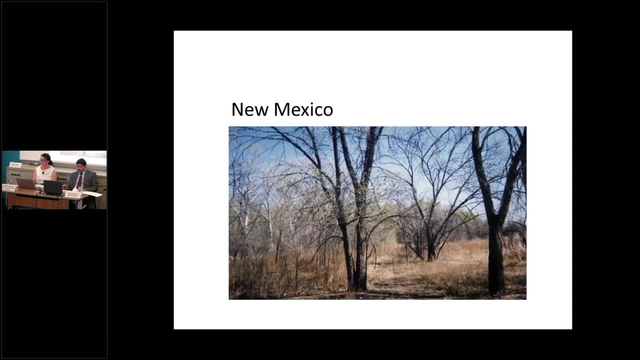 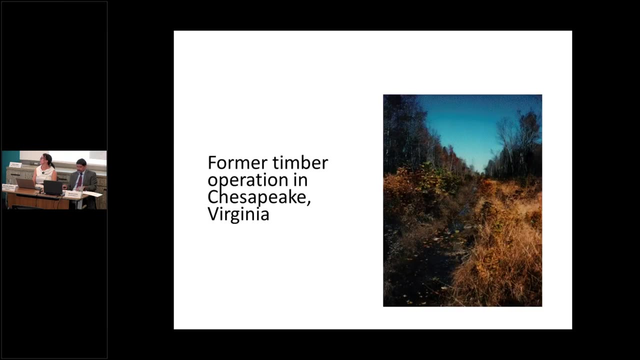 depicted in this North Carolina photo: Next slide. Old logging areas that have water seasonally Next slide, Places where water collects seasonally Next slide, And places where water perhaps once collected Next slide And filled in collection areas. This is a filled in collection area Next slide And filled in collection. 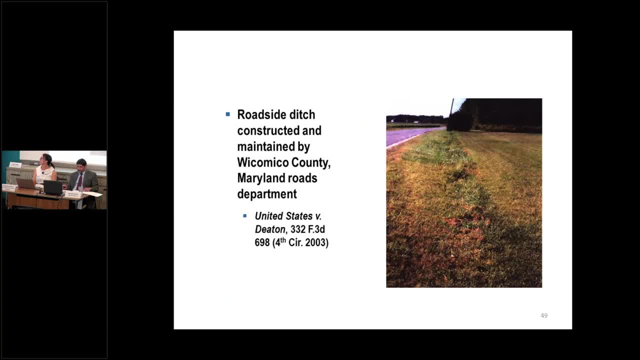 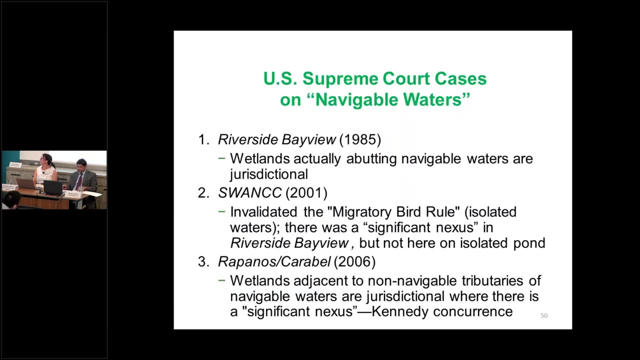 areas- This is a farm ditch, Next slide. And ditches such as this roadside ditch which was constructed and maintained in Maryland, The Deaton Ditch- Next slide. So all of these designations of jurisdiction of waters of the United States have come about as 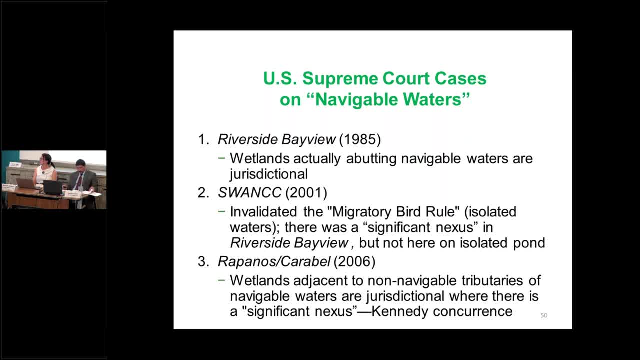 a result of case by case determinations by the Corps. there's a hardship on the Brixton river. This is the state at the time of this bill and the state has the right and the right to decide on whether permits are needed for activities in particular areas. 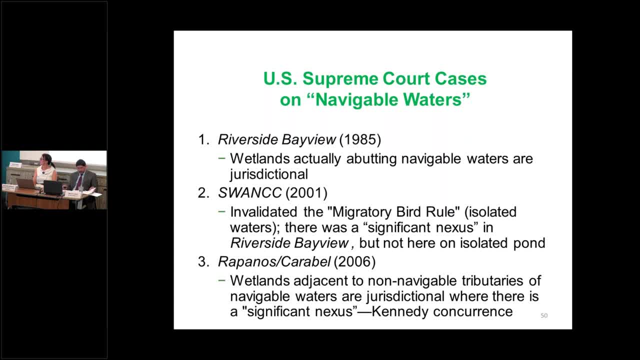 The Supreme Court, as David mentioned, has considered what navigable waters means In three key cases. They're called Riverside Bay, view swank and replica Bell And again, if you need a complete citation and description, go to the outline that's posted online. 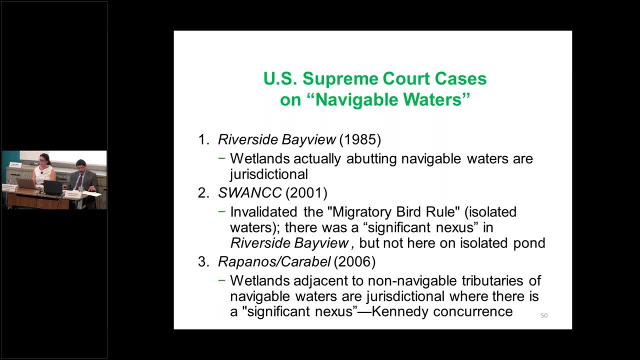 in Riverside Bay, view swank and Rapunzel's Karabelle. and again, if you need a complete citation and description, go to the outline that's posted online. In Riverside Bay, which is in 1985, the Supreme Court considered whether wetlands actually abutting a navigable. 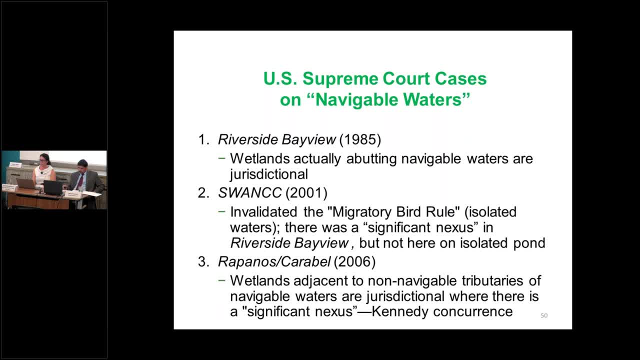 water are jurisdictional under the Clean Water Act. And they said, yes, there's a significant nexus between the navigable water and the wetlands abutting and that that is within the regulatory purview of the Clean Water Act. Then, in 2001,, in a case called Swank, 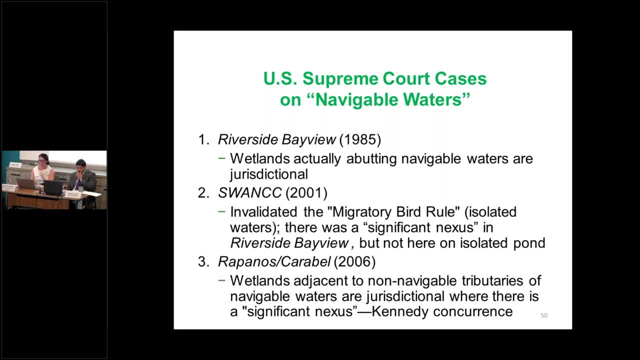 there was an isolated pond that the Army Corps was regulating as a result of migratory birds having stopped there from time to time, And this was referred to. the regulation that was the subject of the case was referred to as the migratory bird rule, And the Supreme Court said: 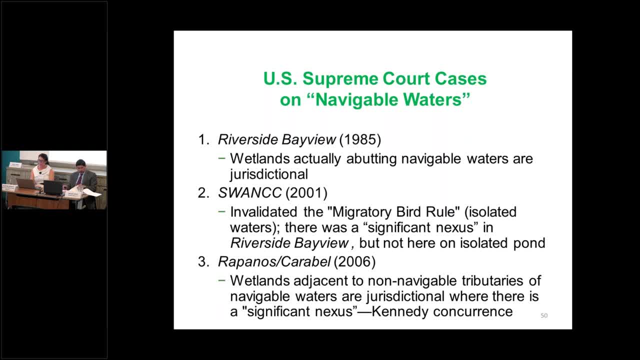 migratory birds on an isolated pond don't establish jurisdiction of the Clean Water Act And there was not a significant nexus between the isolated pond and navigable waters- waters of the United States- and invalidated the rule Then in 2006,. two cases that involved wetlands adjacent to non-navigable tributaries. 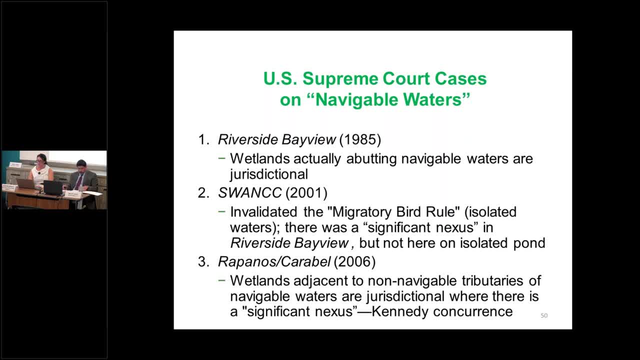 of navigable waters were combined in the Supreme Court. This is called Rapanos-Carabel And the court said that it's jurisdictional. these wetlands that are adjacent. These are the waters that are not deemed to be navigable or they are not considered navigable. 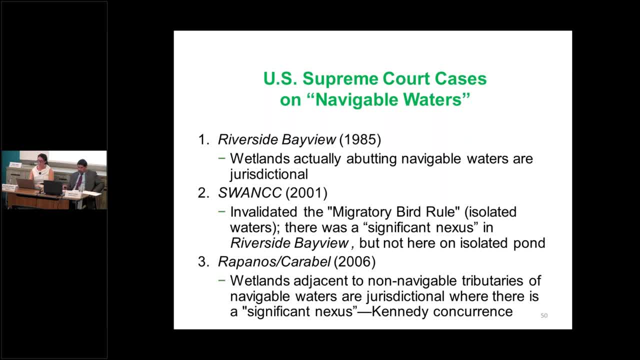 And that one had a different name And that was adopted by the Supreme Court, or Justice Scalia. And then the third case was in 2001, where we heard a Supreme Court's decision to removed the water from the wetlands adjacent to non-navigable tributaries. 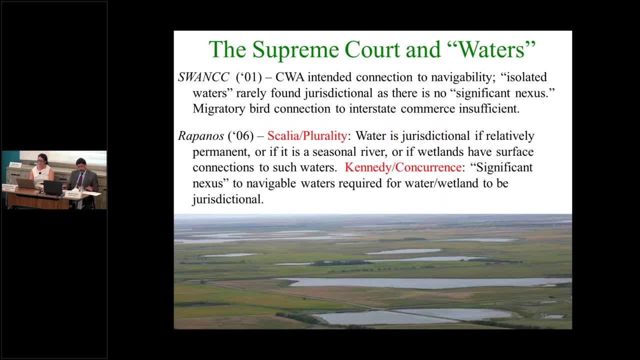 where there is a significant nexus, And then that is the discussion that we're still under today about what that actually means. Next slide, please. So Rapanos was a 4-1-4 decision by the court, with Justice Scalia writing for the plurality of four. saying that WOTUS Waters of the United States could include the water that has been separated from the WOTUS and the waters that have been retained by the ships of the United States could include the water, as the Supreme Court said, within the development of a new water system. 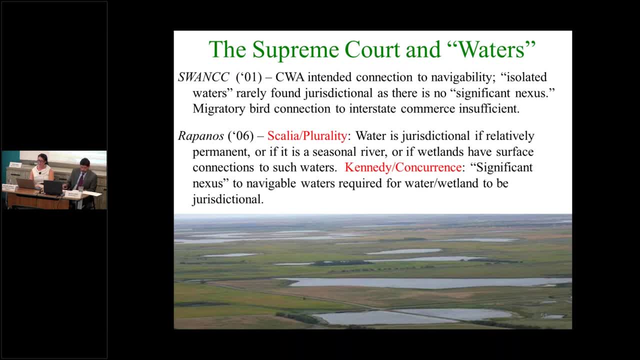 include relevant relatively permanent waters, but not intermittent or ephemeral waters, and also wetlands with a continuous connection to permanent waters. Justice Kennedy in a separate opinion, which was a concurrence, said that adjacent wetlands could be protected if they had a significant 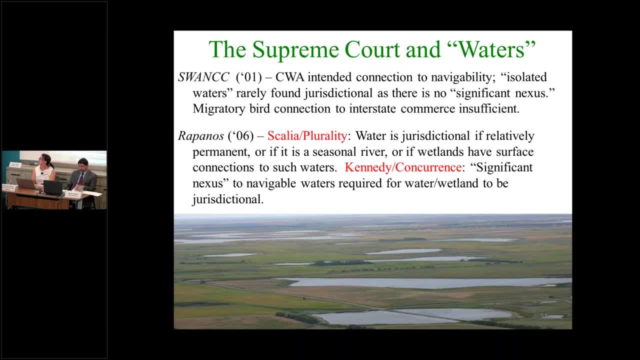 nexus hydraulically to non-navigable tributaries of navigable waters. So when you have a 4-1-4 split in the Supreme Court- which we did in this critical case that involves waters of the United States, there's a doctrine called the 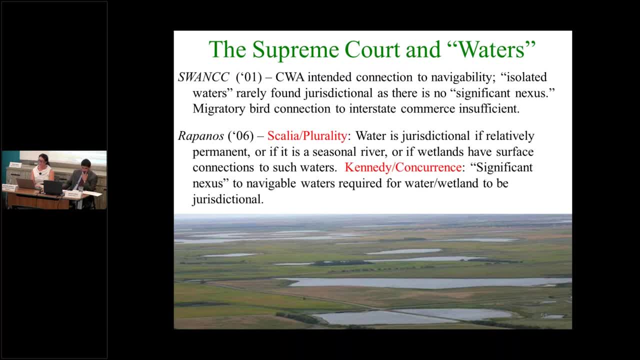 Marx Doctrine which applies to these split decisions that came out of a 1977 Supreme Court decision, And what it says is: if no single rationale is supported by five justices in a majority opinion- which we didn't have in Rapanos- the holding of the court is viewed as the position taken by the concurring justices on the narrowest grounds. that pulls the plurality and the concurrence together. 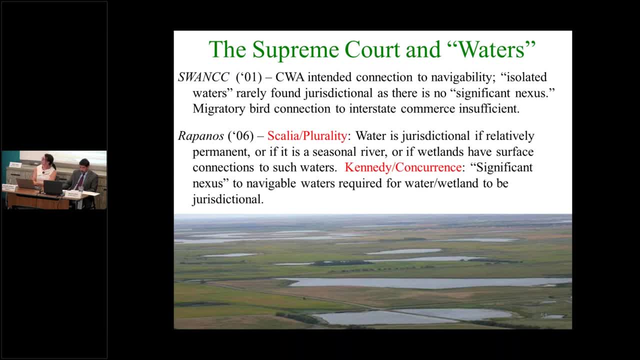 And that opinion is called the controlling opinion, And then throwing up of hands about where we were going with the jurisdictional waters And this becomes key. this distinction between Justice Scalia and Justice Kennedy becomes key when we look at the 2015 WOTUS rule, which we're going to in a minute. 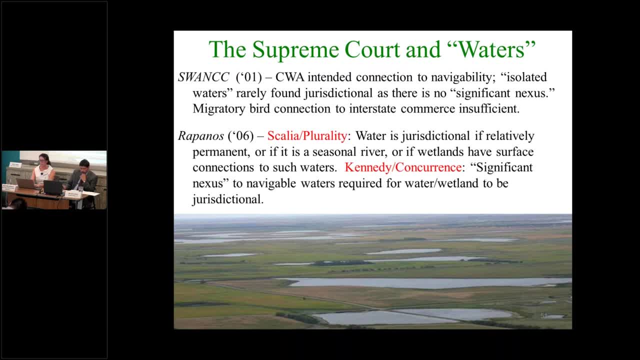 And it applies to it's applying Rapanos to change Challenges to the WOTUS rule and the subsequent articulations of what waters of the United States may mean for us under the Clean Water Act. But fast forwarding to 2015,. the WOTUS rule was based on Justice Kennedy's significant nexus articulation and it references that almost 500 times. 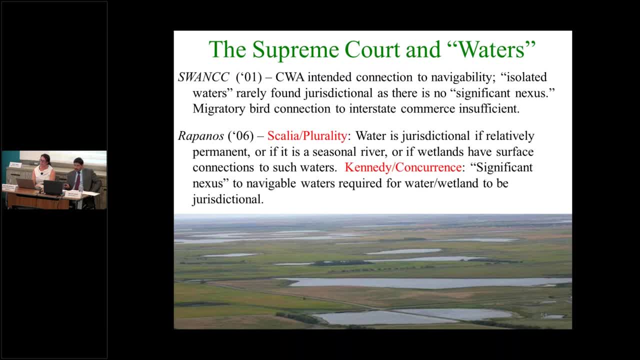 About two weeks ago, The court issued a decision in a criminal case that's unrelated to environmental law, but the parties had briefed as a result of the case whether this Marx doctrine should still apply. A lot of people are critical of it. The Supreme Court did not decide whether Marx is good, bad or indifferent. 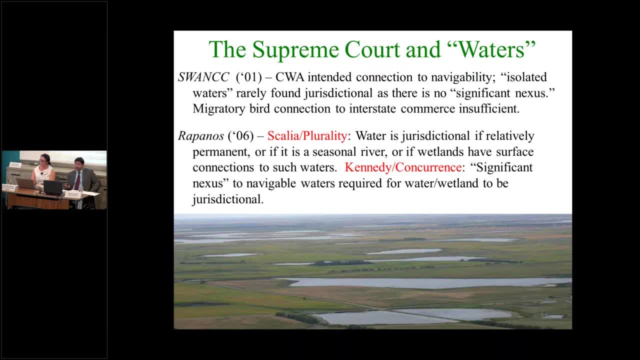 They sidestepped the debate and decided the criminal case on narrow Or grounds, but they did reverse the 11th circuit, which had relied on marks in applying its decision, and many things that many think that the marks doctrine should be abandoned, but doubt that the Supreme Court will do it. 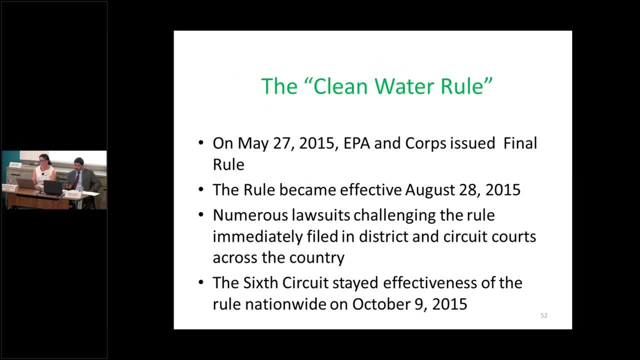 Next slide, please. So since Rapanos, many case by case, jurisdictional determinations have been made by the Army Corps, often conflicting Depending on which core district you're in, and guidance and draft rules were considered between 2006 and 2015,, and those are all described in detail in the outline. 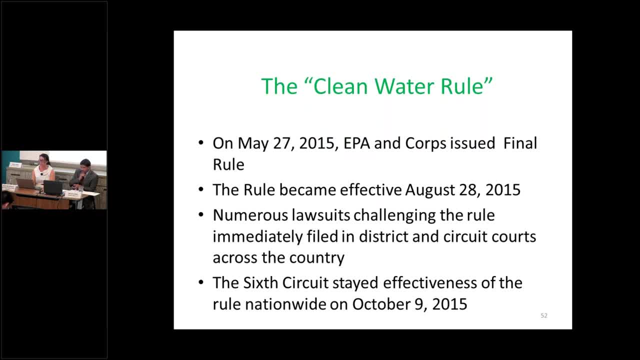 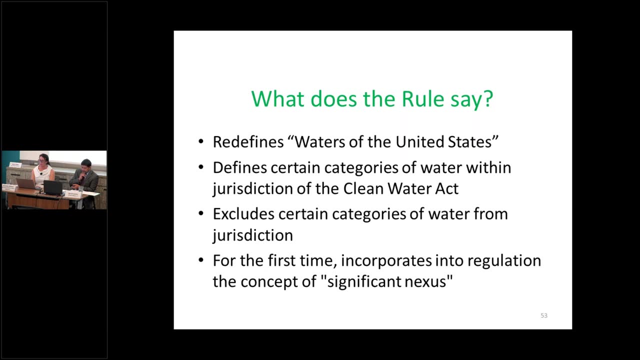 We're going to jump to the 2015 WOTUS rule, And that is also described in detail in the posted outline. Next slide, please. So The rule was intended to clarify what Waters of the US really means and whenever there. 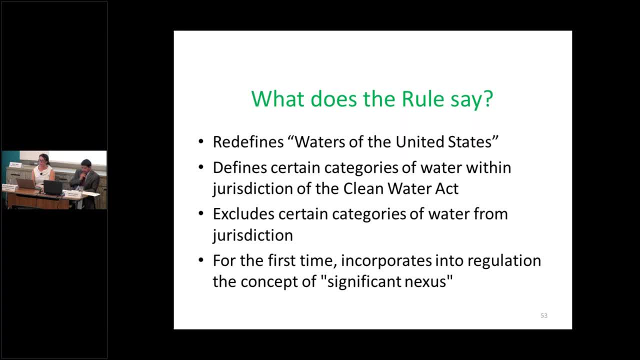 is an interpretation of a statute required. the concept of Chevron deference is likely to come up and it's worth it to take a tiny detour to just talk about what Chevron deference means. It's from a case in 1984 called Chevron v NRDC and the court held that when Congress. 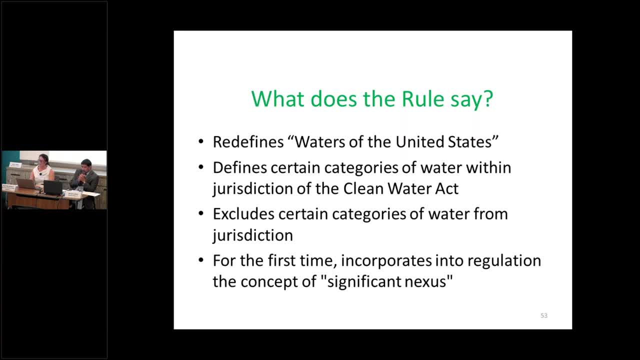 passes a law that doesn't have clear meaning, the court should defer to an agency's reasonable interpretation of the law. and in one of those interesting coincidences of life, EPA was then headed by Justice Gorsuch's mother, Ann Gorsuch, who's supportive. 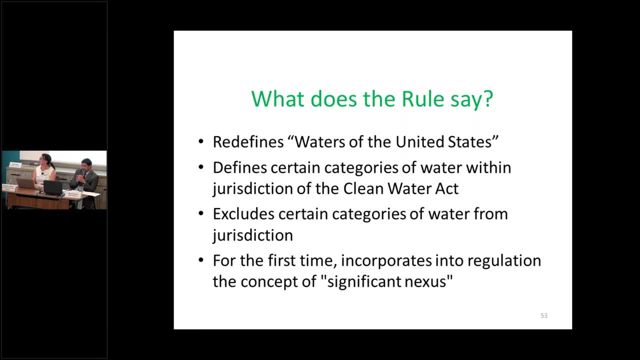 In that case deference, while Justice Gorsuch himself has been a vocal critic of the Chevron doctrine. the Chevron doctrine was heard in late May in oral argument on a petition to the court in another case out of the Ninth Circuit where a statute had been silent on. 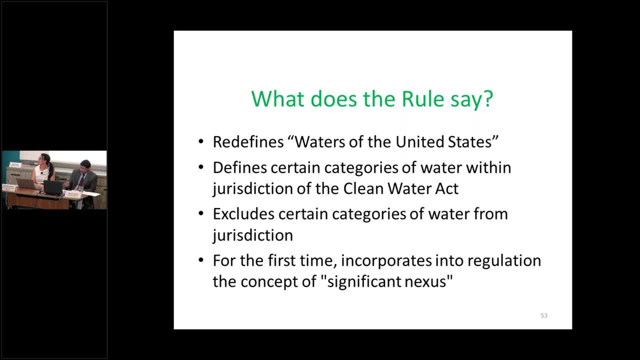 not ambiguous But given deference, and one of the parties had asked the court to consider the scope of deference as a result, arguing that deference applies when statutes are ambiguous, not when they're silent, and the court also sidestepped the deference issue and decided that case. 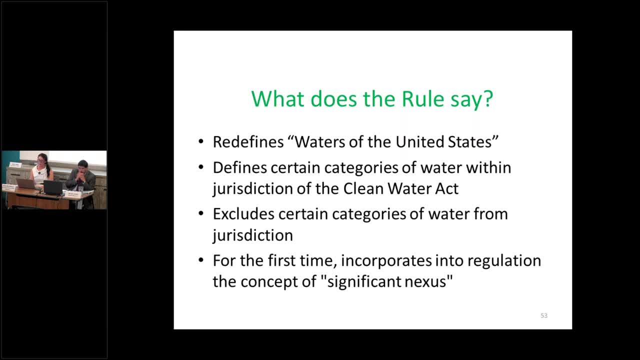 on other, narrower grounds, also a criminal case. so Chevron deference has been raised in connection with an agency. Before we continue, I'd like to make one last point. In the past Congress has been very objective about the status quo. We've seen a number of the recent jurisdictional issues under the Clean Water Act and it's 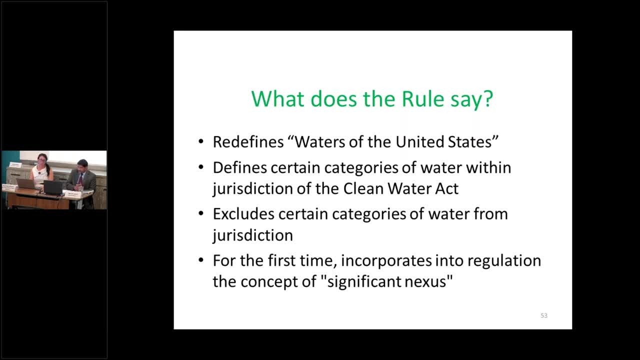 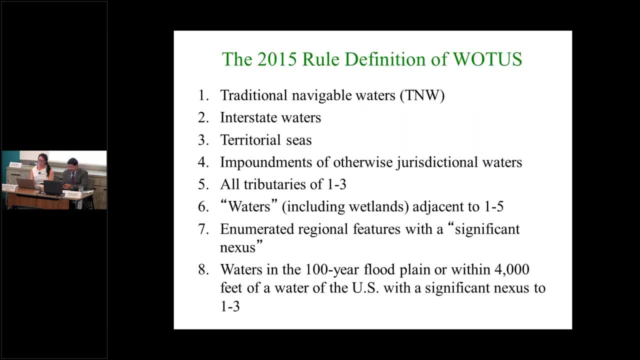 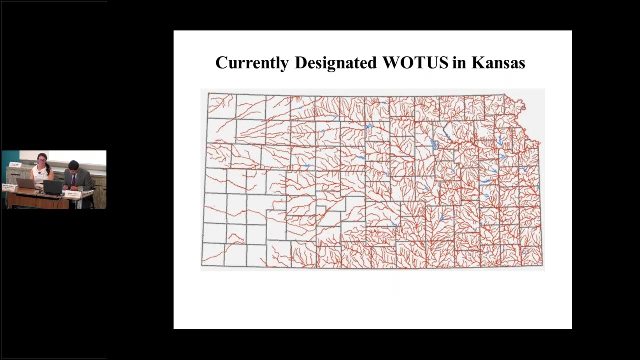 under a lot of debate as well. Next slide, please. Back to the WOTUS rule. Here's the definition of Waters of the United States that was put into the WOTUS rule. Next slide, please. Thousands of comments. The first one is why. 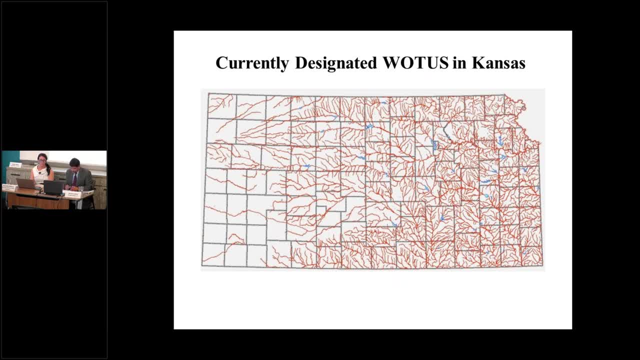 on the draft rule were filed by states, environmental groups, industry groups, trade associations, individuals, And this is just from one state, Kansas' comments. A lot of states filed maps like this showing the currently designated WOTUS in their state. 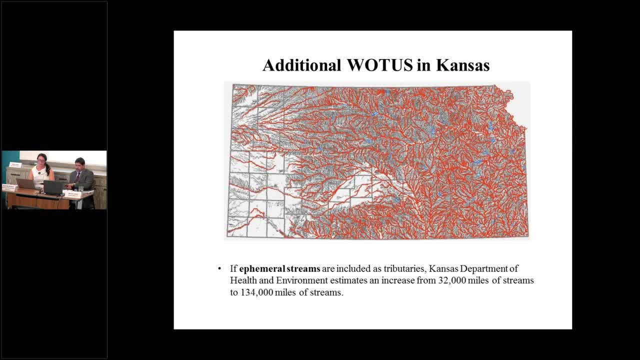 Next slide, please, And this is a graphic of Kansas' increased regulatory area and jurisdictional area under the Clean Water Act. under the rule, This is one of the disputes that has been a large part of the challenges to the 2015 WOTUS. 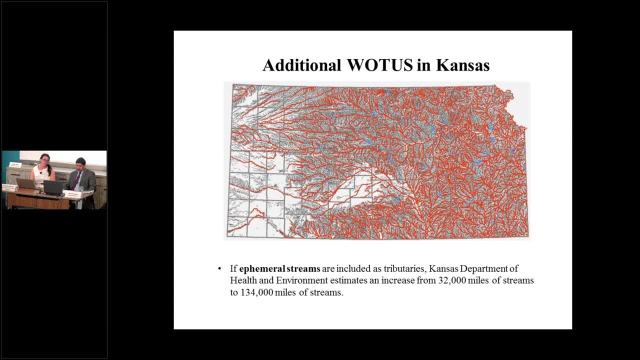 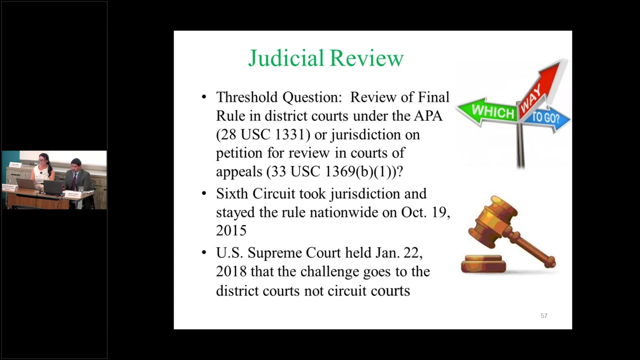 rule And you can see that the streams are many, many more miles of regulated area which, depending on your point of view, raises different issues for you. So next slide, please. So the 2015 WOTUS rule was published in 2015. 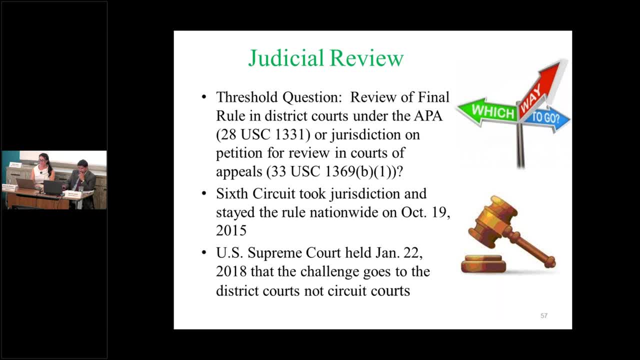 and immediately challenged. The Sixth Circuit took jurisdiction. after a lot of jumping around And after litigating for three years about where the rules should be challenged, which is not stated in the Clean Water Act, the Supreme Court said in January that the rules should. 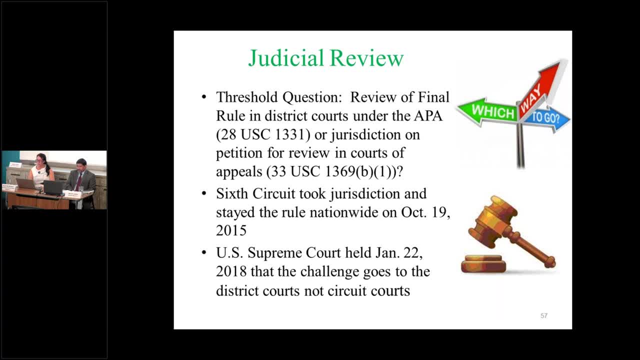 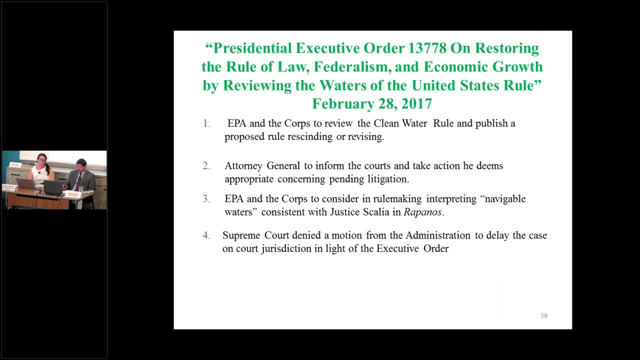 be challenged in the district court, not the circuit court. So challenges are beginning anew in the district court. Next slide, please. In the meantime, President Trump was elected And a month after taking office, the Supreme Court issued an executive order telling EPA and the Corps. 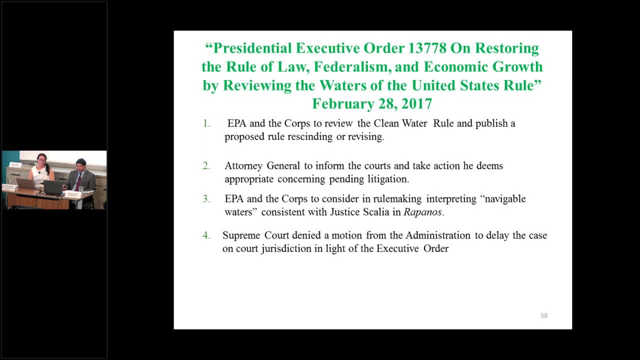 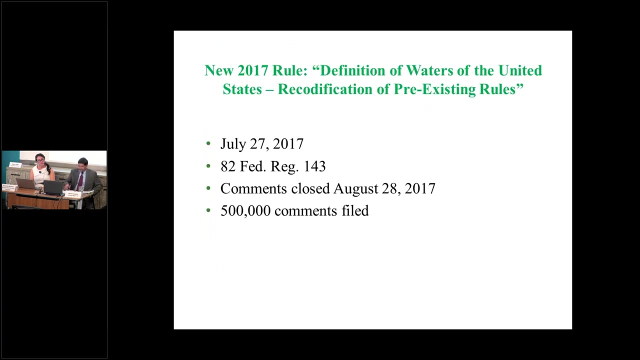 to resent or revise the rule and directed them to apply Justice Scalia's decision in Rapanos in considering any new rulemaking. interpreting what navigable waters means- Next slide, please. In response, in 2017, the Supreme Court put in place a recodification of the existing rules. 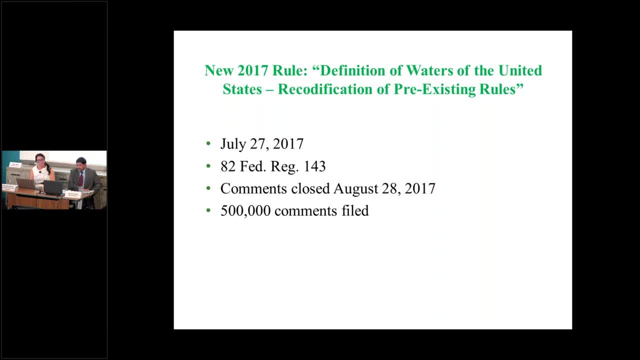 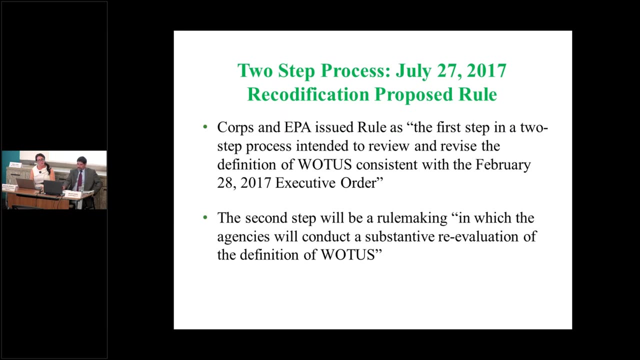 which are all from 2008 and are described in the outline and intended to bridge the new rule that will eventually come out from EPA. Next slide, please. That interim rule, the recodification rule, is also the subject of challenge in multiple lawsuits. 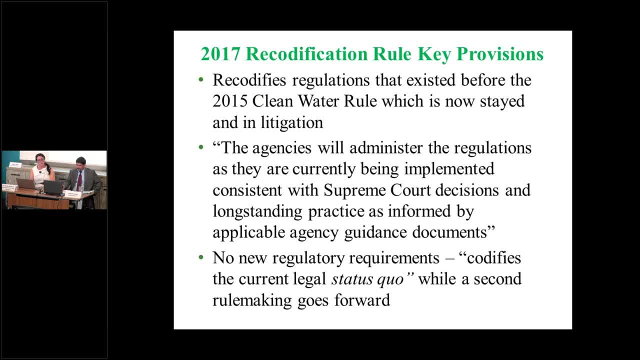 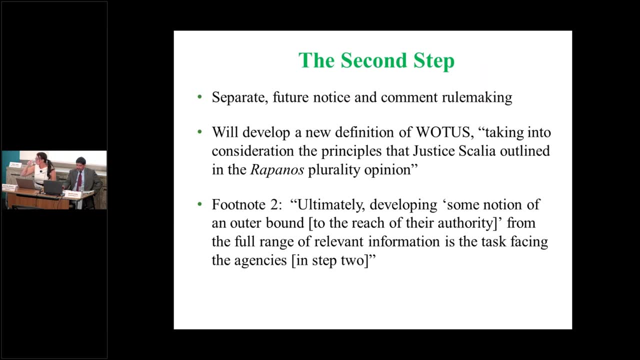 Next slide, please, Next slide, please. And, of course, it was intended to leave the 2008 status quo in place, which is what we're still operating under. Next slide, please. And just to note that it was noted in the recodification. 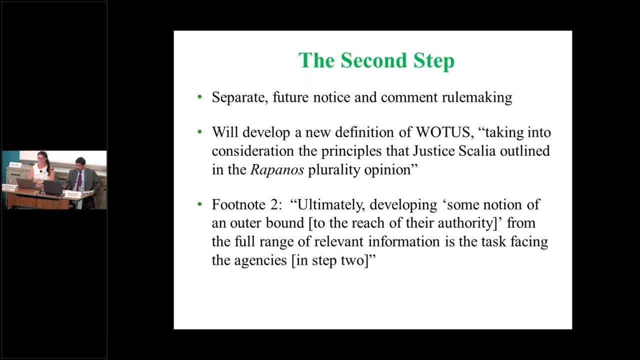 rule publication too. but even at the time of Rapanos pretty much everybody, including Chief Justice Roberts in his concurring opinion in Rapanos, had asked that a rulemaking be done to clarify navigable waters and waters of the United States. 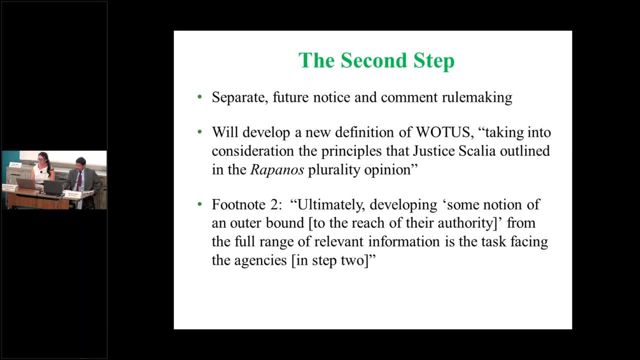 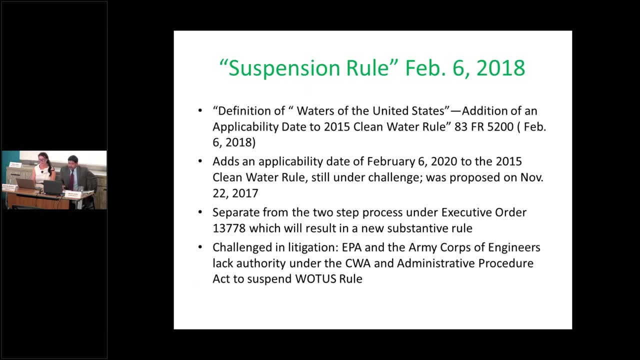 meaning under the Clean Water Act. Next slide, please. An additional separate rule was put into place in February of 2018, which is called the suspension rule. It's also being challenged In litigation and adds an applicability date of 2020 to the 2015 WOTUS rule intended to 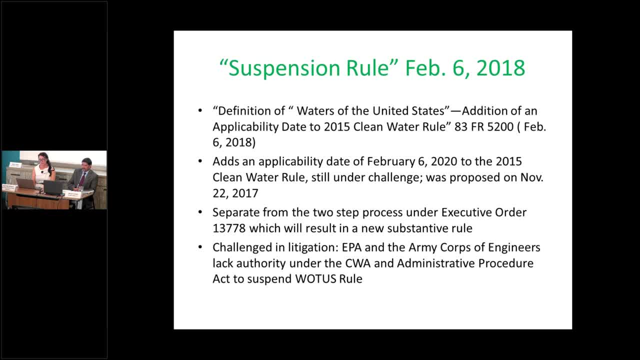 give the administration sufficient time to promulgate a new rule, And I guess what our takeaway can be from all of this is that it's a safe prediction that we're going to continue to operate under the 2008 regs for a while yet. 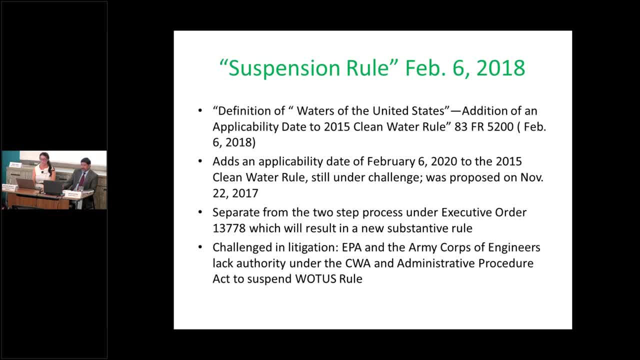 I'm going to turn it over now to Erika. Thank you so much for being here. Thank you. I'm going to turn it over now to Amanda, who is going to talk in more detail about permitting. Thank you so much, Thank you. 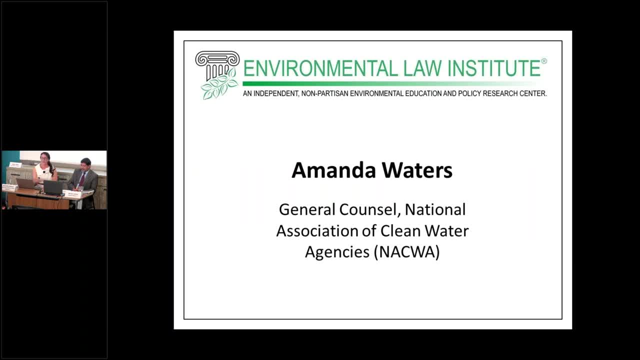 All right, good afternoon. I am so pleased to be with you today and I hope that you're taking full advantage of the ELI Summer Series. It's amazing And, just like your neighbor's newspaper, it's actually free. So I send, we send, NAWQA sends our interns here. 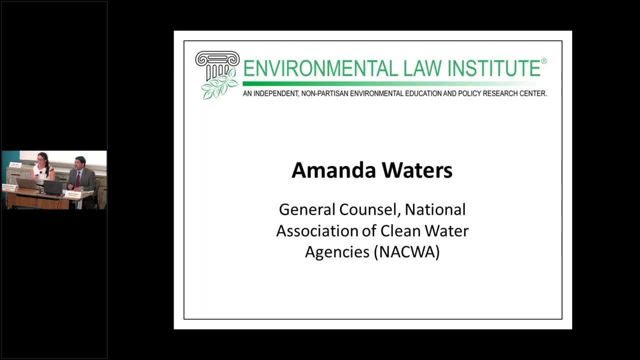 We've got one here today. Daniel is over here, So I work with you. I've been working with you, So I work for the National Association of Clean Water Agencies, and we are an advocacy organization that represents the interests of publicly owned wastewater and stormwater. 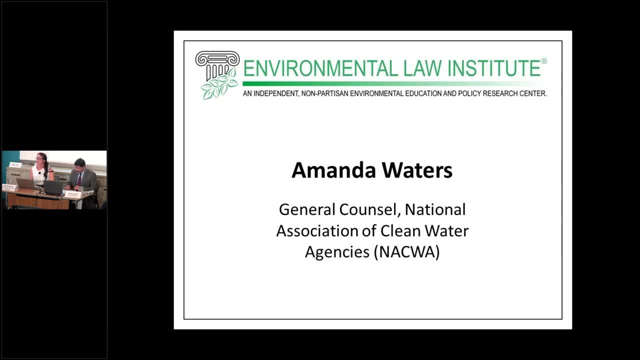 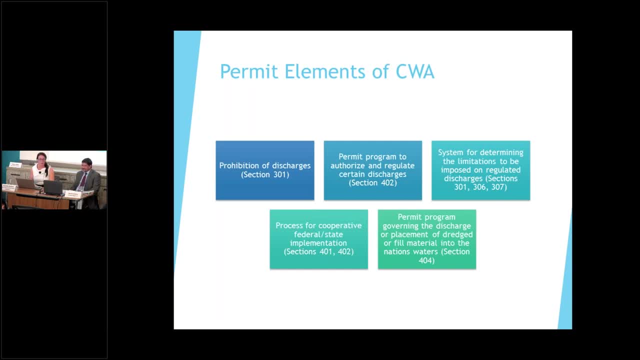 utilities across the country. So we are point sources And today I will be focusing on the permitting aspects of the Clean Water Act. Now, some of this David covered, as well as Karen, so I'll skim some of it. The general prohibition we've already discussed in Section 301.. 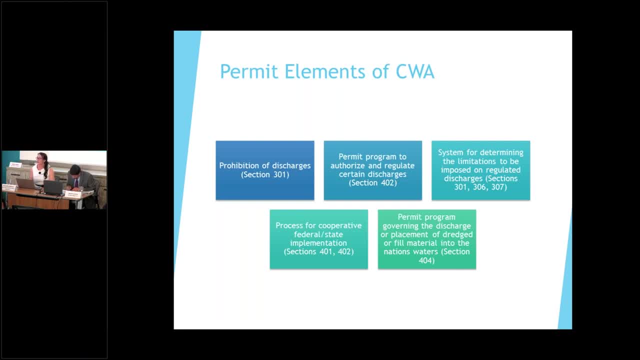 The permit program, the 402, that's the National Pollutant Discharge Elimination System permitting program. it's 402.. You have other sections that deal with the effluent limitation guidelines. We have process for cooperation between the federal and state governments and that's. 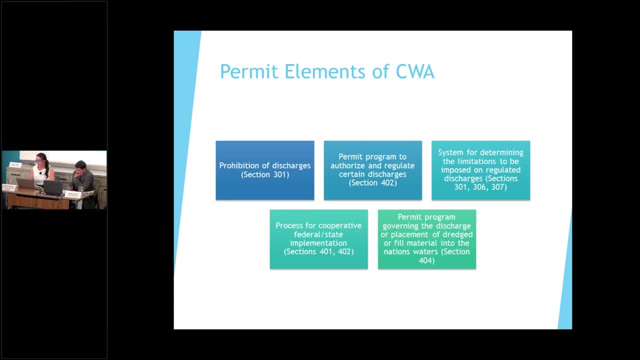 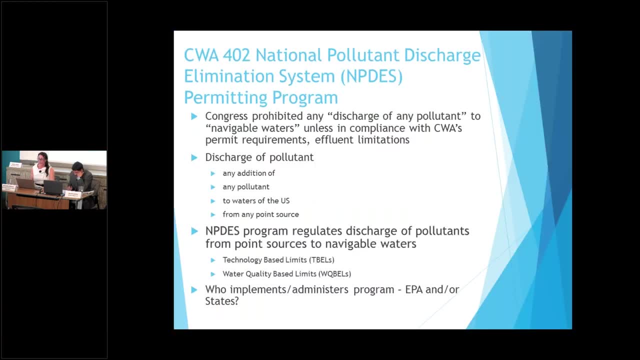 401, and there is 402 part of that as well. And then we have the dredge and fill permitting system, which is 404, and that has been discussed. So here again is the very broad prohibition When you look at the language of the Clean Water Act in Section 301,, discharge of a pollutant. 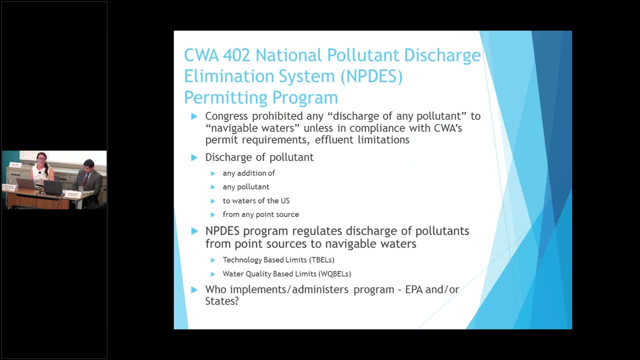 involves any addition of any pollutant to a navigable water or waters of the US from any point source. So David discussed addition very, very broad, or pollutant rather, is very broad. From a point source, though it's something that's very broad. 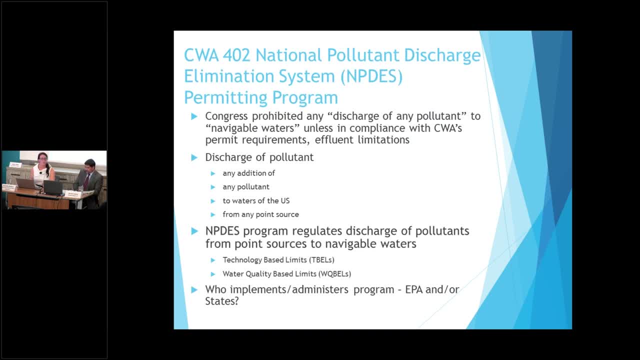 It's something that we'll discuss today because, in particular with regard to groundwater, there's been a lot of recent litigation. MPDS program regulates these discharges through technology-based effluent limits and water-quality-based effluent limits, and there are also TMDLs that are involved in how you set limits. 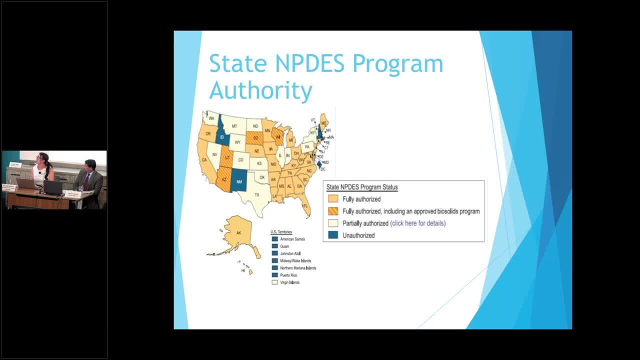 We looked at this or talked about this David did. this is just a map that needs to be updated. now, As I said, Idaho has received approval And Massachusetts may in another year. that may change. Now, regardless of who is administering the program, there's certain requirements. 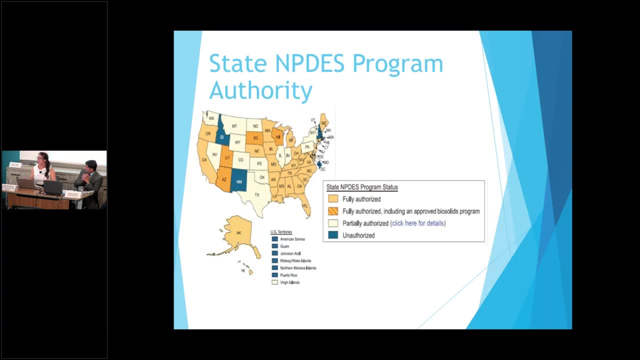 Permits have to go out for public notice and comment, There has to be an opportunity for public participation, And when states get delegated programs, their programs have to be as stringent as what EPA would do. And if a state isn't as stringent, then or is doing something improperly. EPA in theory. 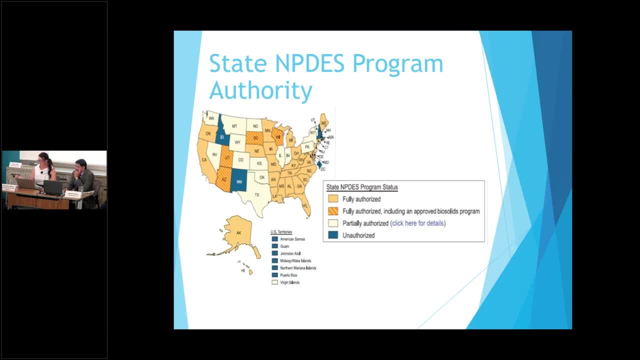 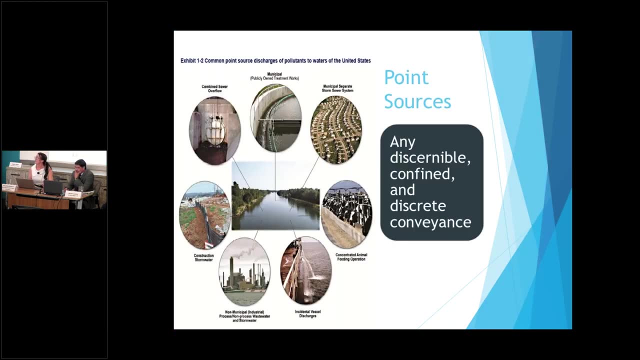 can withdraw. So that's one of the things that we're trying to do with that delegation: Point sources. Here are some examples of a point source which is any discernible, confined, discrete conveyance. We've got combined sewer overflows. 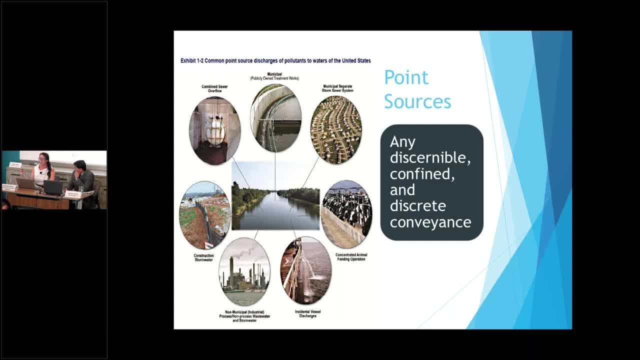 So that's something that we'll talk about a little bit more, but our members deal with that. DC Water here locally has combined sewer overflows. You've got municipal publicly-owned treatment works. You've got the stormwater system, the municipal separate storm sewer system or MS4.. 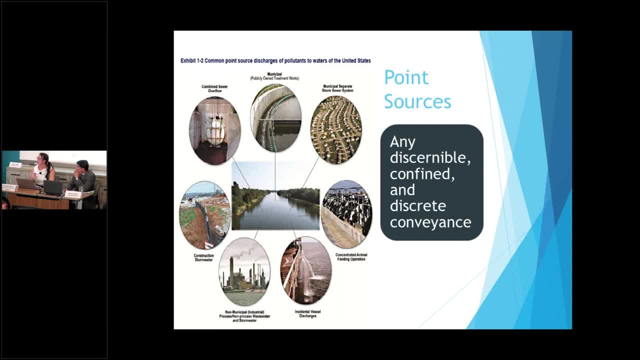 Then you have confined animal feeding operations, whereas agriculture is exempt. if it's confined and meets certain definitions, then it is considered a point source. You've got the incidental vessel discharges non-municipal industrial waste and then construction stormwater. 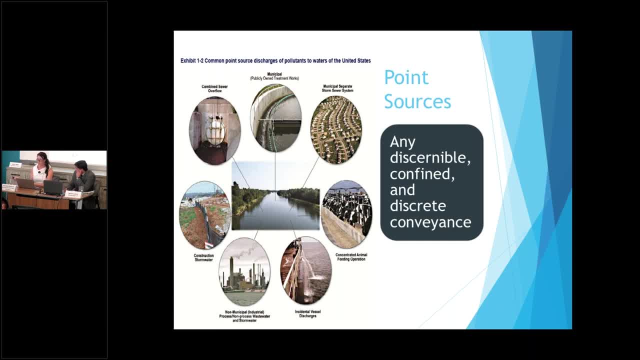 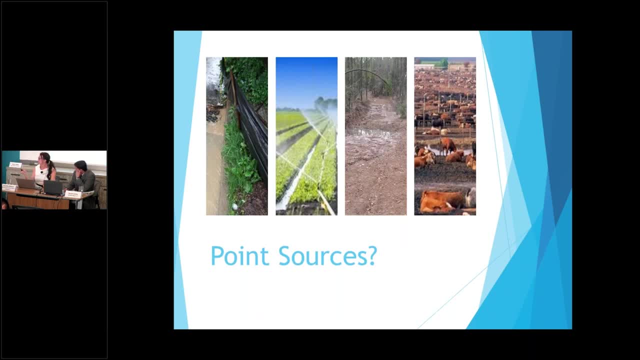 All right, Thank you, Thank you, Thank you. So a little quiz here, and those who are participating by webinar, feel free to participate on where you are. For point sources, here are four pictures, This right here. let's assume that this is a construction zone of more than an acre. 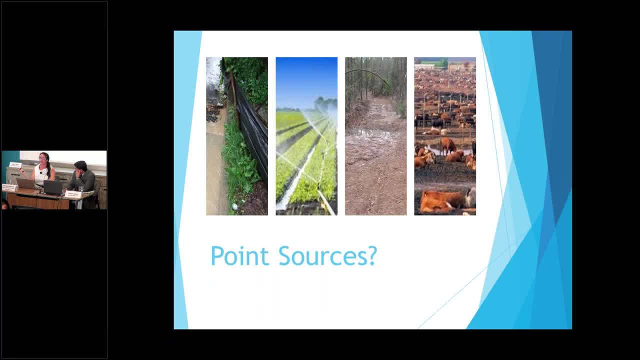 Would this be considered a point source regulated by the NPDES program? all we think: Yes, Yes, If it were less than an acre. if we are to assume that this is a municipal separate storm sewer system, then that would be a point source under the Clean Water Act. 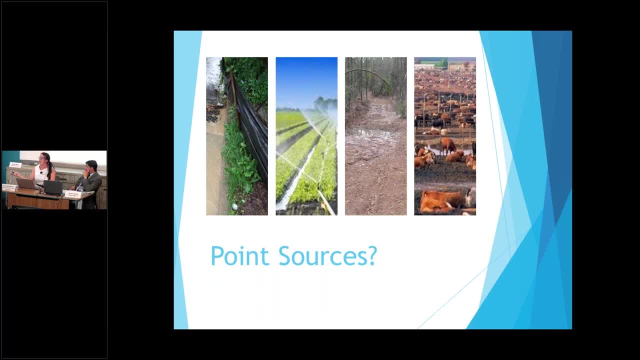 Here we've got return flow irrigated agricultural land, no exempt. This one is: this is a logging road, Assume this is US forest land, So logging road, stormwater it's channelized, Yes, Yes. 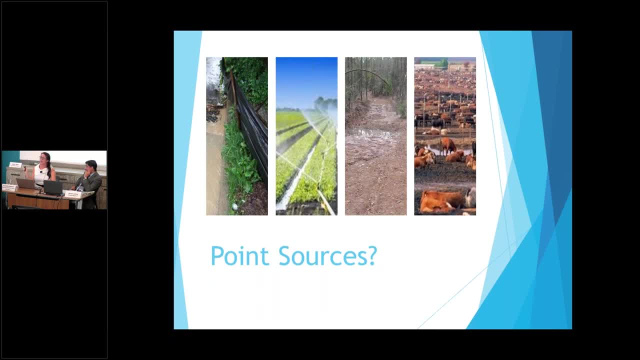 It's actually no. it's exempt as not part of it's considered stormwater and it's not part of the industrial coverage under stormwater. So there was litigation that went up to the Supreme Court on this in EPA rulemaking. 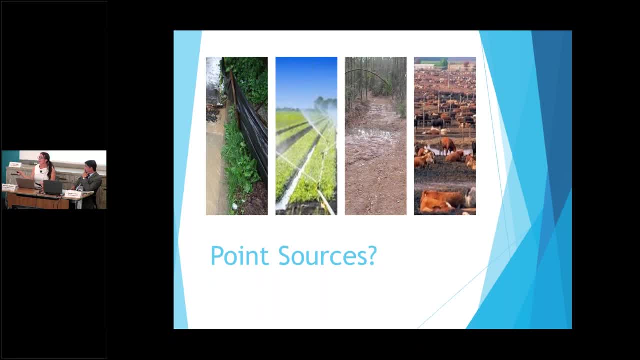 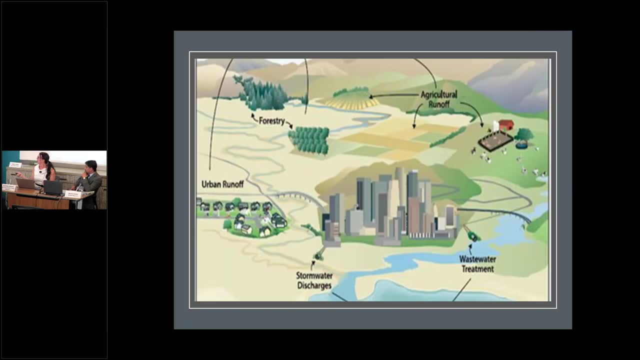 And I'll talk about that a little bit more in a bit. And then there confined annual feeding operation- we already covered. Say that again, Okay. So if you want to look at the landscape, if it's even Here, you've got wastewater treatment, you've got a city, you've got defined pipes and 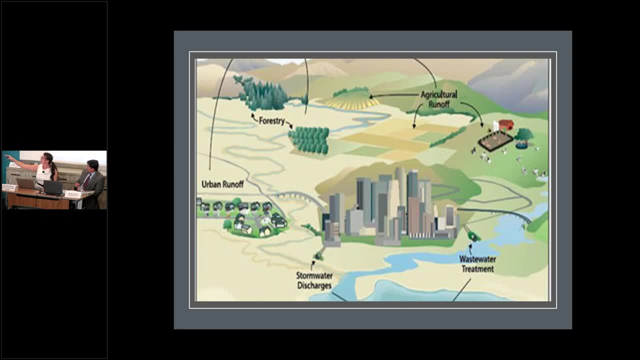 then you've got urban runoff, the stormwater discharges through streets and pipes, et cetera. So for those it's very easy when you're dealing with wastewater treatment, because you do have a pipe that extends and discharges into a surface water. 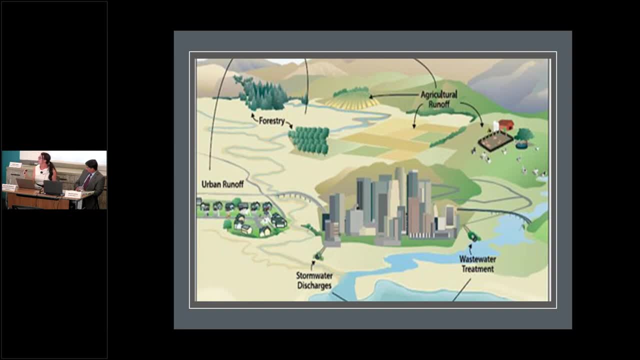 Stormwater discharges, it's a little more attenuated but it is covered. Forestry is like the example. If it's US forest land, then it would come up in that sense not covered And agricultural runoff again, only if it meets the definition of a confined animals. 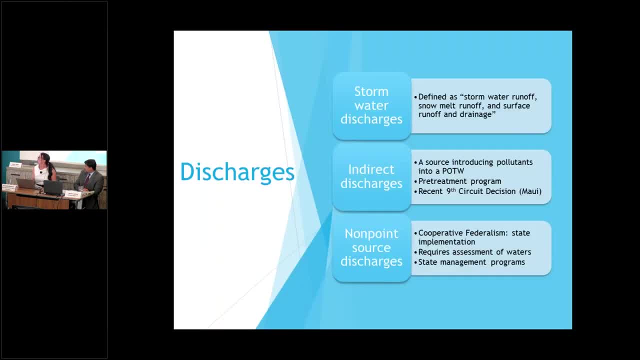 feeding operation. So when you're looking at discharges with stormwater, you really do have to determine: is it in one of those few areas that are covered, Because the rest of it is considered non-point source, diffuse and is then left to the states. 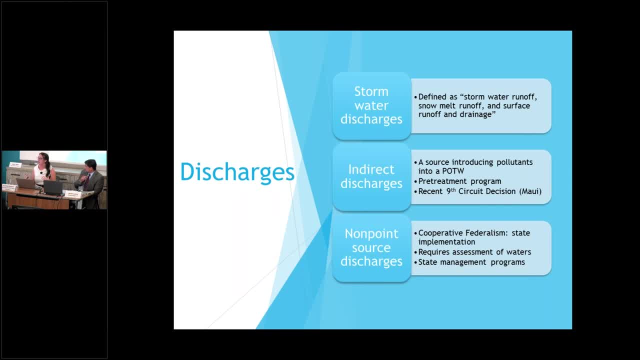 Under the, Under the federalism framework that Kathy touched on in her presentation. from the inception of the Clean Water Act, they knew that non-point source was very difficult to control, And so they set it up that the Federal Clean Water Act would cover point sources, but for 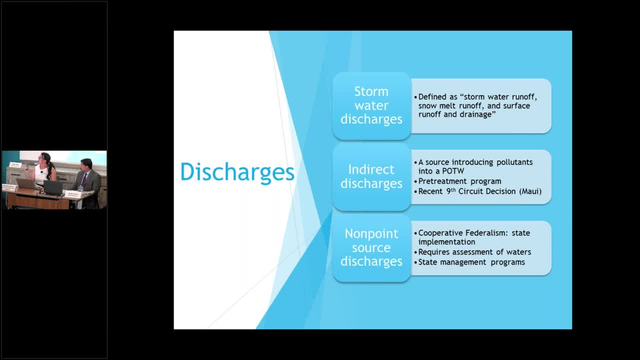 non-point sources, that would be the state's responsibility. Indirect discharges: this would be the pretreatment program. That's where you have industrial users. they discharge processed water into the wastewater system That goes to a POTW to be treated and they have to meet certain limits. 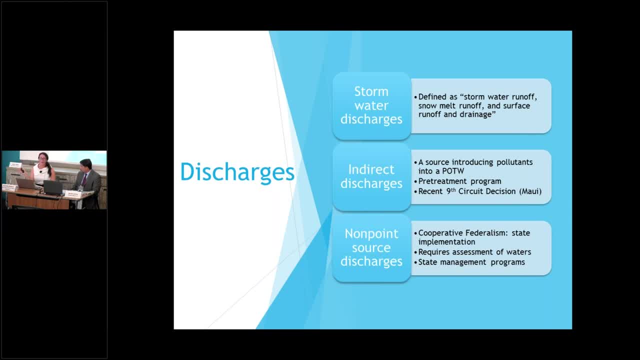 And, until recently, indirect discharge. when I heard this in the Clean Water Act context I always thought about pretreatment. But there is a case that just came down in the Ninth Circuit that discusses and created a new theory of liability called the indirect discharge theory, which I will talk about. 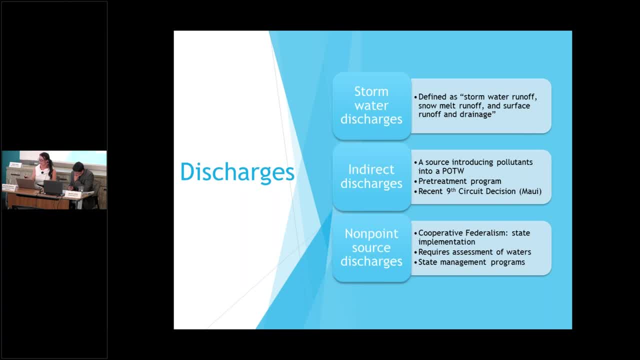 in a few slides. Non-point source. I already mentioned That is the state's responsibility Primarily Now. we talked about TMDLs and we talked about the Chesapeake Bay TMDL. There was a recent case. the American Farm Bureau challenged the Chesapeake Bay waste. 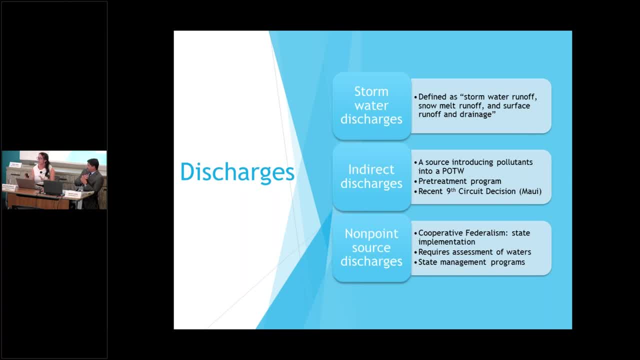 load allocation because there were allocations for non-point source. so they looked at it's a pollution diet. They looked at the Chesapeake Bay. they look at what it's impaired for, then they look at all the sources that go in and then they work with the states to attribute the waste. 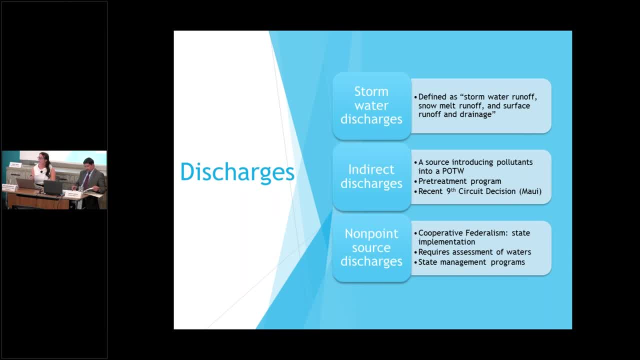 load allocation To those sources, non-point sources. it's permissible to have them brought into the fold in this manner. American Farm Bureau challenged that. It went to the Third Circuit, I believe, and then to the Supreme Court, And the Supreme Court did not review it. so the Third Circuit decision could, and it upheld. 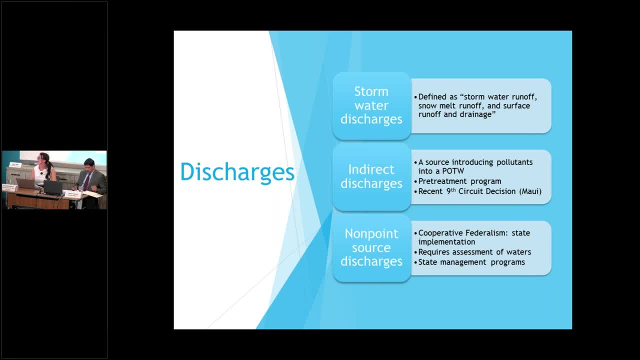 that watershed type of approach that includes non-point sources If you want to. For those of you, it's a great read. It actually explains. It explains really well how the Clean Water Act works. It's amazing. It's a long opinion but it's worth reading if you're interested. 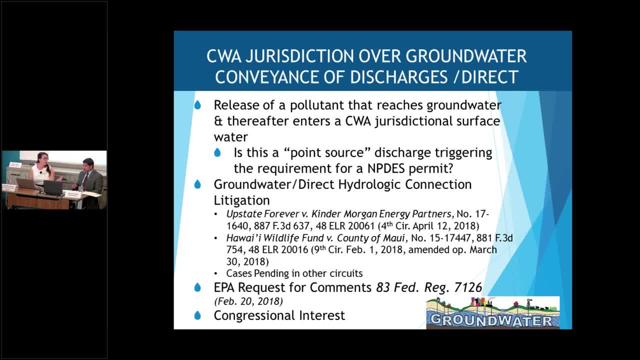 I have the site and I can give it at the end. Is it Third Circuit? Is that right? I think it's Third Circuit, but I can do that. Okay, He will correct me if I'm wrong. I will, It is the Third Circuit. 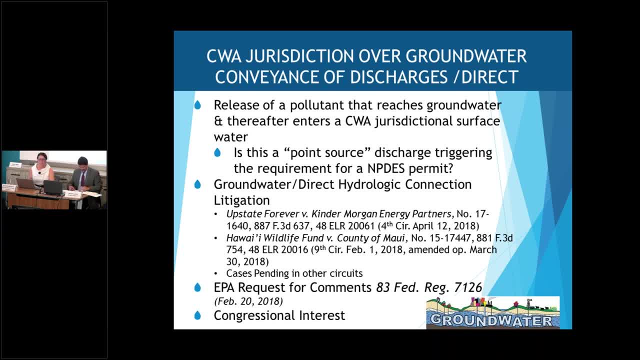 This is Elizabeth. Okay, Thank you. All right, Thank you, Elizabeth, may be covering this too. So let's talk about groundwater for a minute, because I think this issue is absolutely fascinating from an academic standpoint. It's kind of like a mini WOTUS. 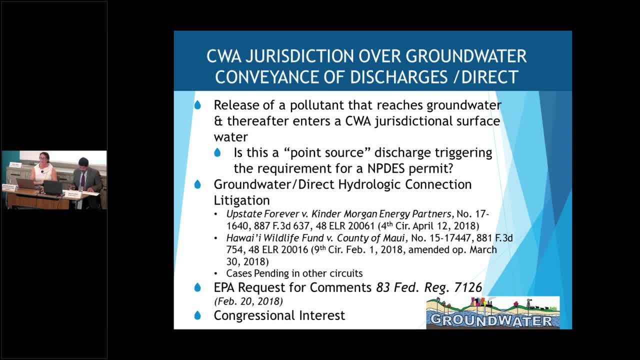 So the question here is not. it's not about jurisdictional waters, It's not whether groundwater is jurisdictional Courts and the Clean Water Act is pretty clear that it's not a water that you ask. But the question really is: is we have a relief from point sources, reaches, groundwater and 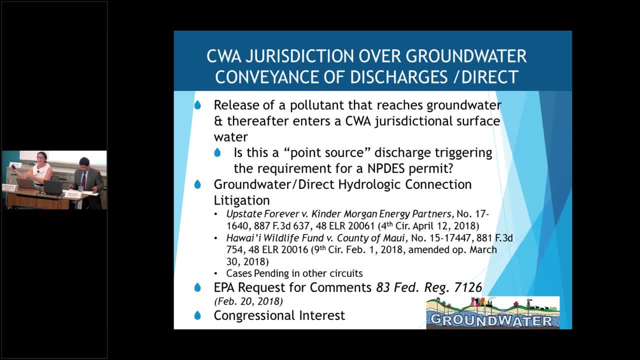 thereafter flows to a jurisdictional water, surface water wetland, whatever is jurisdictional, Does that? is that prohibited by Section 301 of the Clean Water Act? Does it trigger the requirement to get an NPDES permit as a point source? 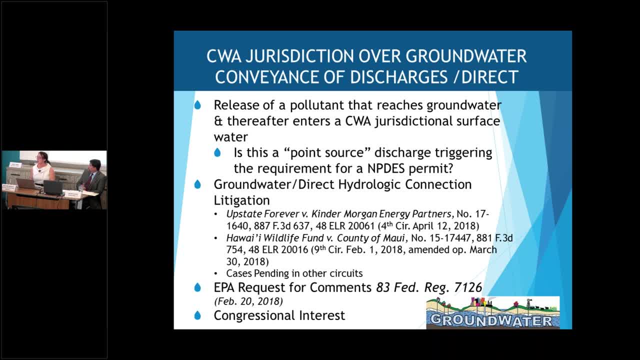 And it's difficult because where do you draw the line between non-point source and point source? So if everything that gets into groundwater and groundwater migrates to surface waters, if all that's covered, then it creates a lot of regulatory uncertainty about what needs. 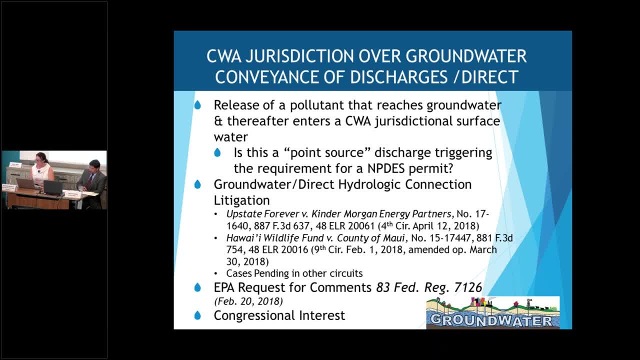 to be done what needs to be permitted, And this is coming up in litigation across the country. It's been litigated. It's been litigated for a long time, But in the last two and a half, three years we've seen an explosion of case law. 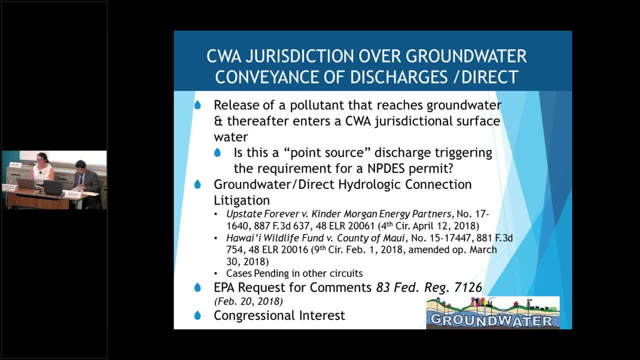 And environmental groups are using this cause of action. in cases It started with coal ash. So, like with coal-fired power plants, they have they have waste from burning coal that they put into ponds. Often these ponds because they have to be located near a surface water for their cooling. 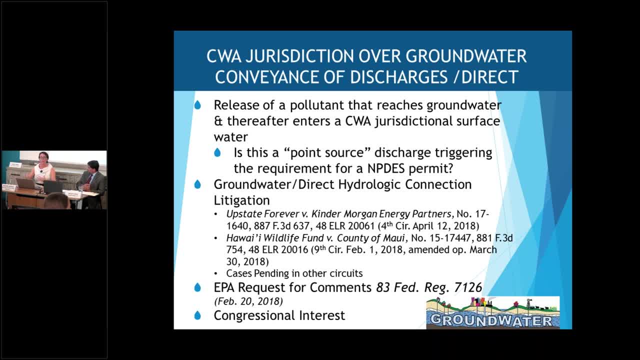 these ponds are located in very close proximity, Most of them are unlined, And so you can see how there would be toxics that would get into groundwater, and the surface water is right there. So our- our membership, though, is getting pulled into this, because you can't just if you're. 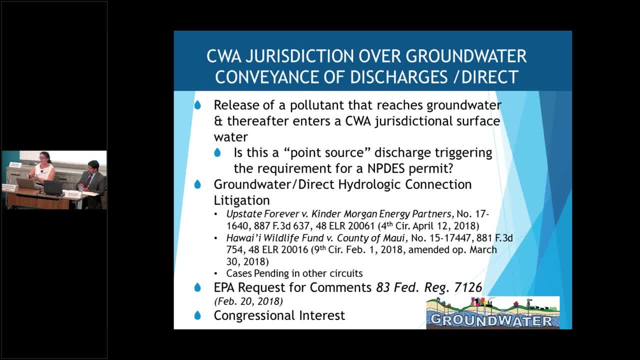 going this route through the Clean Water Act and the NPDES program. you can't just hollow out the coal ash. It would have to be applicable. the broader definition would have to be applicable to all sorts of these discharges. Okay, So I do want to go through just a couple of the cases. 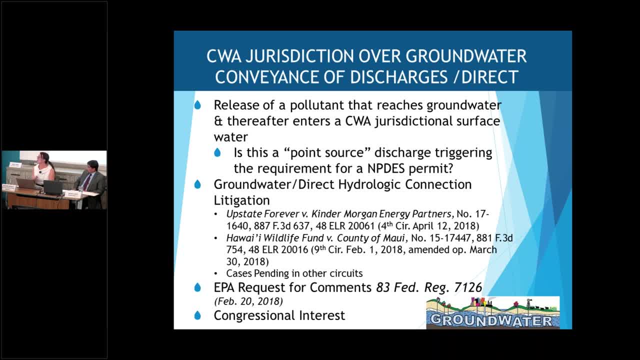 I'm going to start with the Ninth Circuit Maui case and full disclosure. Maui is a member of NAWQA and in that case they have a Safe Drinking Water Act permitted UIC underground injection well, So they they treat their wastewater from Maui to tertiary levels. 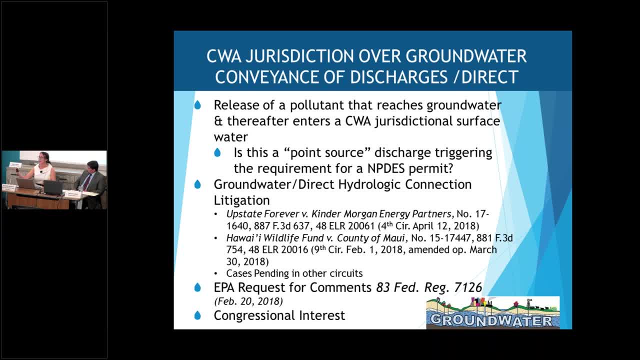 And then, through years of working with the state and EPA, they did not want to have an ocean outfall. So it was decided: inject that, get the Safe Drinking Water permit and you're covered. So they're in full compliance with their Safe Drinking Water Act permit. 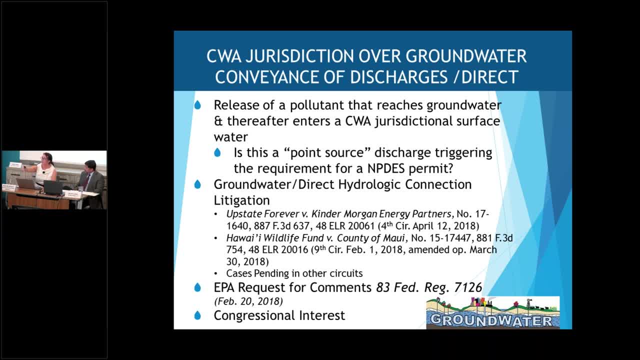 But what happened is is that, over an average of 10 months, the well water got into groundwater and then seeped along about a two mile area of the coast, And an action was brought by an environmental group saying that this requires an NPDES permit. 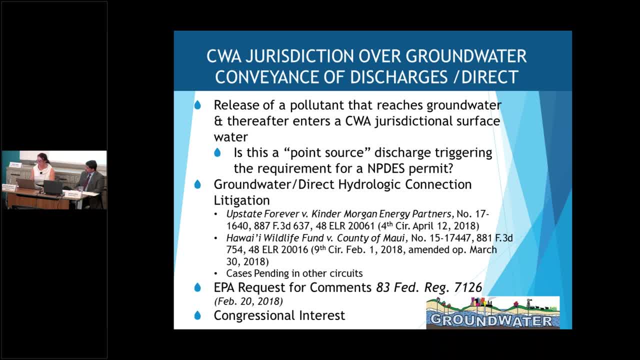 So this went up to the Ninth Circuit and there was a recent decision in February where the Ninth Circuit held That yes, an NPDES permit is required. Ironically, EPA had, under the Obama administration, they filed a MECAS brief proposing they're. 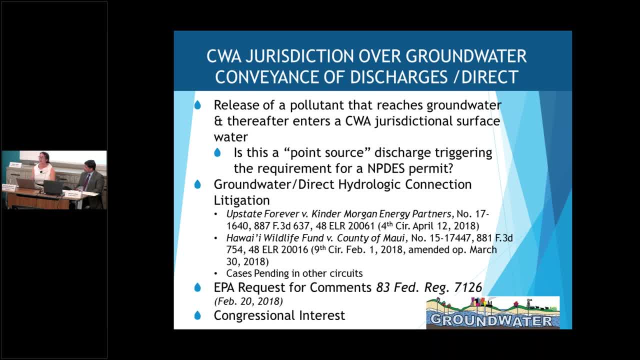 saying that this is a clear, direct hydrologic connection. So where that happens, you have, you have a discharge from a point source. it's clearly connected to surface water. therefore, that is the equivalent of discharging to a surface water. The Ninth Circuit shot that down. 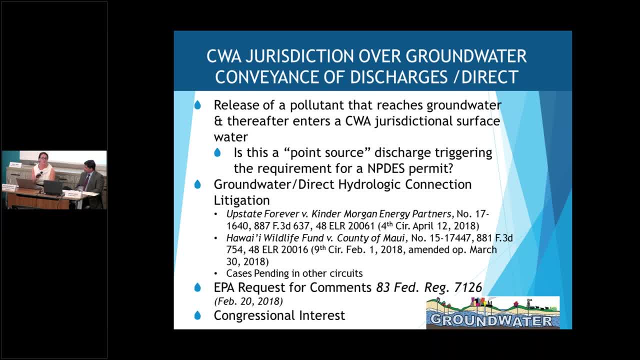 They said that language appears nowhere. A direct hydrologic connection appears nowhere in the Clean Water Act. But then what the Ninth Circuit did is go on to create their own test, which is this indirect discharge theory. And what they said is: you've got to have a point source, you've got to have a fairly 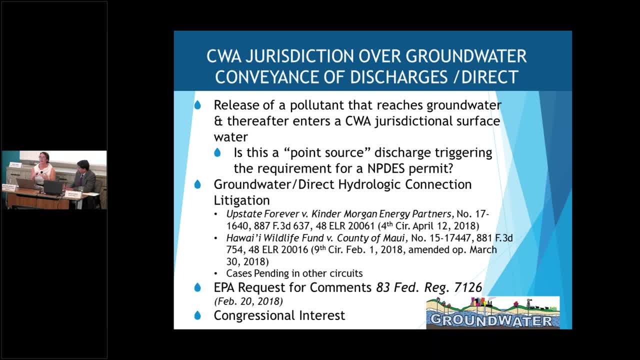 traceable discharge. So it's got to be the functional equivalent of a point source. So it's fairly traceable and more than a de minimis amount. So that was the standard that the Ninth Circuit created. Then you have the Fourth Circuit. 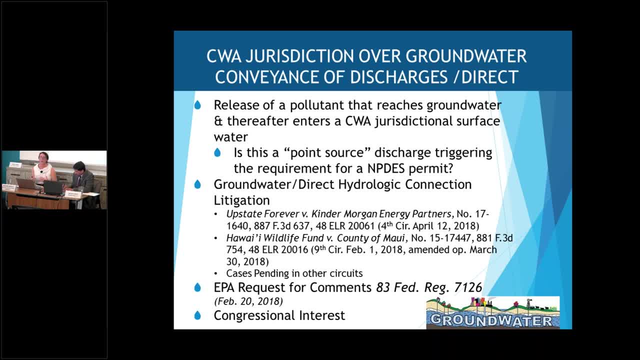 And this is a different case. this was a petroleum spill. So you have a pipeline. the pipeline broke, you had a nasty oil spill. environmental damage that seeped into the groundwater, got into a surface water. Here it was a split decision, unlike the Ninth Circuit, which was unanimous, but they did. 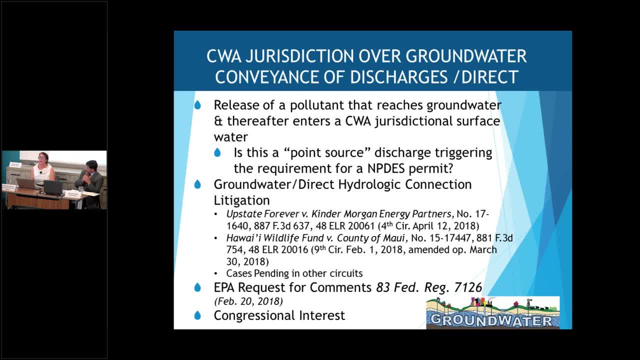 find that there was a Clean Water Act liability requiring a permit. They used EPA's direct hydrologic connection theory to base that on. But they then reconciled. They said: well, it's pretty much the same as what the Ninth Circuit found. 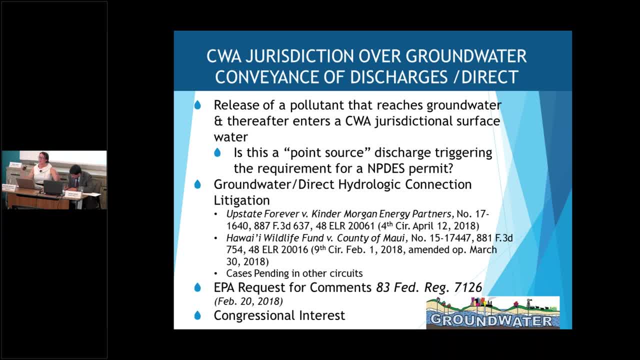 So now you've got two circuit court cases And you have a 1994 Seventh Circuit case that many argue creates a split in the circuit. So all this is going to go up to the Supreme Court. late summer It'll petition the Supreme Court for review. 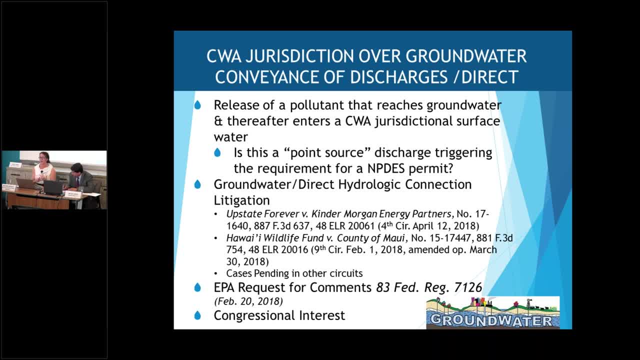 Whether the court takes it depends on a lot of factors. A circuit split is definitely one that would prompt them to accept it- EPA's action on this, Whether they think it's That's Chevron deference, Whether they think the statute is clear and they could step in and be the appropriate. 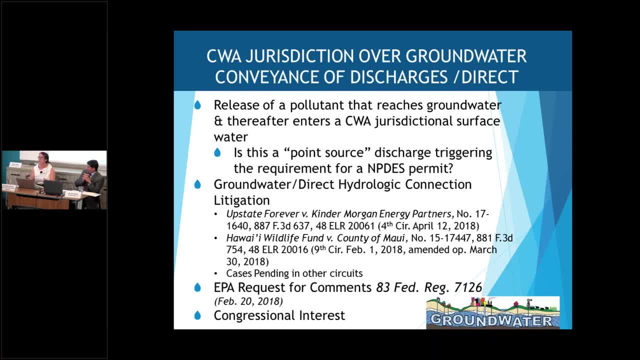 body to say: the statute's clear, either it's in or it's out, Or do they think it's ambiguous and should be left to EPA? So through this, you have EPA putting out a request for comments. This is not a request for rulemaking. 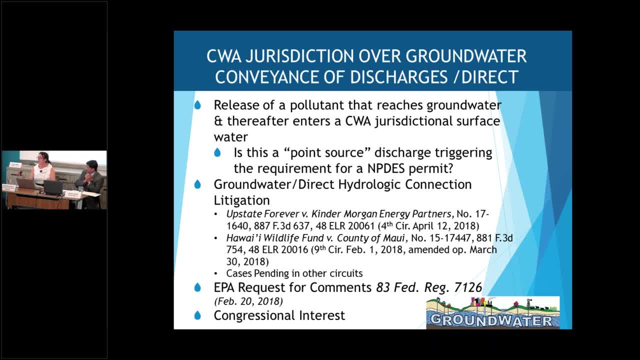 It's sort of they're trying to show that they're doing something on this issue. So in February they put this out. The comment period has closed. What they do with those comments we don't know. Are they going to come back with a statement? 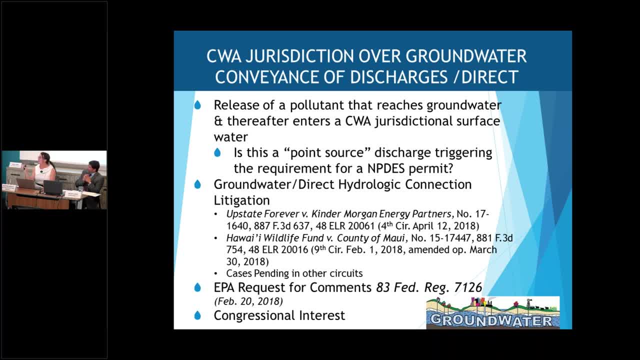 Are they going to come back with a rulemaking? So there's a lot to watch here, including congressional interest. We have Congress. the Senate Environmental and Public Works Committee held a hearing. There was something in the 2018 Omnibus Bill about having EPA come and report back on this. 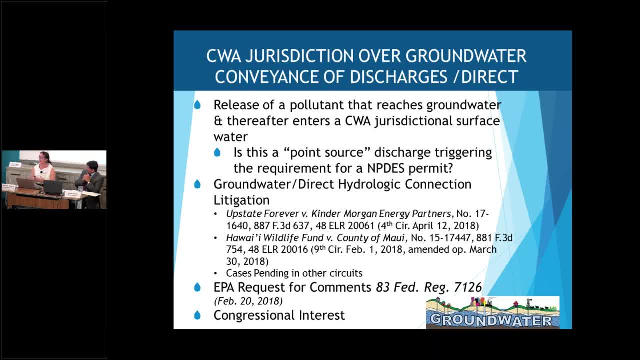 issue With Republicans in control. they very much want there not to be a permit requirement. But there's a great paper that is posted on the ELA website- The website for this series- and Kathy wrote it And it gives. if you want to know more about this, it gives a lot more information, including: 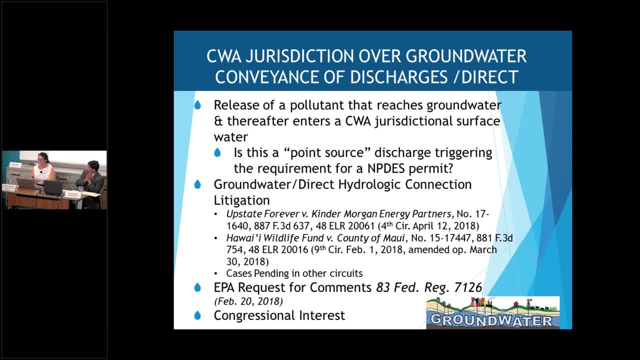 the cases Kathy also submitted. I testified before the Senate on behalf of NAWQA, but I advocate a position, So I'd rather you read Kathy's and then you can decide on your own what you think. And I don't know about what EPA is doing, by the way. 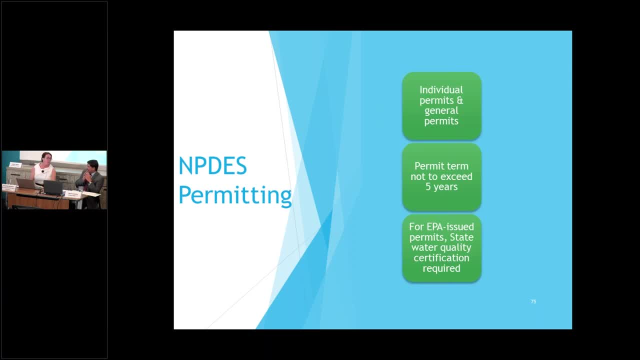 Yeah, Funny enough, EPA, and there's some litigation in New England right now on septic tanks And septic tanks. same thing You would think that they would. they would say yes, But they don't. They don't have a direct hydrologic connection theory, because there it exists. 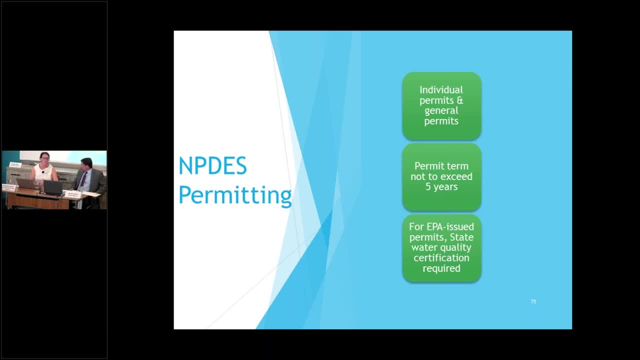 Well, they took a 180 view saying no, this is never a point source, So they're going to have to reconcile that. And just one more interesting note on that: In one of the cases in the Sixth Circuit it's the Tennessee Valley Authority. 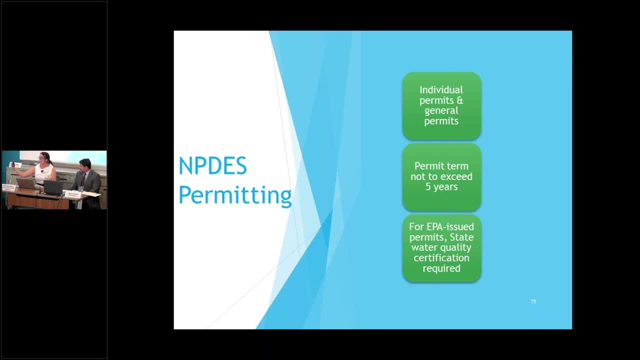 So when it if and when- and they intend to appeal this- to petition the Supreme Court for review. If it gets to the Supreme Court, it's the Department of Justice that will have to represent TVA in the Supreme Court Right. And the Department of Justice is on record in the Ninth Circuit as supporting the direct. 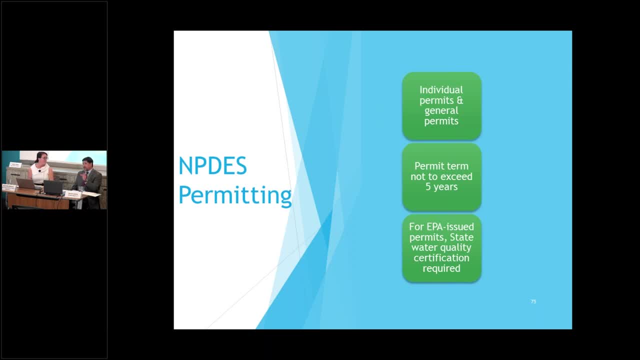 hydrologic connection theory. So it would be the Solicitor General's Office, along with, actually, the Environment and Natural Resources Division, has an appellate section- that will be leading the effort in these cases. It's an interesting sort of entanglement. One important thing that we- I think I was supposed to say at the beginning, but remember- 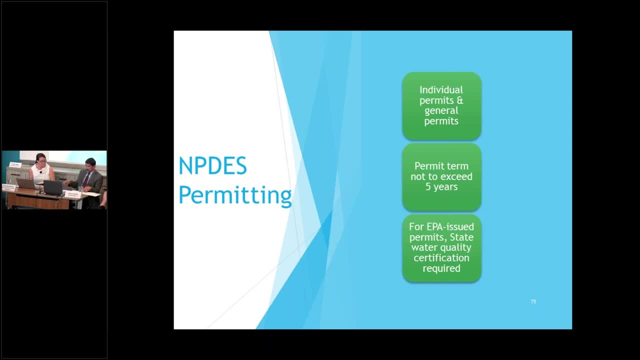 that the Clean Water Act protects surface water. We're not dealing with the groundwaters. That's what all these complexities come to be. But the reality is we're protecting on the ground. Yeah, Under the Clean Water Act, we're protecting surface water, the rivers, the lakes, et cetera. 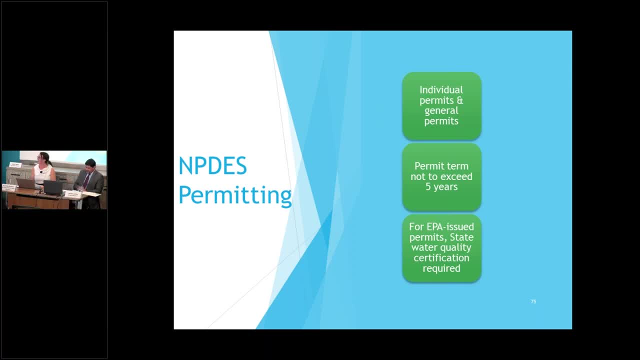 Does that make sense? Yeah, Thanks for that clarification. With NPDF permitting you can have individual or general permits. Individual is what it sounds like. You have particular requirements that are tailored to that given discharge. Then with general permits, you have an activity that's similar where you could have a general. 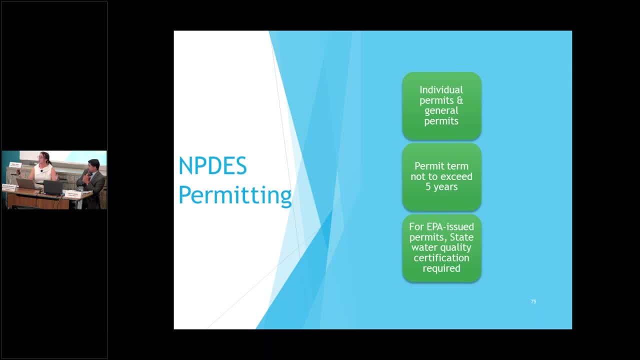 set of requirements that would cover anybody who then files a notice of intent to become a public servant. That's covered under there. If they meet qualifications, the eligibility, then they can get a general permit. Permits do not exceed five years. They have to be renewed and reissued on a five-year basis. 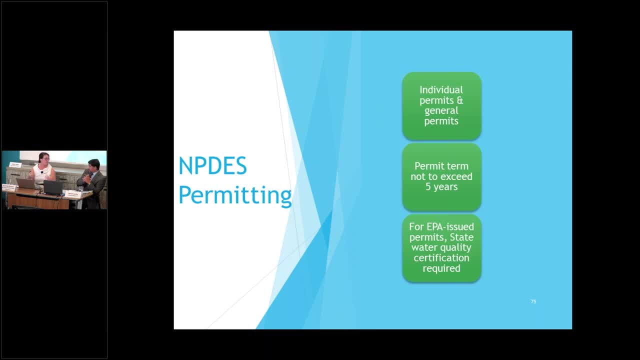 However, there are many, many that are administratively continued because resource- it's a resource issue for states to keep up with this permitting cycle. So what happens then? You just abide by the existing permit until you get your new one. We already talked about water quality certification. 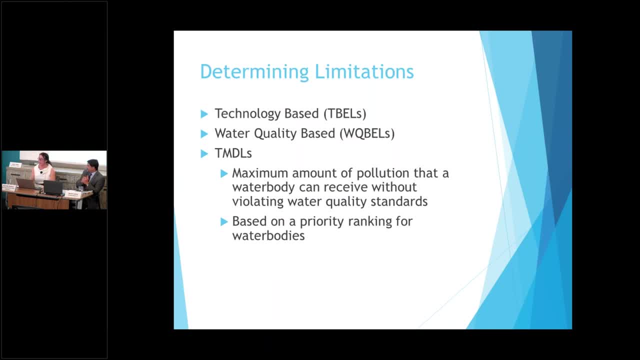 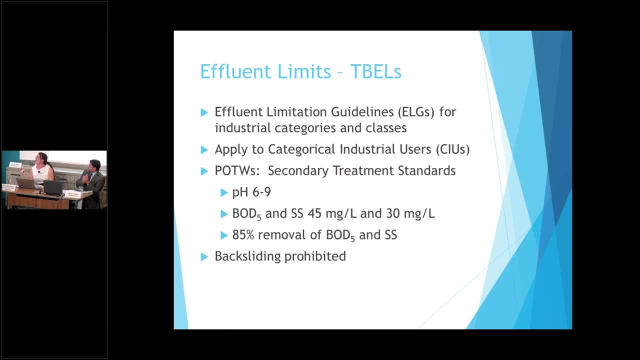 So let's talk about that. Let's get into technology-based effluent limits. We've got water quality-based and TMDL Technology-based are, if you think about, you've got the discharger and then you've got whatever's being discharged in the water body. 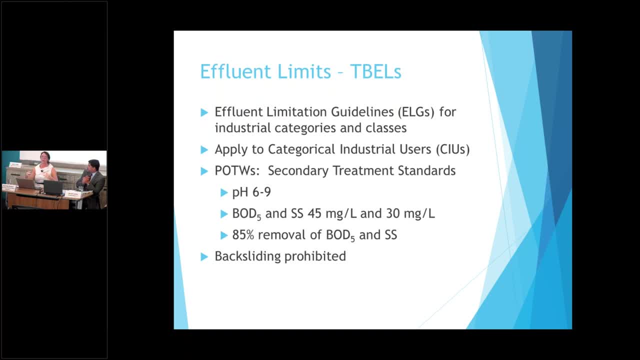 Technology-based is not focused on the water body, It's focused on it was like the first step of the Clean Water Act. Let's see what's possible through technology and then, looking at these categories of industry, such as publicly owned treatment works, you set up technology requirements for what can? 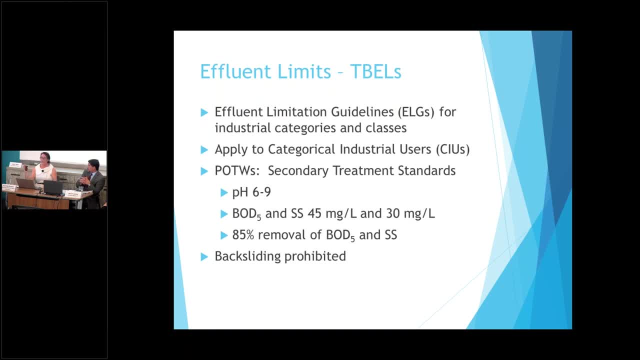 be achieved. And then those they look at technology. they don't look at what's happening inside the plant. They don't. well, they actually say, do this meet these levels? and you can't, they can't control sort of how you meet those as long as end of pipe, you're meeting those levels. 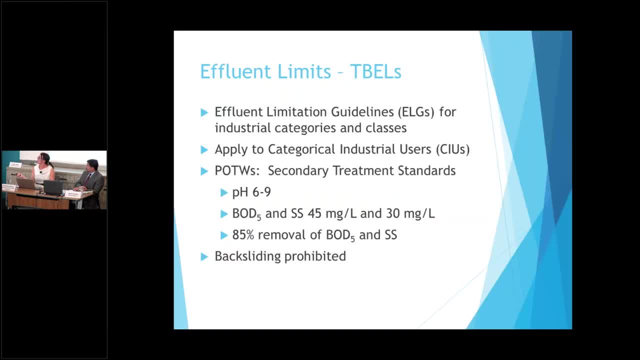 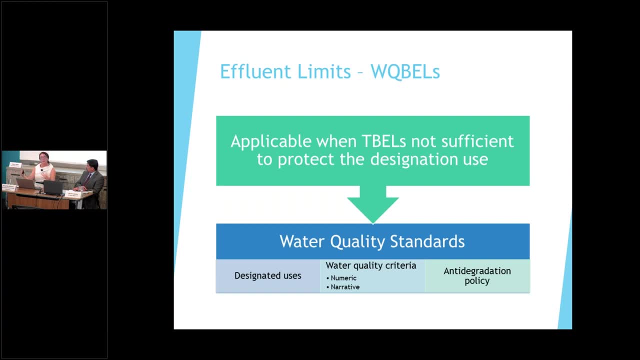 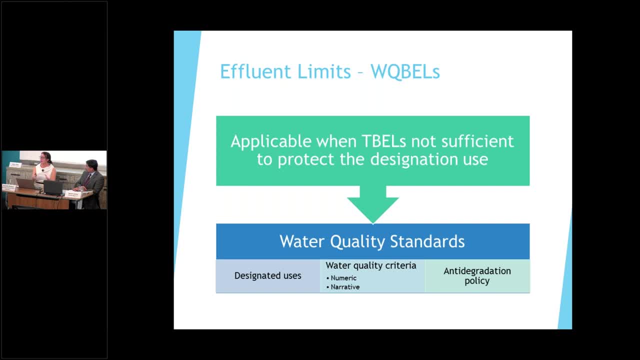 effluent limits are achieving And if, through those limits, you're not able to comply with water quality standards, the criteria, then there's a process. this is- and you mentioned this, it's a much more analytical, scientific process, where you have to look at those standards and figure out what the 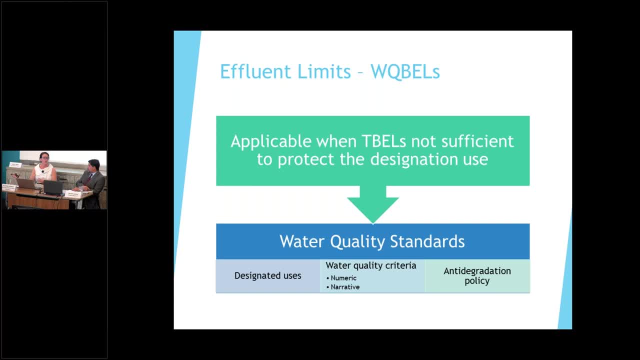 limits will be in order to maintain the designated use of the receiving water body. Okay, So for water quality criteria, you've got both numeric and narrative. When it's narrative, it could be no toxics and toxic amount, So there's a process for translating those into numeric. 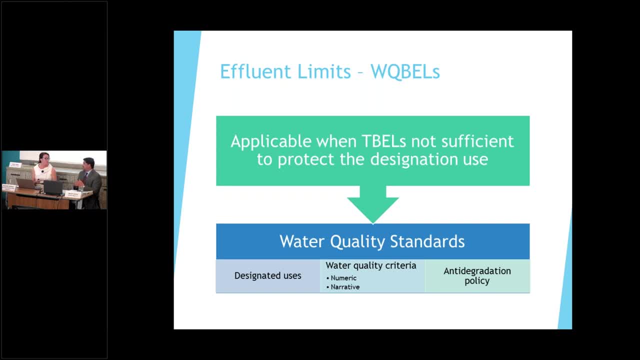 It's more complicated, especially when dealing with something like nutrients. It's very complicated. Anti-degradation policy applies to water quality-based- You touched on this- For technology-based. it's anti-backsliding, so that means if you're issuing a new permit. 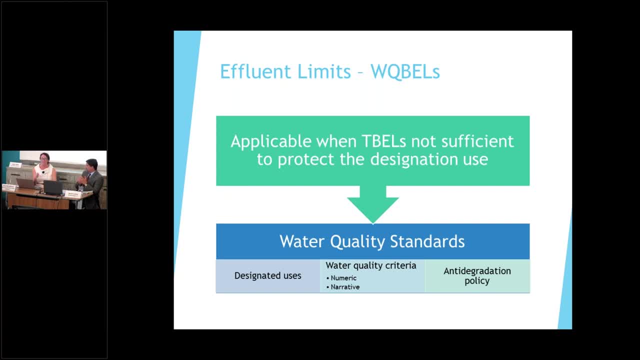 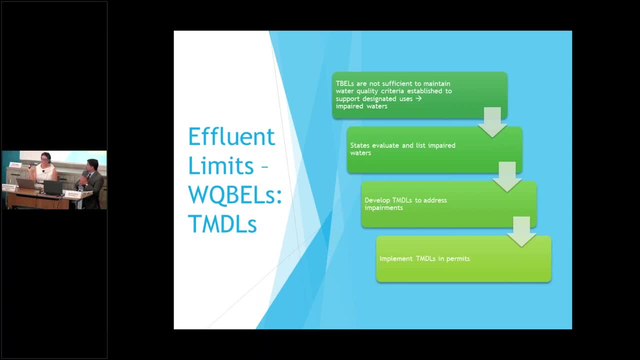 you shouldn't have less stringent requirements and limits than the previous permit. There are some exceptions. for the most part, that's what you need to know. TMDLs. I think that we have covered this pretty well and I'm running out of time. 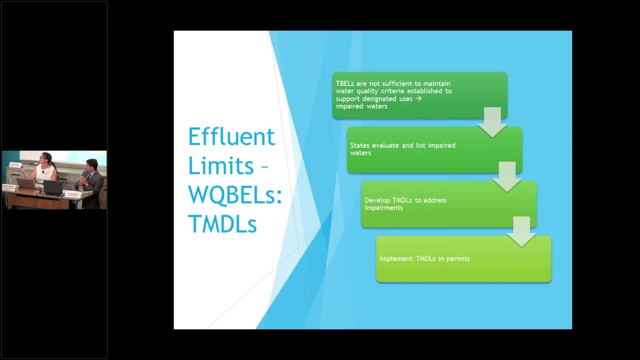 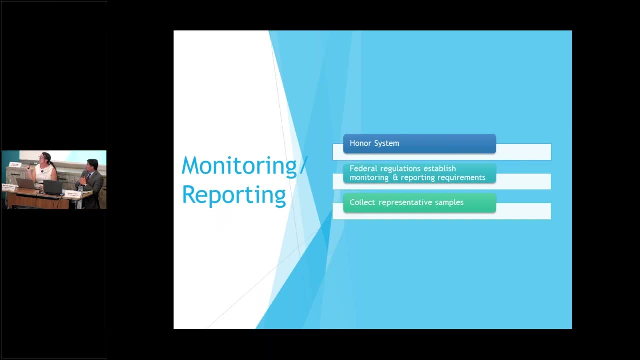 State responsibility to list their impaired streams and then develop TMDLs and implement these in permits. So that's going to also be part of how you come up with your limits. Monitoring and reporting- This is an otter system, So dischargers will complete discharge monitoring. 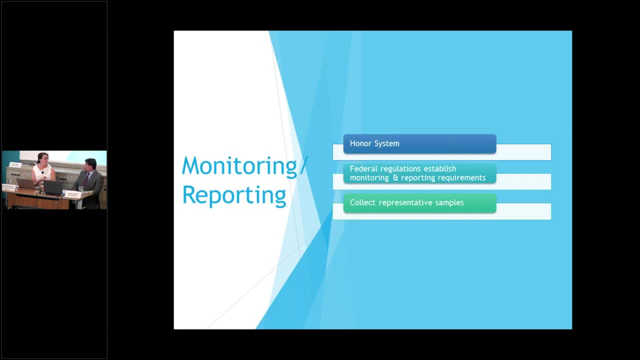 Many of them are doing this electronically. finally, they're getting into the 21st century, So the federal and the federal regulations will set what those reporting requirements are and then they will collect representative samples based on what the pollutant is. It could be a 30-day geometric mean, it could be averages, that sort of thing, and they 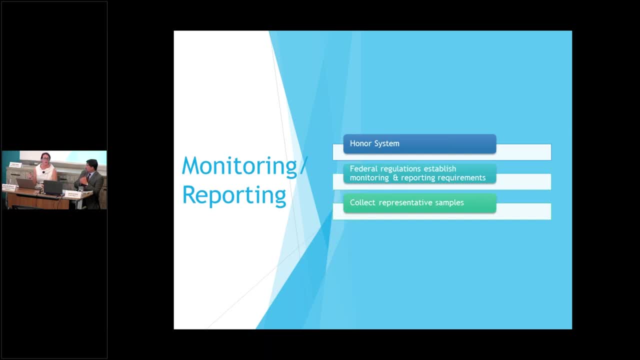 report it And then the permitting agency, whether it's the state or EPA, reviews that and if there are violations they can go and report it. They can go and bring enforcement against the discharger. Moving on to wet weather permitting. 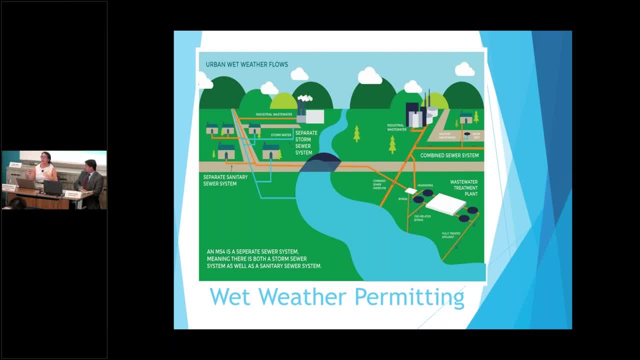 So you have the Clean Water Act in its beginning and it's really focused on continuous discharges, where it's going all the time. But then in 87, they amend things to address stormwater because they're seeing that we're getting the point sources under control. stormwater is an issue. 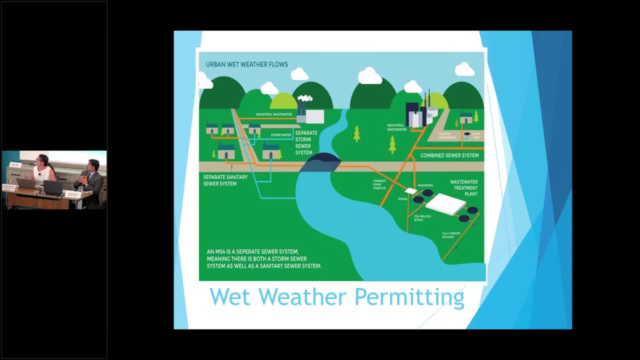 And so they start looking at stormwater. And so they start looking at stormwater, And so they start looking at ways to address stormwater in addition to combined sewer system overflows. A combined sewer system- we have it here in DC. 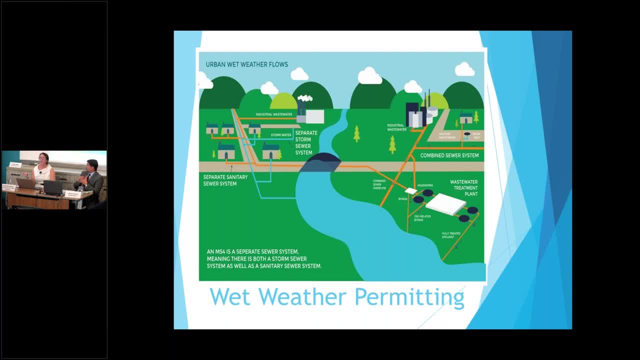 You find it in a lot of older cities. It was considered very efficient at the time. It's where you have your stormwater and your wastewater, So you have your household waste coming out of a building here when you flush the toilet or put something down the sink. 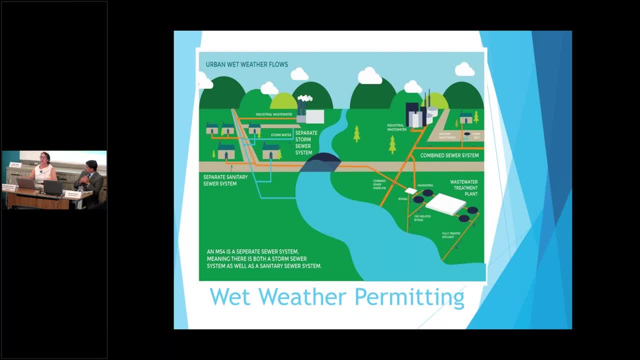 And then, when it rains, you have your stormwater basements that capture water. What happens is that you have a lot of waste coming out of the building And then, when it rains, you have your stormwater basements that capture water, And then, when it rains, you have a lot of waste coming out of the building. 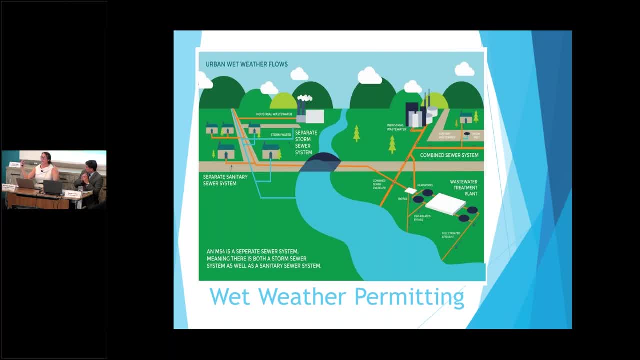 What happens is that you get a lot of water mixed with sewage in your pipes when you have heavy rainfall and that inundates the system. Your treatment plants are very sensitive. They can only handle so much flow coming in. If you take in too much flow, you wash out your good bacteria or biological treatment. 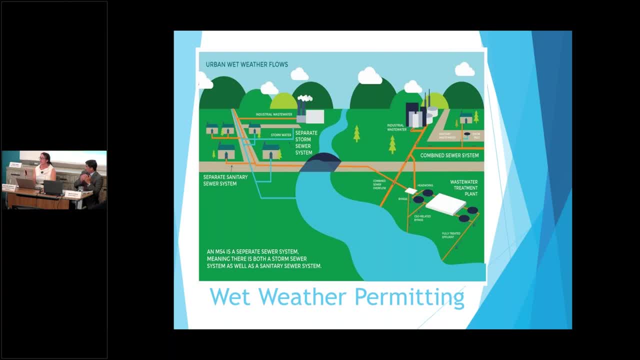 and it can cause a lot of damage. So what cities have done is they've constructed overflows. So what cities have done is they've constructed overflows And when it gets to a stop, it's like, oh, there's a stormwater. 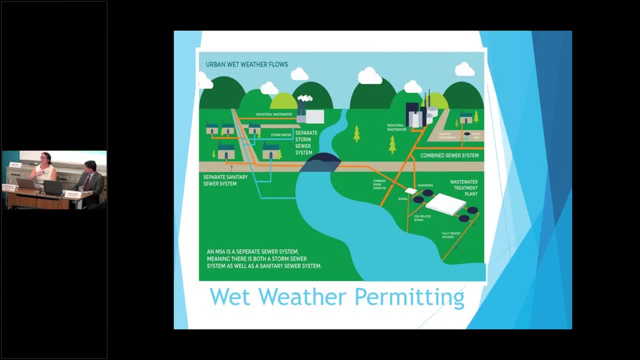 a certain level where the plant is going to receive too much flow, that gets diverted and it overflows into surface waters. it's a problem. there was a combined sewer overflow policy that was was enacted in 94. i think it's now actually ratified in the clean water act, so it's part of. 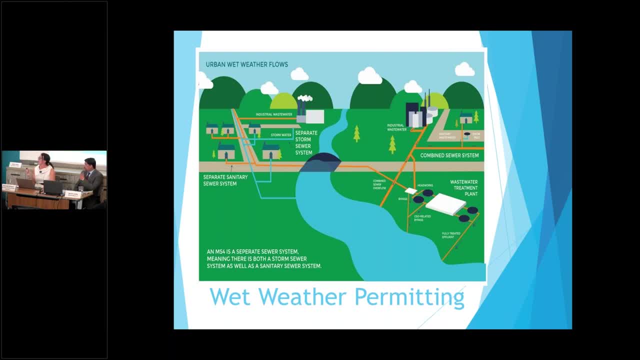 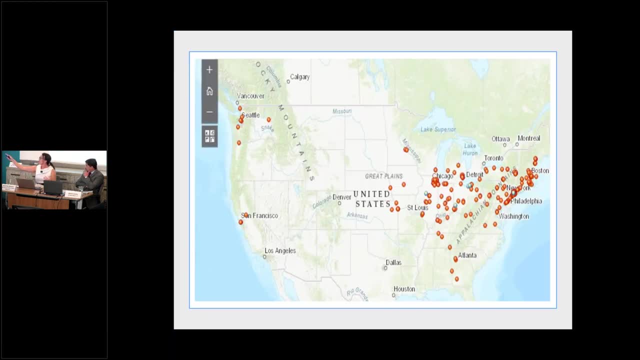 the clean water act, and so with those combined sewer overflow policies, you have consent decrees existing and here's a map of where you see uh. the bigger these are, the bigger- over 50 000 uh population, cso communities. what you have are consent decrees, so the policy envisions a good 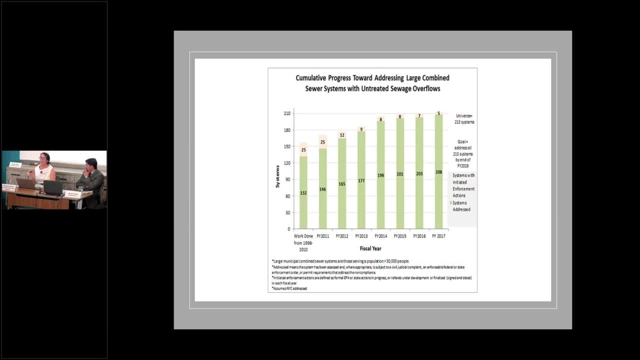 way to address these are consent decrees, because you can't just go out and in a year separate all the systems, and even separation is not now the um, the preferred method, because then your storm water is not getting any treatment. so a lot of things are being done and 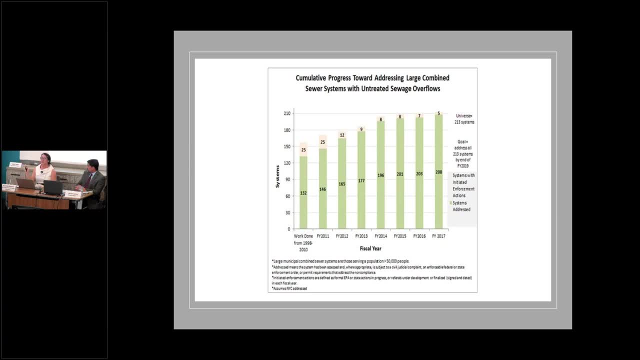 you can't just go out and in a year separate all the systems, and even separation is not now the preferred method, because then your storm water is not getting any treatment. so a lot of things are being done and you can't just go out and in a year separate all the systems, and even separation is 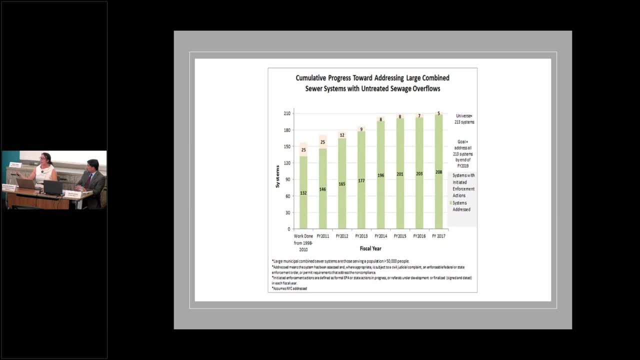 not now the preferred method, because then your storm water is not getting any treatment. so a lot, it's more. you know 20 years. we're now seeing 25 years to give time to, to implement these big capital projects, because the reality is for, uh, public utilities, it's you that pay. so how much? 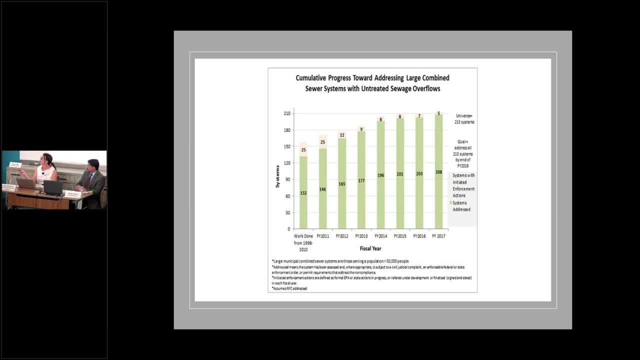 can the population bear in rate increases in order to fund these things? if you guys done a good job with their enforcement, you'll see here, of the um 213 systems that are for populations of 50 000 people or more, um that there are 208 that are under enforcement consent for your negotiations. 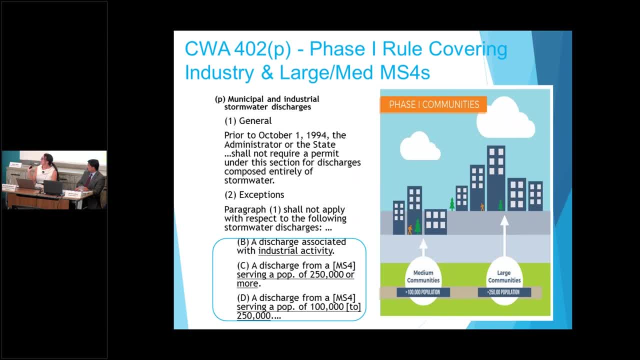 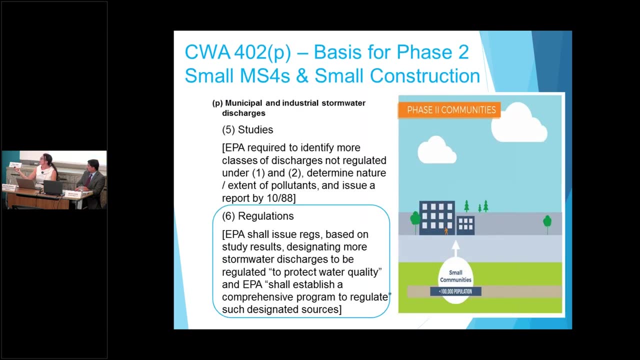 okay, so i am running out of time, let me run through these. this is the 87 amendment. this is where you have the uh phase. uh, large ms4s and industry come into the fold. uh, you can look these up in my slides. um, small construction came in. this was so. 1990 is when you had the phase one required to get permits. 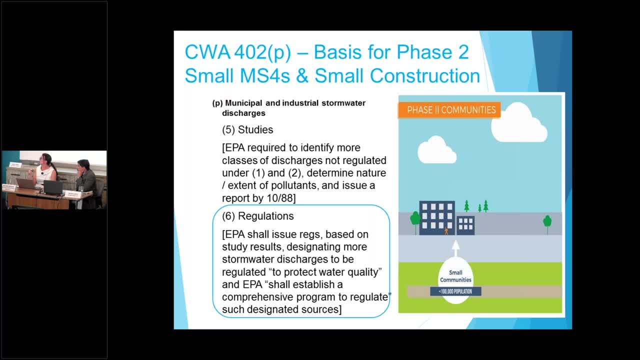 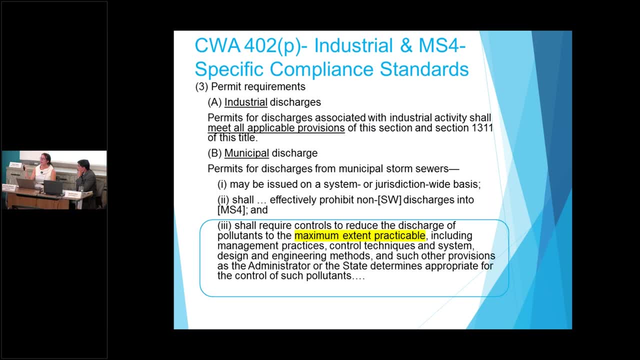 and it was 99 when you had the rule making for phase two. the it's appropriate, it's important to note out. for stormwater it's a different. it's a different standard. it's maximum extent, practical. normally cost does not come into play at all in the clean water act, but with this, 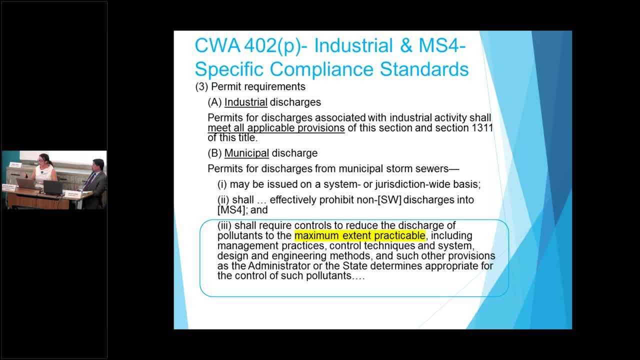 with this standard. it does um. so you have to do best management practices to the maximum extent, uh, practical uh, to achieve what you're going for, like you can. your goal may be water quality, but if you get to a point where you cannot spend any more as a community, then that's your. 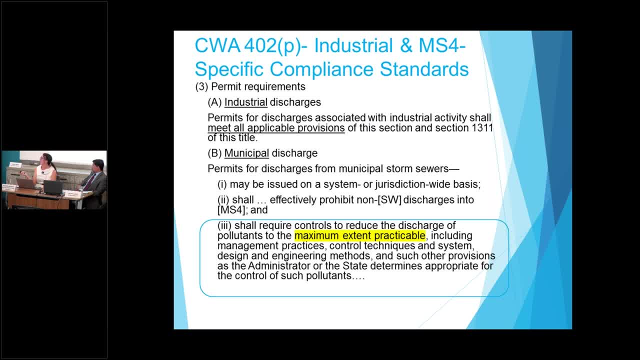 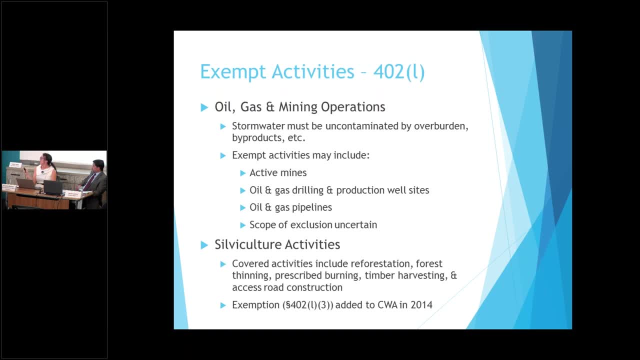 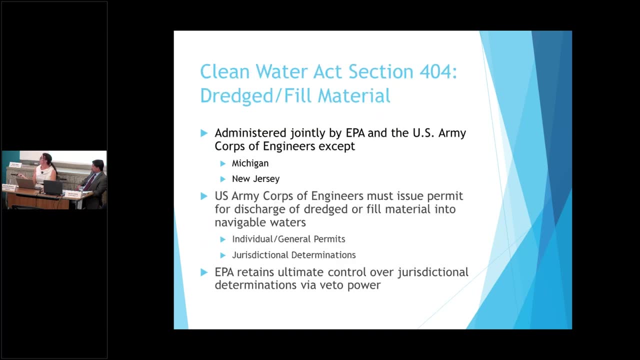 your mep, your maximum practical, so cost does come into play. uh, just, these are exemptions from this. uh, the stormwater permitting. uh, the silviculture is the forest example and that's the decor case and i can provide more information on that. uh, the 404 dredge and fill program. i think we've covered that. uh pretty well, there are two states. 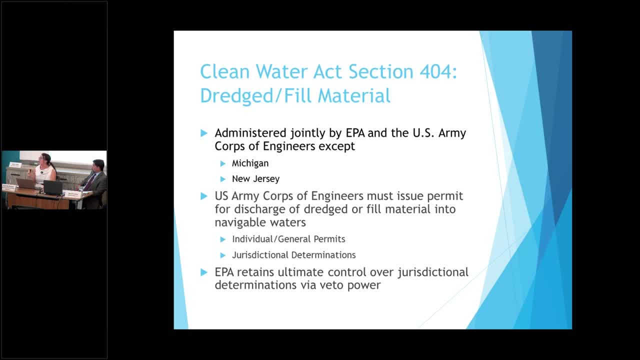 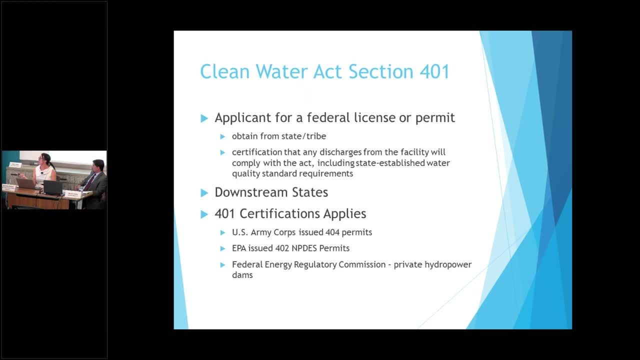 that have the ability to administer it: michigan and new jersey, um, and even though the corps is the main party for going out and doing uh jurisdictional determinations, uh, epa does have the ability to overrule that. and 401 we've covered. so that is all for me. 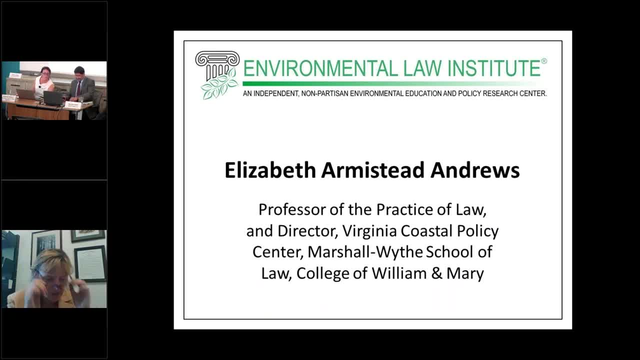 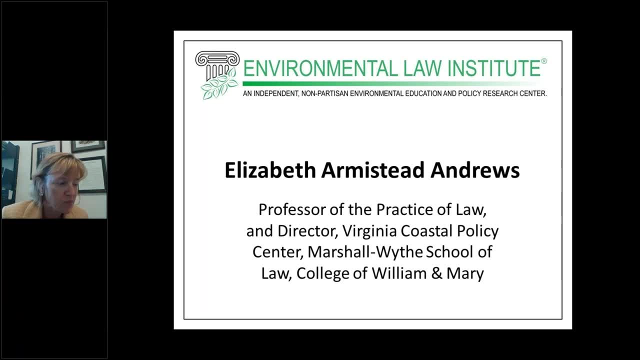 okay, this is elizabeth and i'm beaming in through the wonders of technology. um, i appreciate the opportunity here today and i'm totally impressed by my comrades who are able to cover this part of the conversation, but i've been surprised by how many of you have, uh, had a chance to participate and 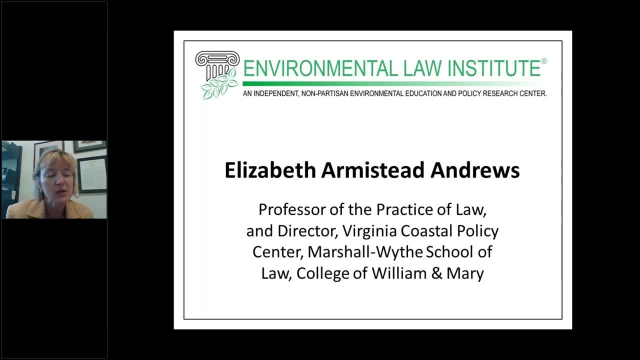 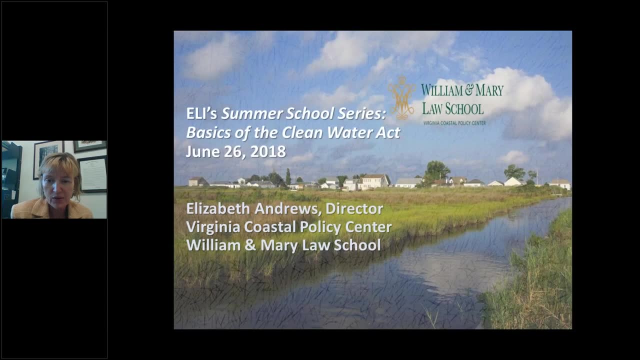 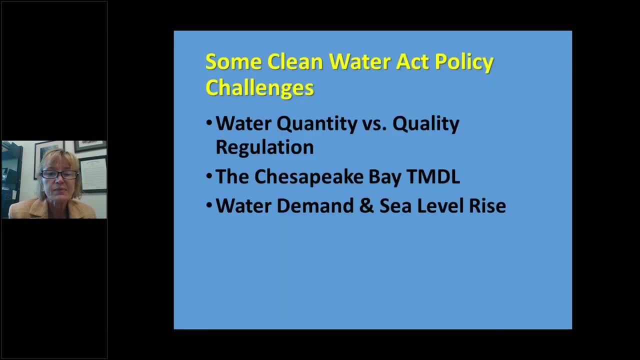 how many of you have uh had an opportunity to participate in this program? so thank you. or if you want to join um, we have some more questions that we have. um uh, up and yell at me in the middle if I'm going over my time, please, So just a few. 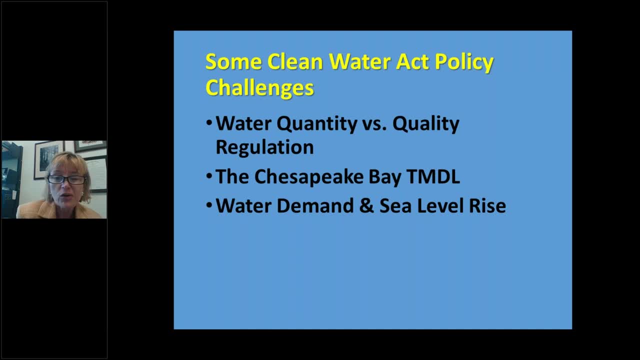 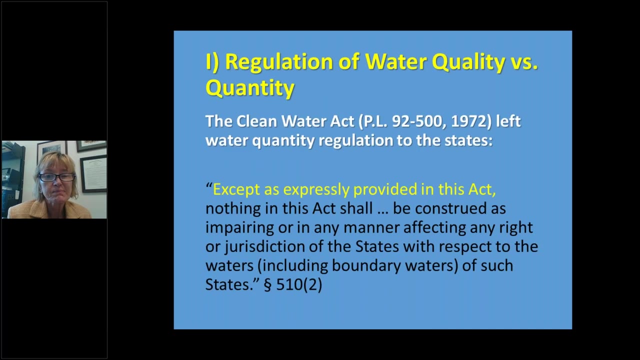 policy challenges that I'm going to cover: Regulation of water quantity versus water quality, which I believe Kathy touched on a little bit, Chesapeake Bay, TMDL that David mentioned and also Amanda, and then I was asked to talk about water demand and sea level rise or climate change. First of all, the Clean. 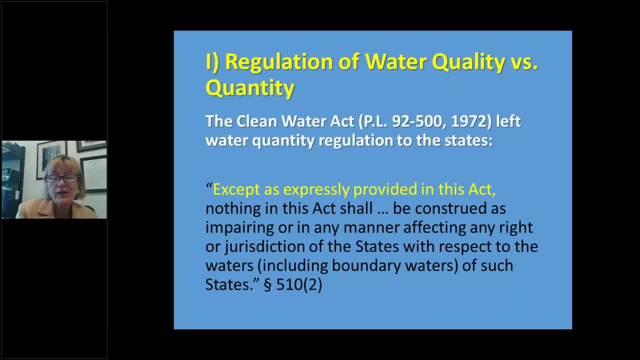 Water Act back when it was adopted 1972, largely and again this is the 30,000 foot view level that we're doing in this class. So, in general, left water quantity regulation to the states, and this is a provision I think Kathy might have. 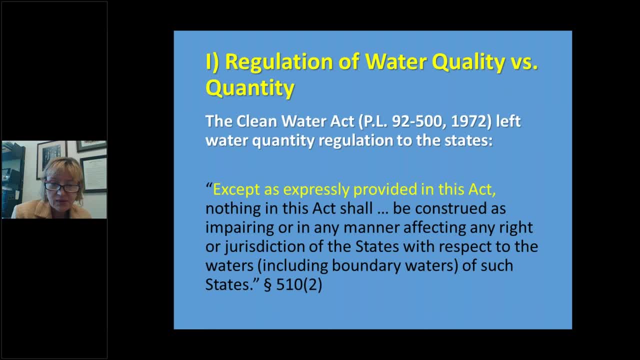 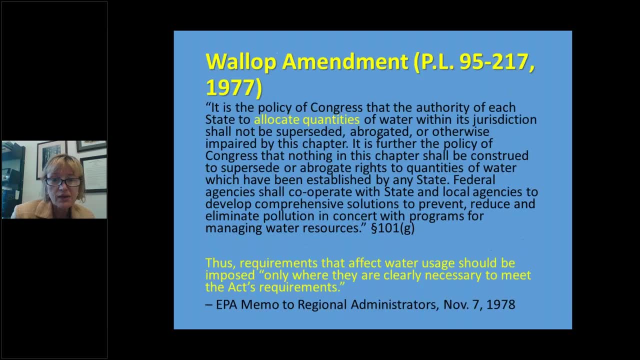 flashed up on the screen already. except as expressly provided this act, Nothing shall be construed as impairing or in any manner affecting any right or jurisdiction the states with respect to the waters of such state. And again, the wallop amendment that she mentioned in 1977.. Policy of Congress. 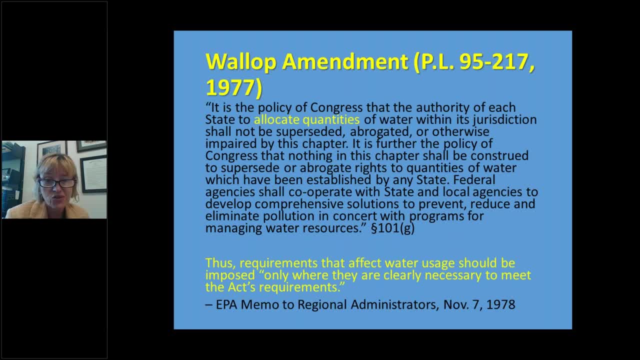 authority of each state to allocate quantities of water within its jurisdiction shall not be superseded, abrogated or otherwise impaired by this chapter. And then there was an EPA memo that came out after that- Interestingly enough, I think I saw Kathy added that to your presentation as well- saying that: 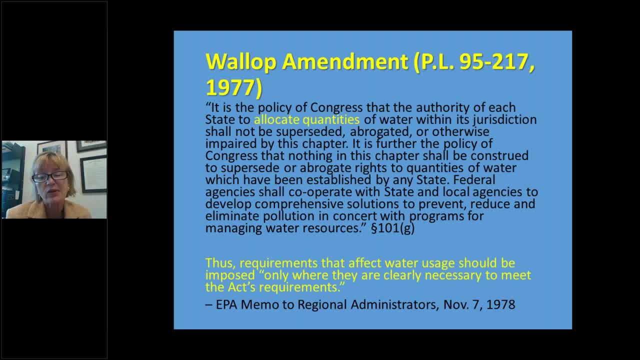 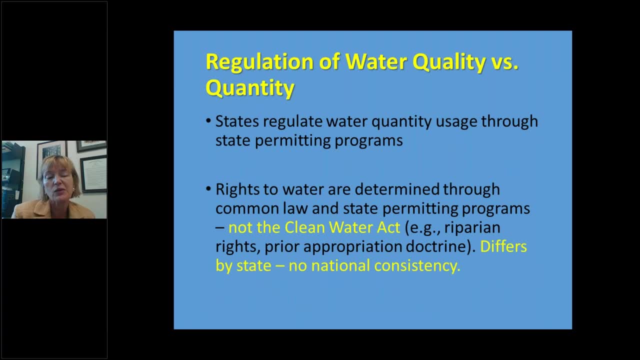 requirements that affect water usage should be imposed only where they are clearly necessary to meet the Act's requirements. So that's the general construct and, as David mentioned, the Clean Water Act in general is dealing with surface water, not groundwater. It's in general dealing with water quality versus quantity. States do regulate water. 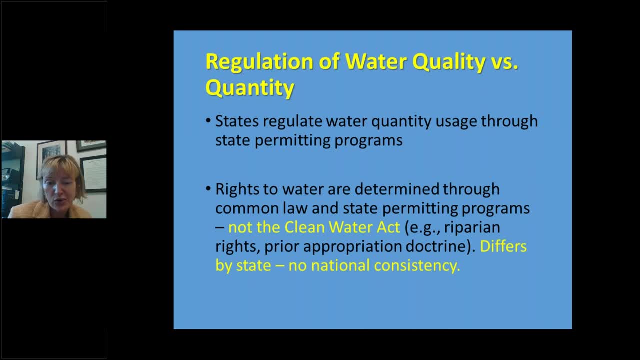 quantity through a variety of different, through their common law and through their state permitting programs, A variety of doctrines, whether it's riparian rights or prior appropriation, depending on where you are in the United States and what the doctrine is. So there's not the national consistency. 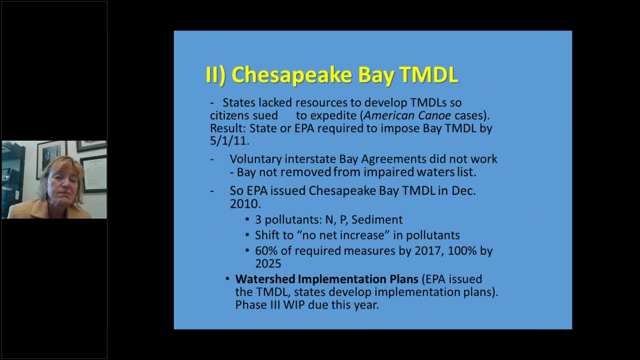 that is set by the water quality rules. It just be made. TMBL is actually an excellent example of how regulation of the Clean Water Act has to be a creative process, A flexible process and an iterative process at times, because the Chesapeake Bay TMDL. 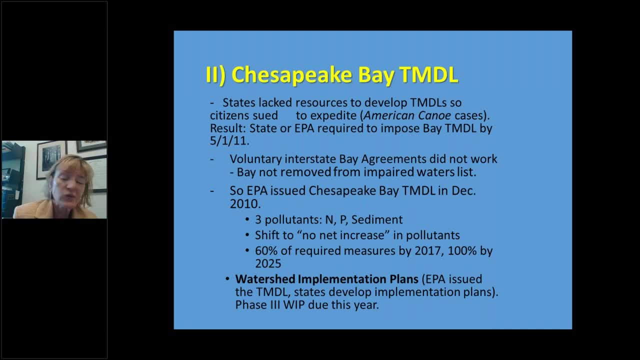 involves numerous States and you have to bring everyone to the table and get them to agree on the requirements that are going to be imposed to achieve water quality standards for the Chesapeake Bay TMDL, Many tributaries and all many different governmental layers involved. So to give you a brief history of how it, 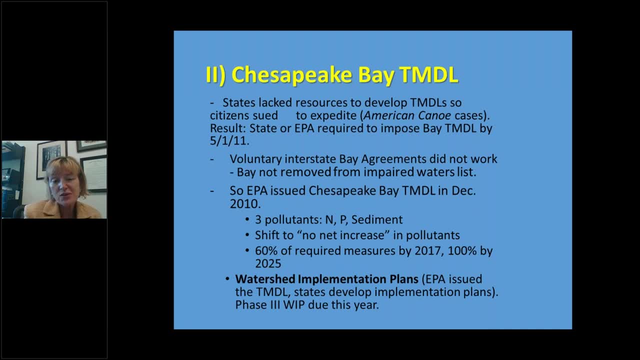 came about, the state's essentially lacked the resources and sometimes the political will to develop TMDL. so to give you a brief history of how it came about, the state's essentially black: the resources and sometimes the political will to develop TMDL. They lacked the resources and sometimes the political will to develop TMDLs back early. 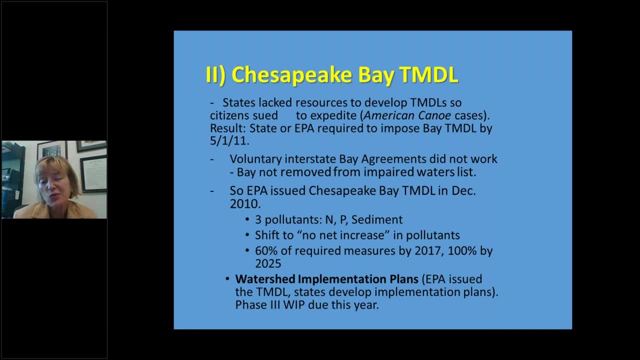 on. So there was a series of court cases brought the American Community Association cases, because there was a feeling there had been a lack of sufficient progress on restoration And it led to these numerous lawsuits against the EPA for failure to develop TMDLs and 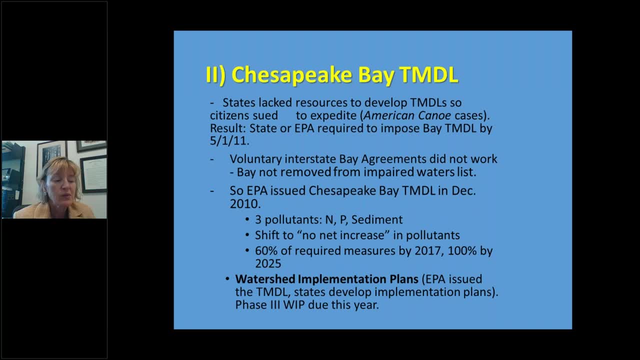 the cases were settled pursuant to consent decrees from the EPA and generally required the EPA to develop TMDLs for the Bay segments by 2011,. if the state had not done so by then- It was in Virginia's case, for example- the consent decree set out a TMDL development. 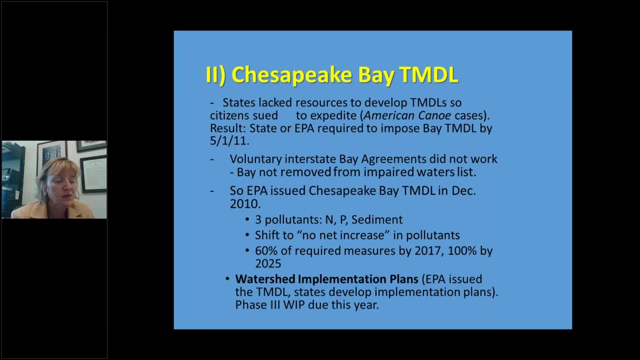 schedule that went through 2010 for the state to meet. The states also tried to engage in a series of voluntary agreements- Chesapeake Bay agreements- to try to clean up the water body. Everybody around in the Bay states knew that the Chesapeake Bay needed to be protected. 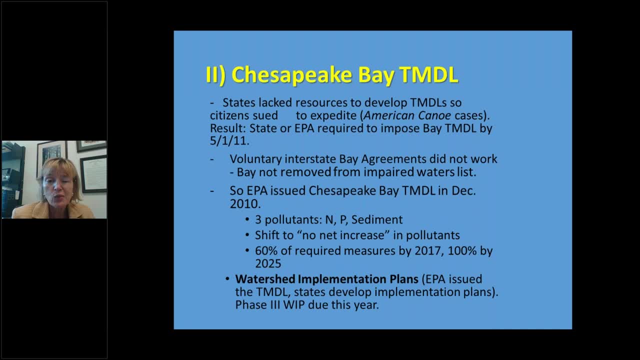 and cleaned up. but how to get there, And especially with a voluntary agreement, was subject to discussion, and the result was the Bay was not removed from the impaired waters list through those voluntary agreements alone. Just to give you an indication, there was a 1983 Bay agreement that first set up the 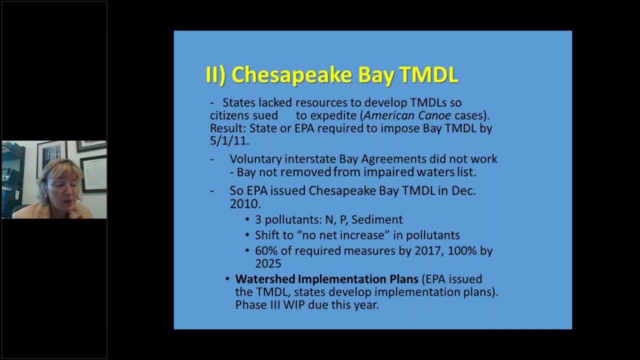 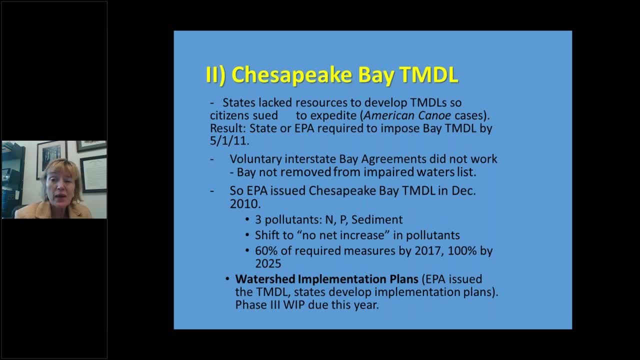 And the Chesapeake Bay agreement, as it was called. it called for states to act to remove the Bay and its tributaries from the impaired waters list by 2010.. There was a big call at the time to achieve that, and the headwater states were included. 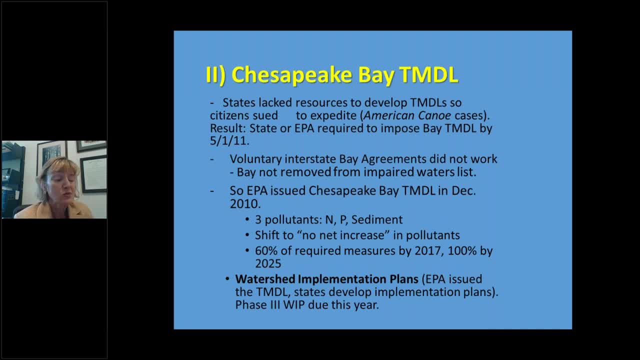 on the Chesapeake Executive Council And also in 2000,, Congress did amend the Clean Water Act- Section 117, to achieve the goals established in the Chesapeake Bay agreement and clarifying EPA's role in the process. the Chesapeake Bay program's what they call their principal staff committee. 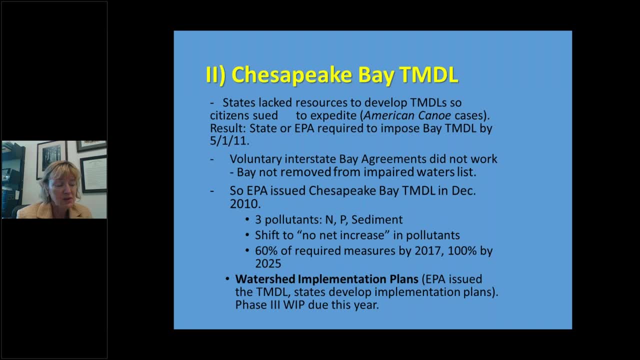 requested that EPA develop the TMDL, It was clear that things weren't working as well as they should and by 2010 it was clear the goals would not be met. So by 2008, Chesapeake Bay program recognized the 2010 goal would not be met and the 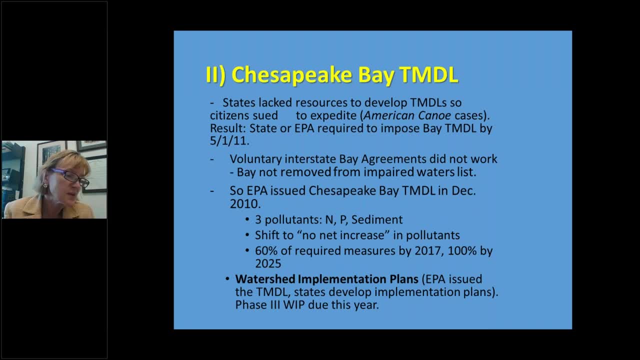 TMDL process began. So it's different from the framework for point source permitting that Amanda just went through so well, because it does have so many different governmental entities involved and it does have a difference, a different standard that people talk about in a way, you know, under the point. 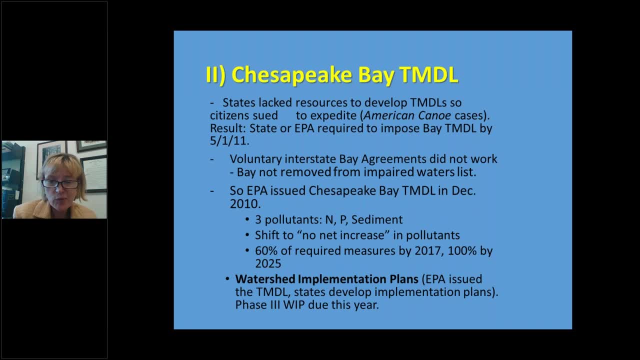 source permitting. that was just covered. it's about getting your permit and you're issuing pollutants to a certain extent as allowed by your permit. Here there's a lot of discussion under the Chesapeake Bay TMDL that there is to be no net increase in pollutants, So it's a slightly different approach, trying to improve the. 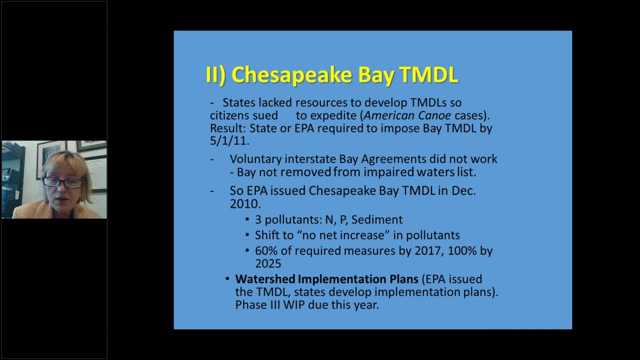 water quality. Three pollutants are at issue: nitrogen, phosphorus and sediment. The states are required to have in place 60% of the required measures by 2017 and 100% by 2025.. It's important to note that doesn't mean that all of the reductions. 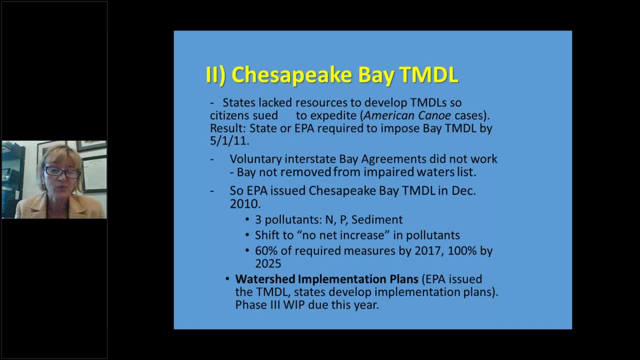 that are required by the Chesapeake Bay TMDL have to be achieved by 2025, but the measures have to be in place to achieve that- The going back to the Cooperative Federalism approach that was just talked about by a number of the panelists. the EPA issued the TMDL but left it to the states to develop their 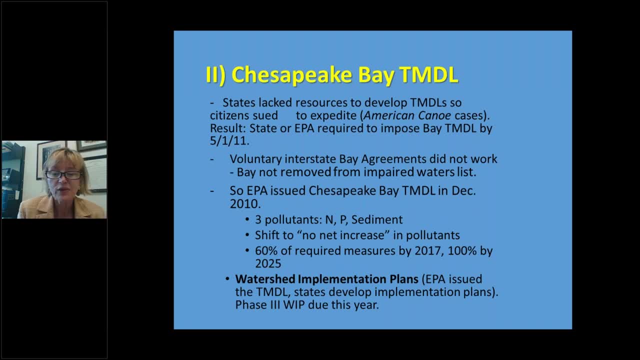 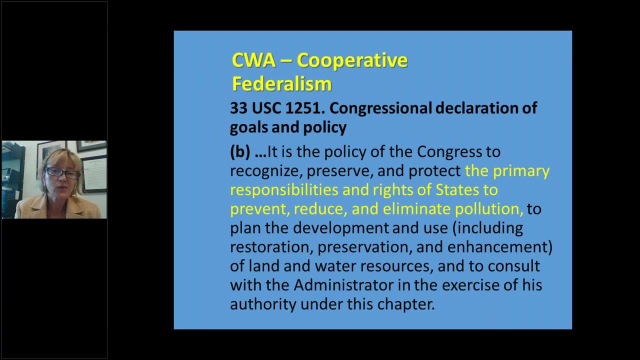 own watershed implementation plans, and so we've had two iterations of that. We're now working on the Phase 3 WIP this year, and again, here we go with a Clean Water Act and the Cooperative Federalism that it's a policy of Congress to recognize. 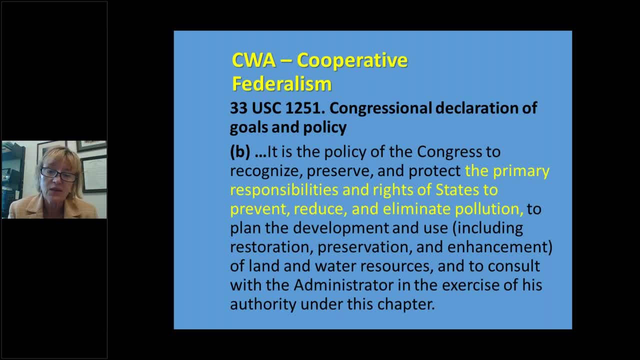 preserve and protect the primary responsibilities and rights of states to prevent, reduce and eliminate pollution. and a number of steps have been needed. You know now they are being flushed by the Delegates: Ken Davenport Council andaminates from Almost 100 to around 65. They are commercially that the schedules that act and North America posed problems Very e hineな. 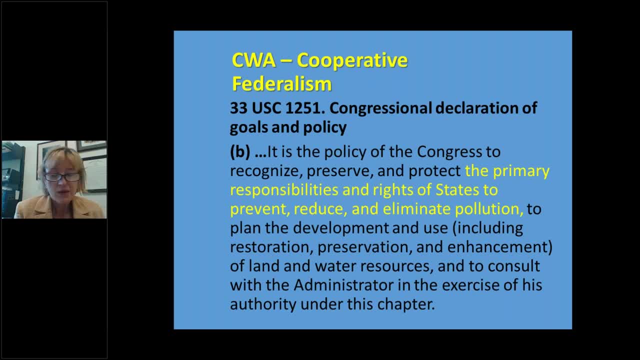 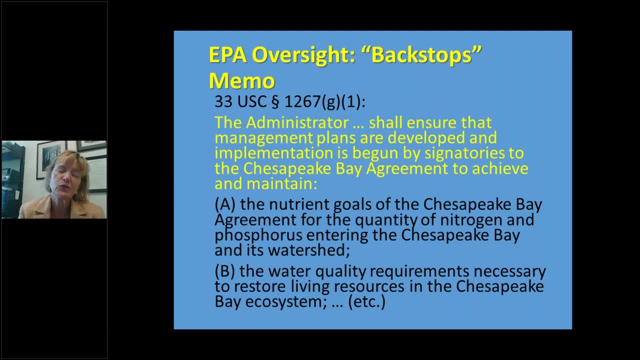 etc. etc. so how do you achieve this when you have multiple states involved? how do you enforce that? what the EPA did was they issued something that we call the backstops memo, saying to the states: we have to have reasonable assurance that your measures you're putting in place, that you're developing it through your 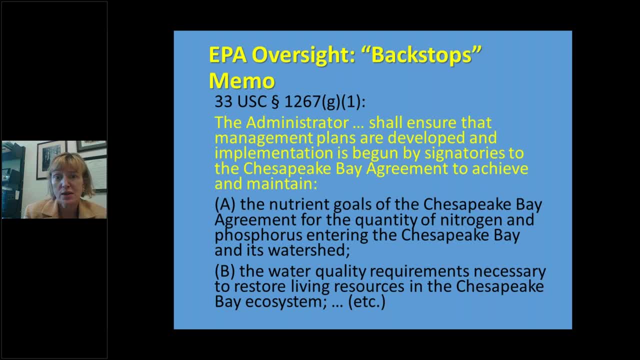 watershed implementation plan will actually achieve water quality standards and will protect the water quality of the bay. and so, to achieve that, we're going to have you submit the watershed implementation plans to us for approval, and if you don't do a good job on those, if you don't put enough protections in 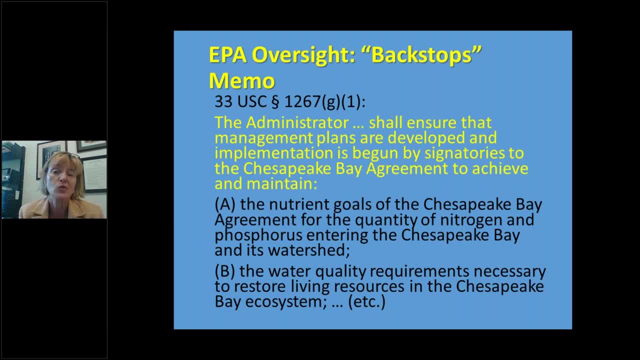 place and propose enough measures to be taken to improve the water quality sufficiently to comply with the TMDL. then we have some backstop measures that we can implement and this is some of the authority that decided for that that the administrator of the EPA shall ensure that. 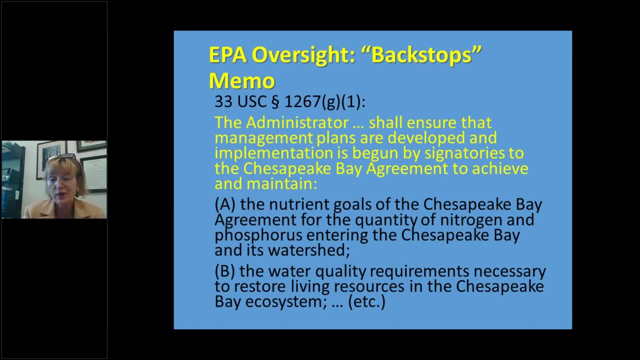 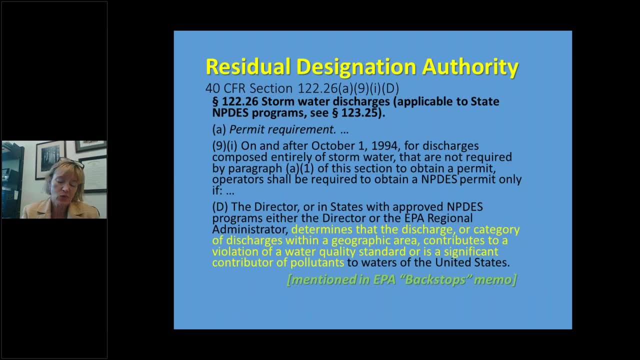 management plans are developed and implemented. implementation has begun by signatories to the Bay agreement and it's in. one of the things that they mentioned in the memo is that they could increase enforcement for existing permittees. they could increase requirements for point source permittees. they could reduce grant funding from the EPA to the states, which is very 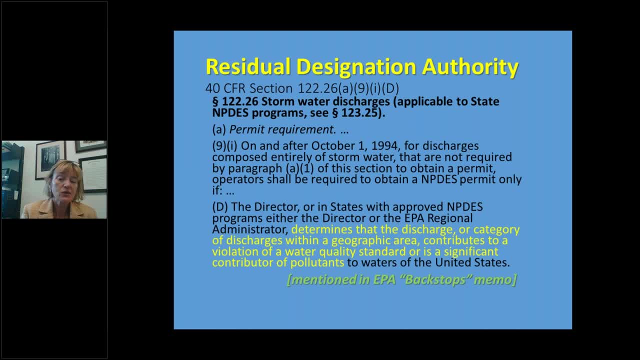 important funding for the programs the states have. and another is that they might exercise what's called resilience designation authority, and this is an interesting provision, I think, David- I don't recall you covering this in your presentation, but it is. it's a part of the Clean Water Act. the enforcement that they can do is that they can if they. 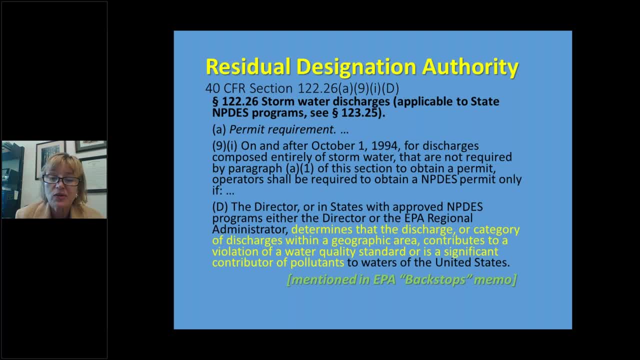 determine that a discharge or category discharges within a certain geographic area contributes to a violation of a water quality standard or is a significant contributor pollutants to waters in the United States, then they can require a permit and then enforce under that. so that is a way to get to. 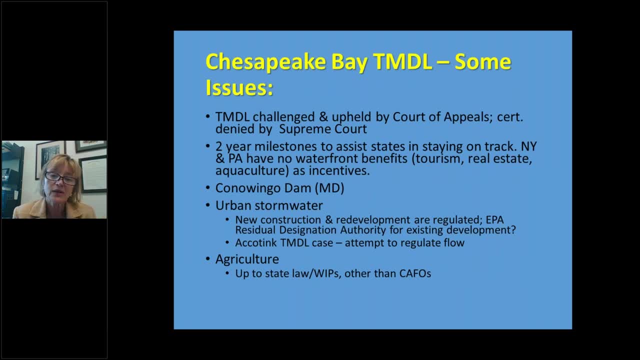 pre-existing development and try to get control over their their discharges of pollutants. so some of the issues with the Bay TMDL, some of the big policy issues: again, you have to be creative and you have to be flexible in this iterative program in order to have it change for the different challenges that come down. 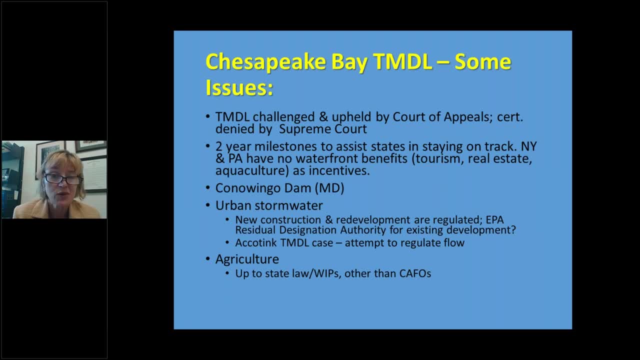 the as you're implementing this huge TMDL process. the TMDL was challenged- I- amanda talked about that a bit- and David- and upheld by the Third Circuit Court of Appeals. I did send into Eli. I think they're going to make available both the district court and the Court of Appeals decisions. as David said, it's. 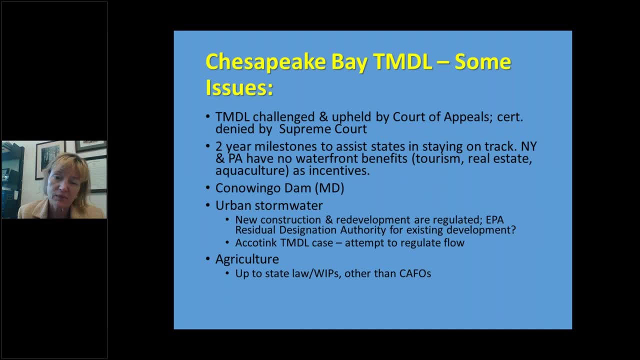 interesting reading for those of you who are seeking summer beach time reading. it's. it's a good. it's a good opinion, setting forth a lot of the background material that might be helpful to you. and then the Supreme Court declined to hear the case. there were a number of different concerns with the people that brought the. 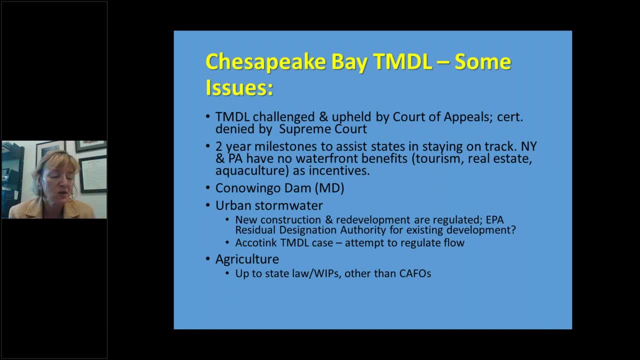 case was brought by the American Farm Bureau and American Home Builders Association at all and they were concerned about what they saw as EPA overreach into the realm of what the state should be doing. but also there was concern about precedent, because this is again an interstate effort and if it is, 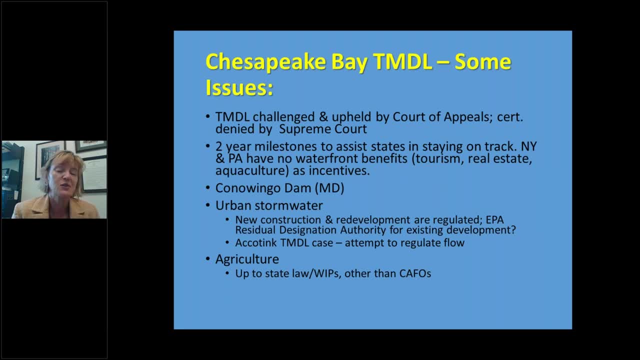 upheld by the courts for the Chesapeake Bay. it could be used for the Mississippi River and other water bodies. so the trial judge did say that the Bay TMDL is within the EPA's Clean Water Act Authority and it was not arbitrary or capricious and was. 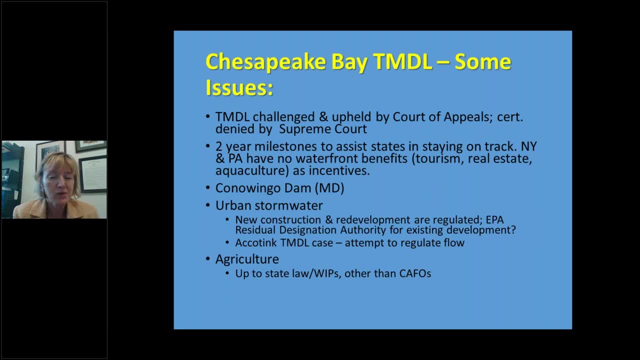 subjected to appropriate public notice and the appellate court agreed. the three judge panel agreed. so there are two-year milestones in place under the Bay TMDL to help the states, because it is a long time out to 2025 to make sure the states are staying on track and 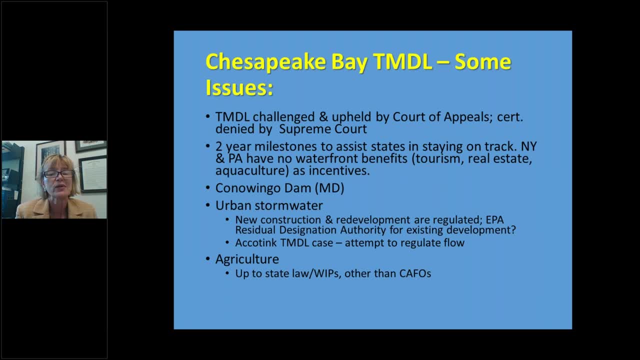 We did a midpoint review where the EPA came in and assessed how each state was doing. One thing that's interesting to note is going back to flexibility and creativity. headwater states such as New York and Pennsylvania have no waterfront benefits on the bay. 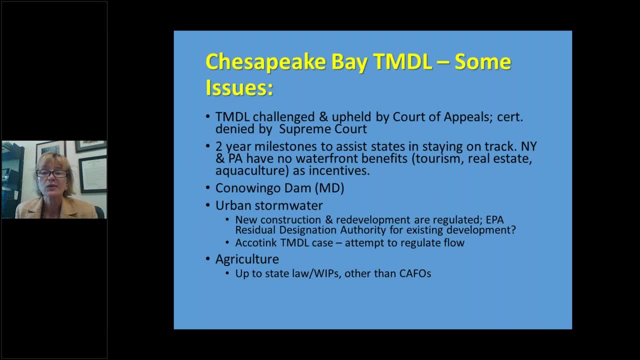 They have the Susquehanna River coming down, but they don't have the tourism and the real estate values and the aquaculture generated by being on the Chesapeake Bay itself, And so you're asking them to spend dollars and clean up the water quality for people. 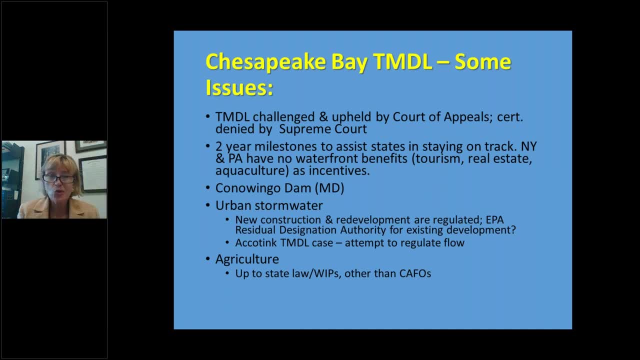 downstream, And that's just a reality of the process. Again, the joy of having a multi-state process in place is trying to keep everyone at the table and discussing how to achieve this when it's getting it's going to get more and more. 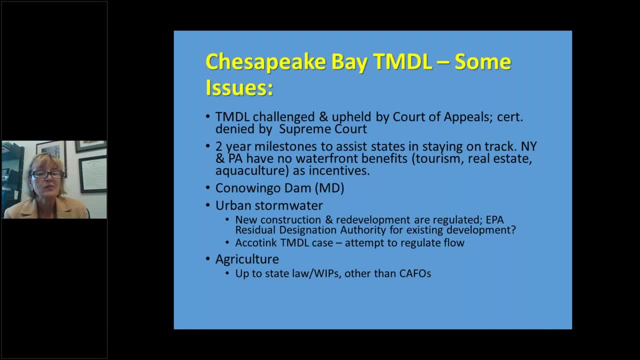 costly as we go along The Conowingo Dam. actually for years people didn't realize it was serving as essentially a large sediment trap for the Chesapeake Bay, And it's now no longer doing that, And so we're trying to figure out among the bay states how to deal with that increased 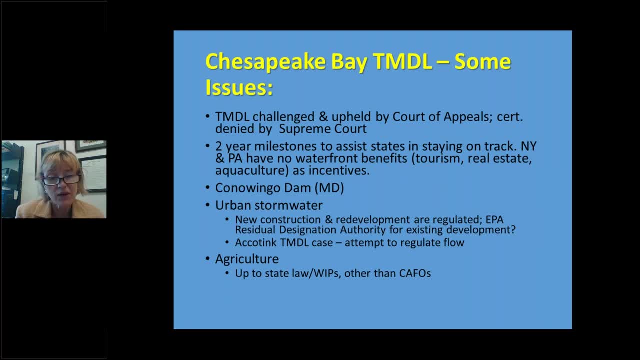 pollutant load, sediment and nitrogen and phosphorus from that. So again, that requires flexibility And the Bay Program is a multi-state effort, with work groups assigned to different topics, with state representatives from all the different bay states coming to agreement on how best. 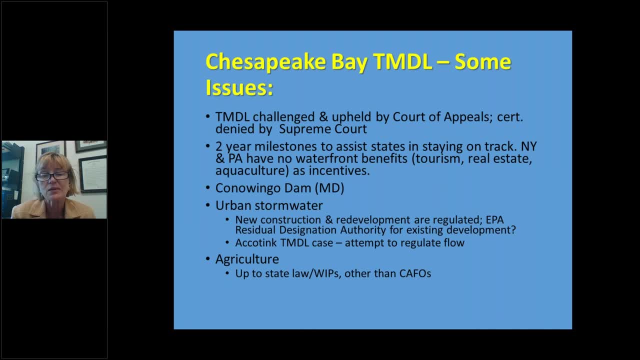 to approach these challenges. Urban stormwater- There's a big one. Back in 1972, it wasn't as big an issue as it is today. We have more and more impervious cover. When we talk about impervious cover in stormwater world, what we mean by that is rooftops and 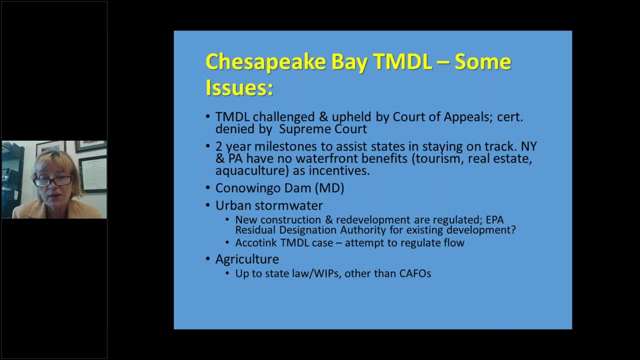 decks and parking lots that are impervious, so the water doesn't filter through, It sheds off and it creates runoff with greater volume. And so what do we do about that? Because, as Amanda mentioned, we have construction And Construction general permits that deal with the larger construction sites and redevelopment. 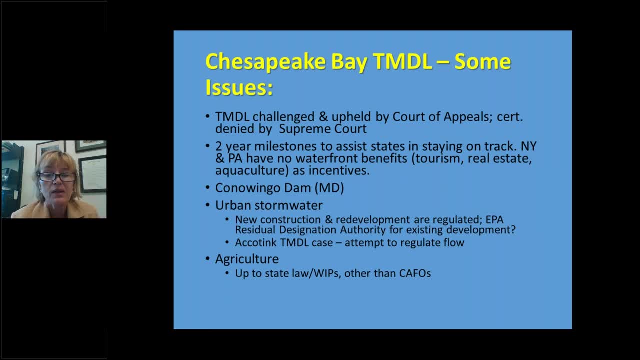 sites. But what about the prior existing development that you can't go back. You don't have the authority to force retrofit. There was an example of a TMDL case on the tributary of Akatink Creek and up in Northern Virginia. 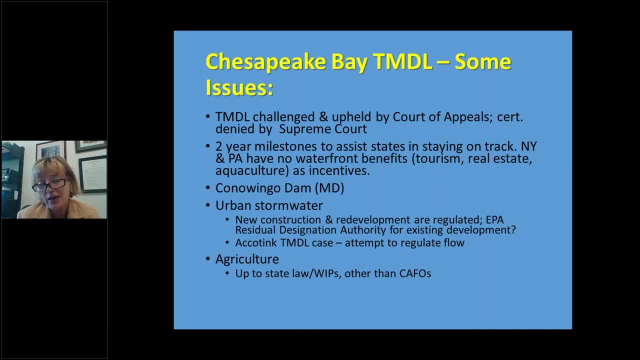 It was a case the Virginia Department of Transportation and Fairfax County and urbanized County in Northern Virginia Challenged a TMDL that had been issued by the EPA was attempt to regulate the flow of water itself, because the water volume is what was damaging the stream and generating the 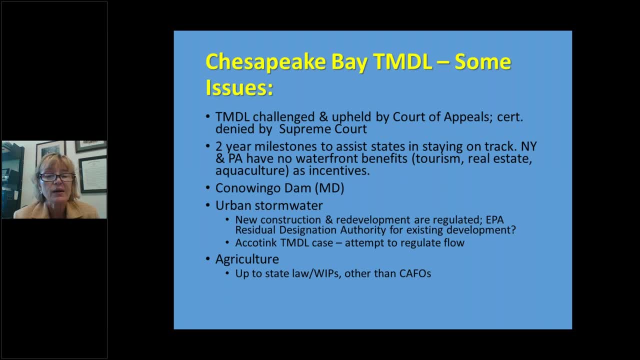 sediment in stream as it turned up the bottom of the stream And the court overturned that and sent it back to, remanded it back to, and they're actually having an effort underway in Northern Virginia to think about how to address the pollutants in the Akatink now because it's a real dilemma. 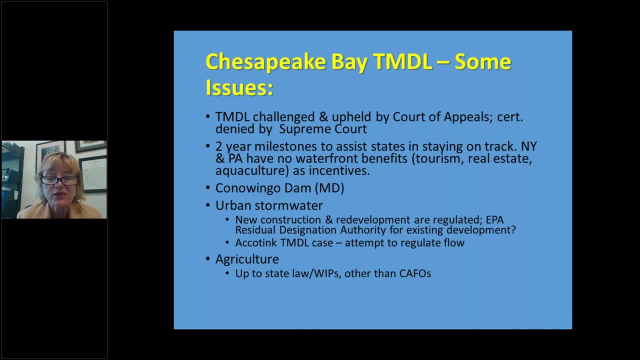 What do you do? What do you do when the water volume itself is causing damage? That residual designation authority that I talked about a minute ago is one way to get to that, possibly by some of the larger sites that are generating a lot of runoff. 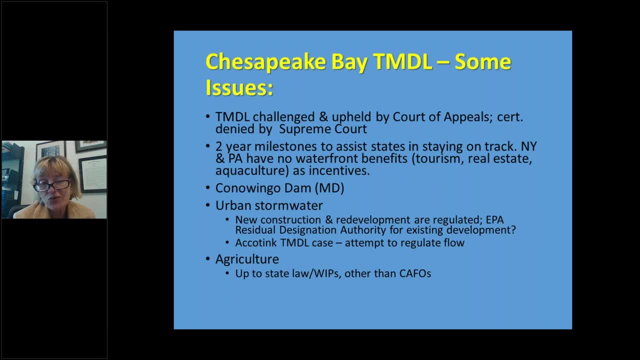 That's something that in the future could be attempted. or there's also stream bed restoration projects that are important to create the ability for streams to absorb more of a volume of water, But of course those are quite expensive as well. And then agriculture is another challenge. 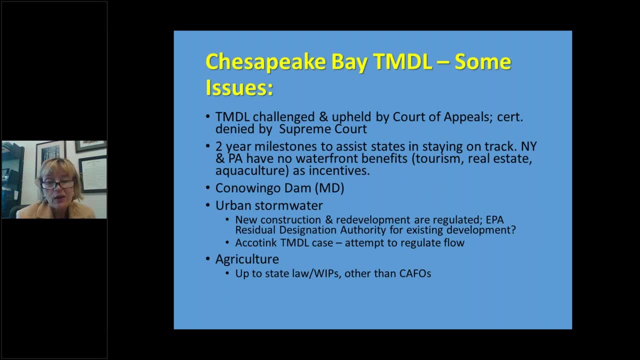 I think Amanda mentioned that CAFOs, Of course- that's a big issue- Of course- are permitted, But, on the whole, dealing with agriculture is something that has been left to the states through their whips, their watershed implementation plans. 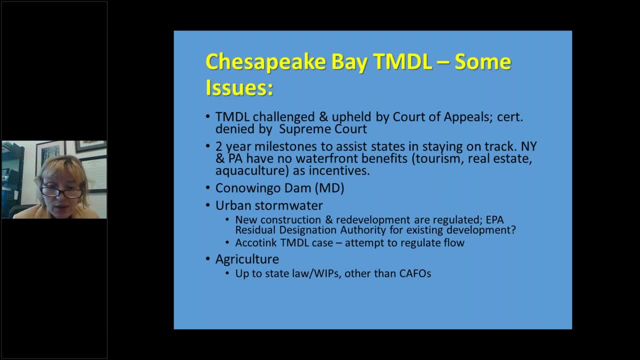 And that, of course, is dependent upon, frankly, a lot of times, political will and what the states are willing to do to do that. Adjusting the modeling for the Bay TMDL based on projected growth and therefore increased pollutant discharge, and on climate change is another challenge. 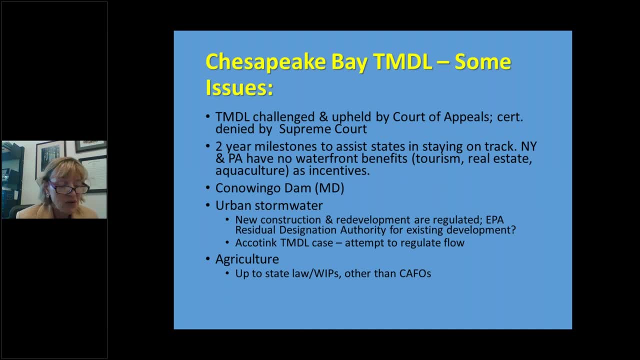 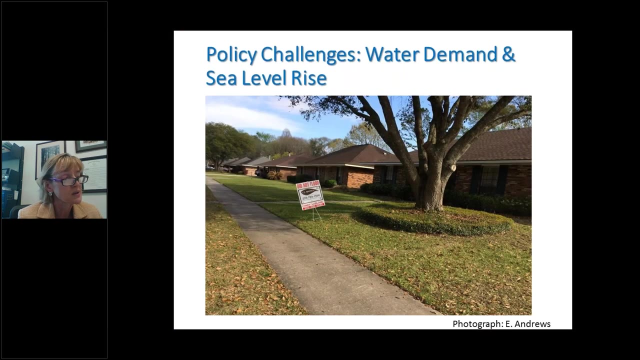 States have agreed. the Bay states have agreed that they're going to try to do narrative strategies at this point and committing to adopt climate change targets later on. No actual numbers until after 2021 and the Bay model will be updated and then states will update their whips, their watershed implementation plans. 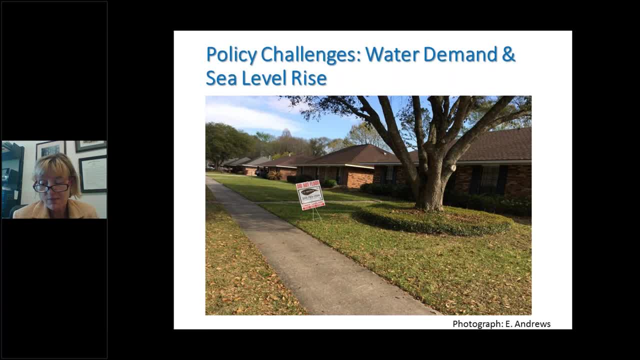 This is a picture that I took down in Louisiana. actually it's sad, but that's how it's advertised now If a home has not been flooded. The increased need For water and sea level rise and its impacts also pose some policy challenges. 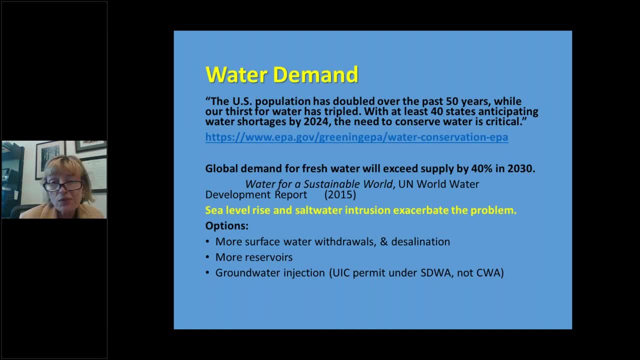 Just to show you off the EPA's website itself: the US population is doubled. Our thirst for water is tripled. At least 40 states are anticipating water shortages by 2024.. So obviously water demand is important, And the UN came out with a report estimating the global demand for fresh water will exceed. 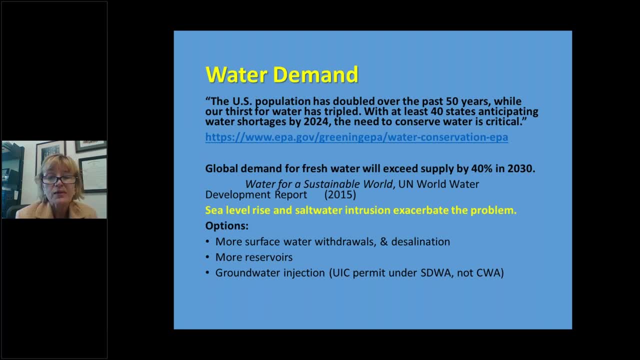 supply by 40% in 2030.. And sea level rise and saltwater intrusion into our water supply, It only exacerbates that problem. So we can create more service water withdrawals and engage in desalination efforts, which can be expensive. 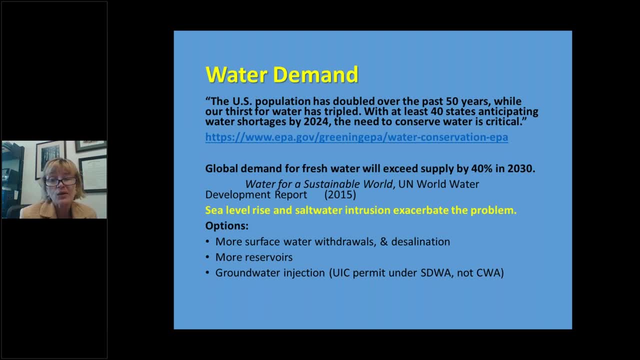 Build more reservoirs or do groundwater injection projects, which actually calls for UIC permit under the Safe Drinking Water Act, a separate kind of permitting system than the Clean Water Act. But we have an important project in Virginia that's been proposed: the SWIFT project. 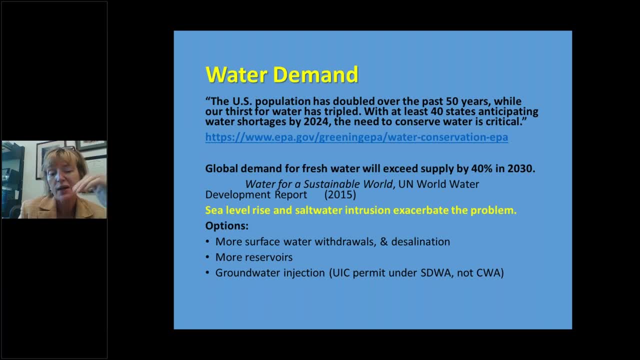 sustainable water initiative for tomorrow. that would take treated wastewater and inject it into the groundwater. Not only would that push the water pressure so that it holds back the saltwater intrusion, but it also would inject some pollutants into the groundwater aquifer. that would have gone. 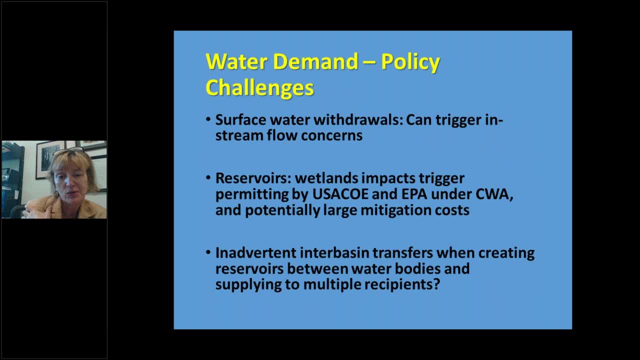 into the Chesapeake Bay otherwise, And so now people are talking about that as a way to achieve Bay TMDL requirements as well. Lots of nuances with the Bay TMDL and water quality regulation. So surface water withdrawals: if you do it too much from a particular stream, it can. 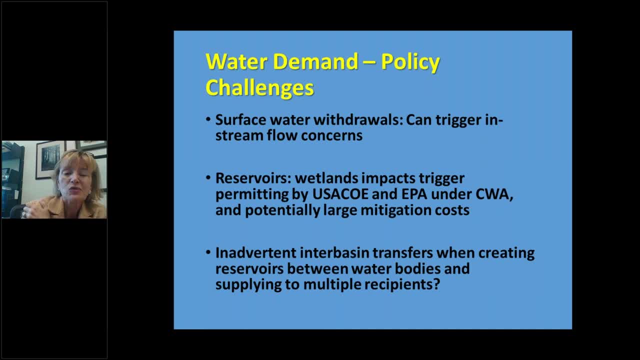 trigger in-stream flow concerns and water quality standard concerns, and reservoirs can trigger wetlands impacting which wetlands permitting I mean, which Amanda just covered, And also inner basin transfers. I won't go into that with this timeframe, but it's something. 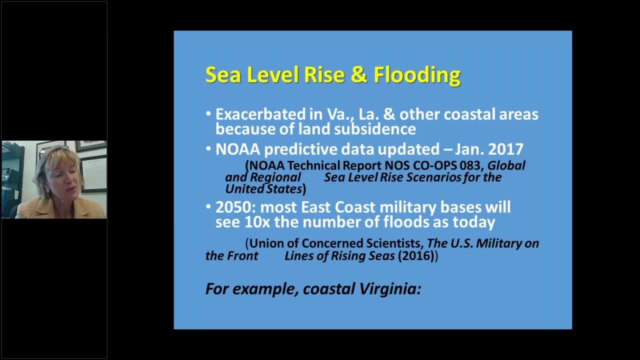 that also can trigger concerns when you're dealing between water bodies. So, when it comes to sea level rise and flooding, we talk in terms of relative sea level rise in areas like Virginia and Louisiana, where there is significant land subsiding, And so it exacerbates the impacts of that. 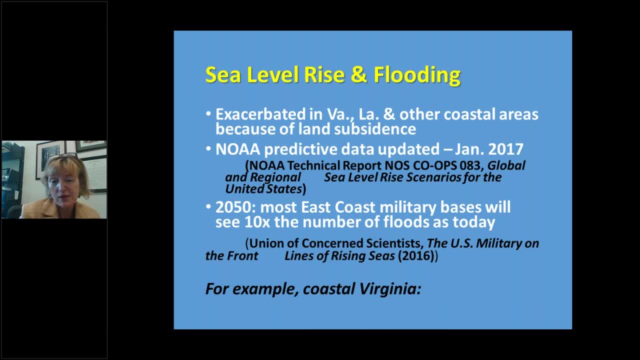 And NOAA tracks and has predictive data that it's come out with just in January of last year, talking about various sea level rise scenarios. The Union of Concerned Scientists has come out with a report- in fact they just came out with one, I think it was last week- talking about properties that will be underwater because 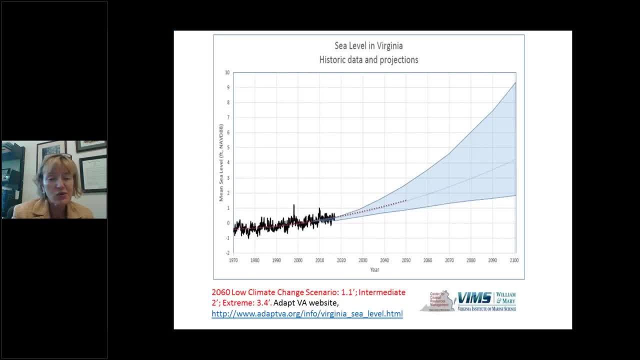 of sea level rise, So it is a serious issue, For example, in coastal Virginia. this cone of blue is to show you the prediction of water restriction out of the band of possible sea level rise scenarios based on actual observed data from 1970 through 2016 at Sewell's Point in Norfolk, Virginia. 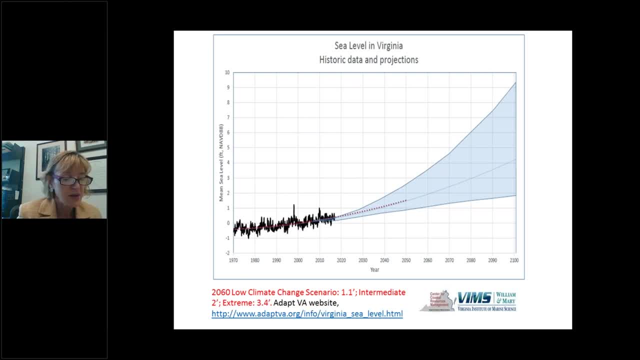 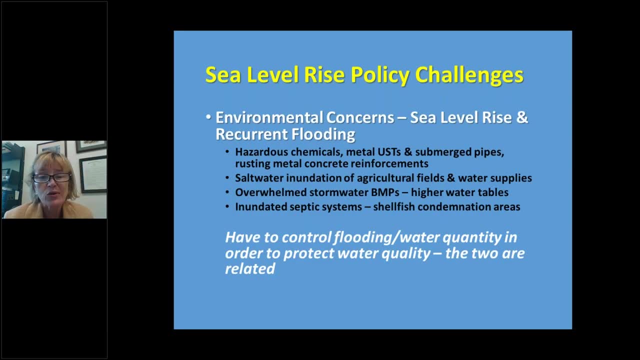 They took those observed values and projected out 40 years into the future and adjusted it to include land subsidence And, as you can see, it can be a serious issue And that's going to pose all kinds of water quality concerns that people may or may not. 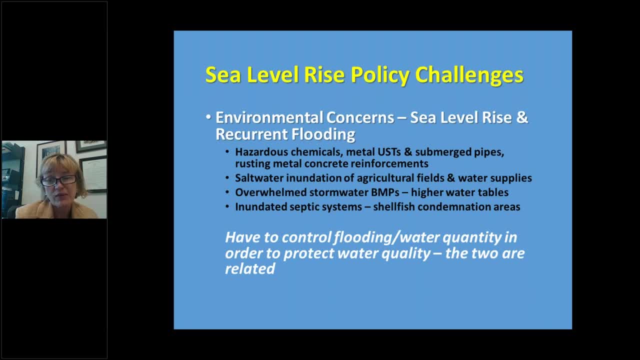 think about. that can be regulated under the Clean Water Act if need be, but it's going to take again flexibility and creativity. Hazardous chemicals, underground storage tanks, metal underground storage tanks and submerged pipes, and rusting metal. concrete reinforcements- the metal reinforcements that are in within. 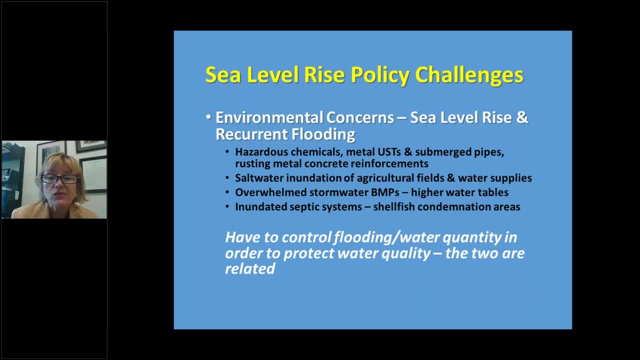 the concrete of bridges and highways. all of those don't do well when exposed to saltwater, flooding, Saltwater inundation of our agricultural fields and water supplies, our stormwater best management practices when they're in high water table areas. As that water table increases and the flooding increases, you can overwhelm your stormwater. 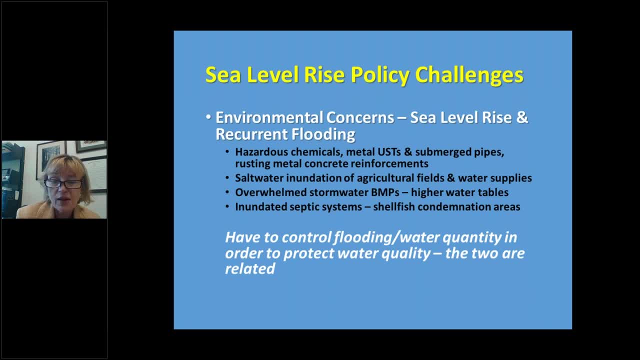 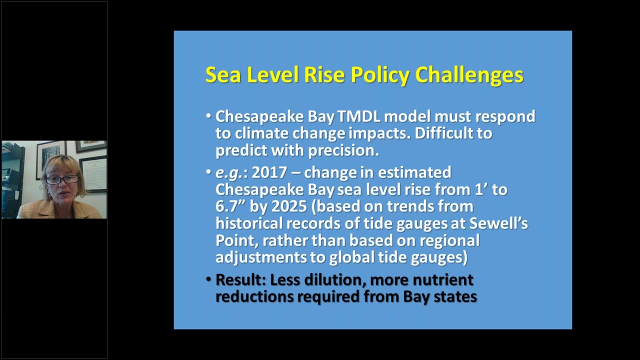 BMPs and you can have inundated septic systems and you can have areas for shellfish that are condemned because of the E coli. So there are a number of water quality concerns keyed into water quantity, impacts of sea level rise and flooding. So here's to give you a very specific example about climate change. 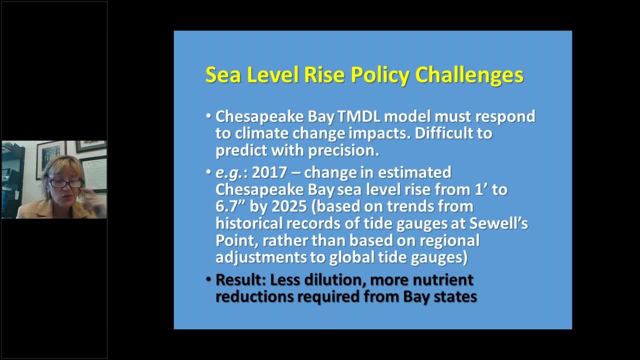 We have to constantly revisit the Bay Model to figure out if it's appropriately and sufficiently reflecting the changing conditions, because it's not static in the Bay and the water quality and the inputs to it, So it's difficult to predict the position, And an example of that is in 2017, there was a change that the program agreed to in the 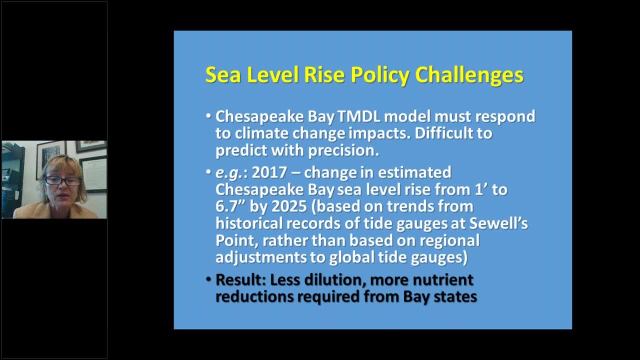 estimated sea level rise for the Bay And that was in 2017.. And that's because they realized they'd been looking at regional adjustments to global tide gauge data And they realized it would be more specific and accurate to look at trends from that Sewell's. 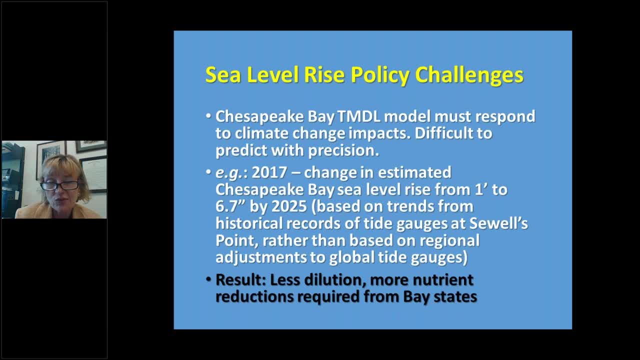 Point tide gauge in Norfolk that I just mentioned with that graph, And so we had to adjust and the amount of sea level rise anticipated And the result is less dilution, more nutrient reductions required from the base states. So it can have serious impacts on the requirements that are being implemented. 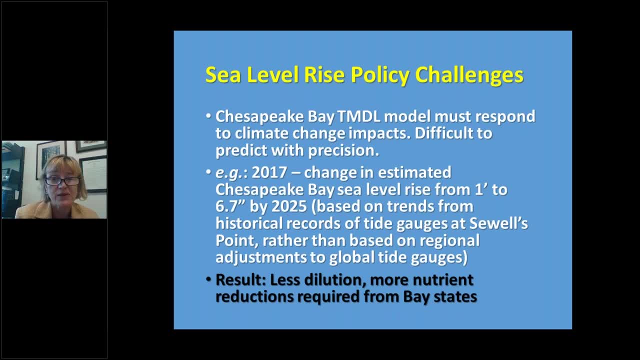 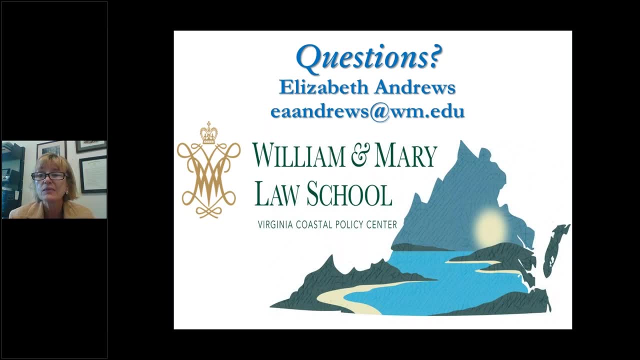 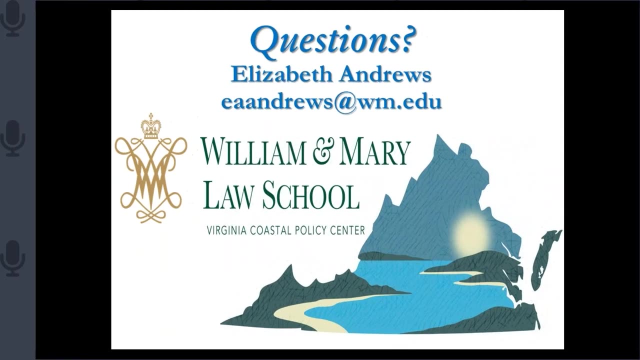 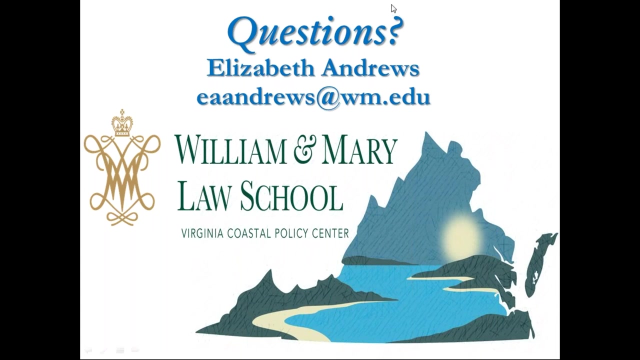 And the dollars spent to achieve the Bay TMDL requirements. And that's it for me. Can you hear me, Elizabeth? Can you hear me or no? Yes, you should be able to hear me, Elizabeth. She knew that I'm right there. 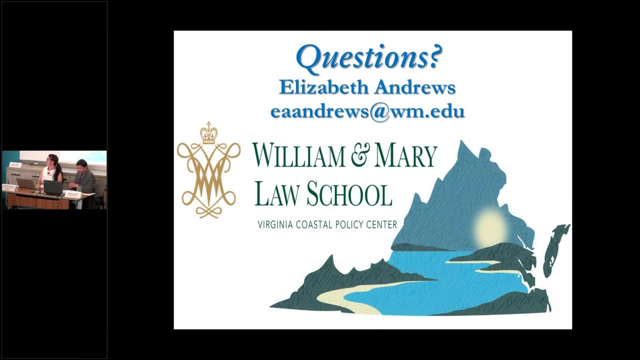 Okay, Wait, yes, I can hear you now, Sorry. No, I was curious about the idea of putting the treated water into a groundwater facility. right, Groundwater, of course, is where we get our potable water, So our drinking water comes from ground research. 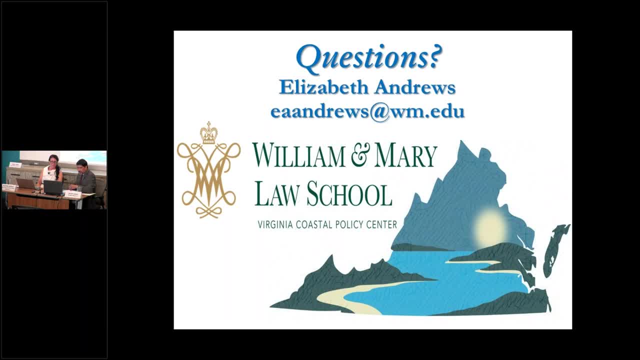 Is that something that was addressed or how? the impact of that, or I'm not? the SWIFT project this year? Yes, they're treating it. they are treating actually. they have a network of 11 different wastewater treatment plants. It's the Hampton Road Sanitation District Authority and they are taking that water. 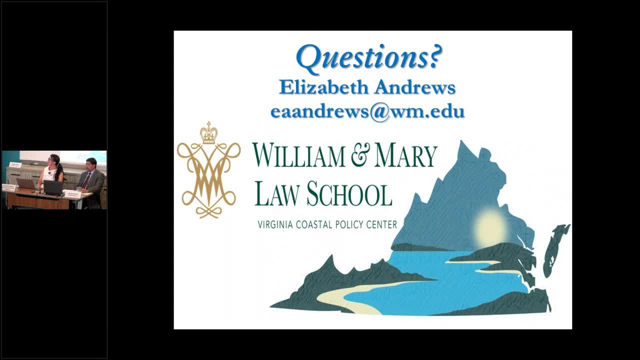 and treating it to a higher level, to a drinking water level. So it's potable water and before they injected it. but there is a monitoring lab proposed, et cetera. Okay, Great, Great idea, actually, All right. 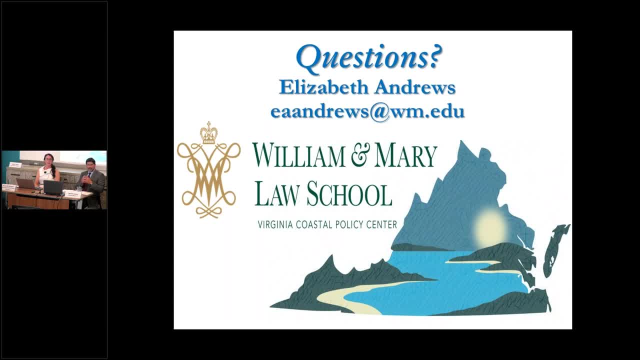 So questions from the audience? Great. Thank you so much to our speakers again for coming in both on the web and in person today. Now we're going to open up the floor for Q&A, So if you have any questions, please feel free to reach out. 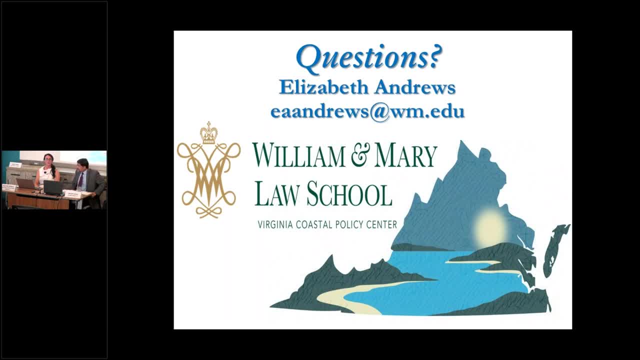 So if there are any questions from the live audience, we'll take those first. Yeah Great. So I have two interrelated questions. The first is what percentage of permits applied for under the Clean Water Act are actually issued, And the second is whether acquiring a permit is a particularly onerous process or if it's. 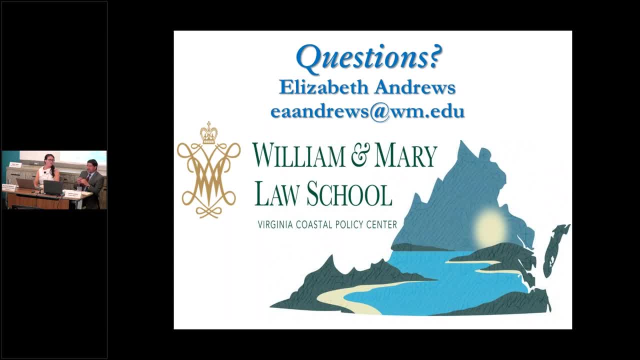 more about just sort of checking the boxes. Okay, Good question. If I understood it correctly- and I don't know that I can answer- however many people apply for a permit, how many people actually get it, which is a great question, which means: 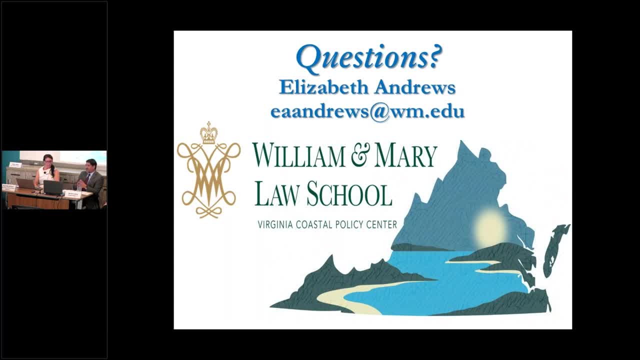 that if everybody gets a permit, of course the permit is meaningless. And how onerous it is to obtain a permit, I think varies. So I can answer probably the second question, which is it depends on what kind of permit you're trying to get. 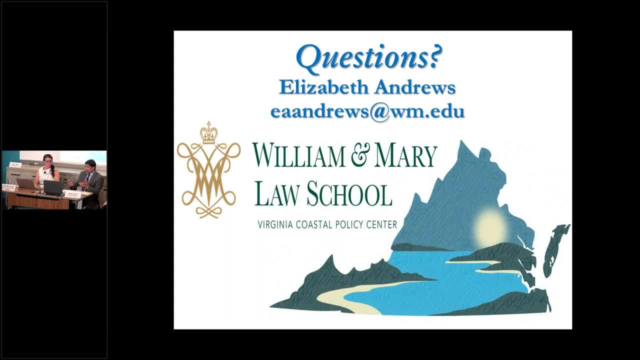 It depends on how well the facility is running. It depends on what kind of permit you're trying to get. It depends on how well the facility is running, For example- and Amanda can probably speak to that better. what I can answer is that 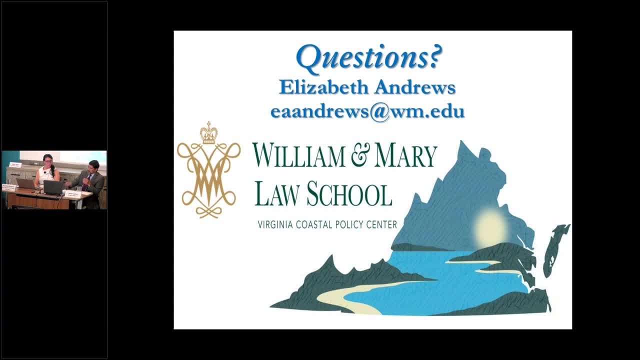 we do look at the permit as our way of enforcing when a particular facility whose permit is not complying with the permit. And Amanda brought up a good point, which is this is an onerous system. So, going back to your question, it is. 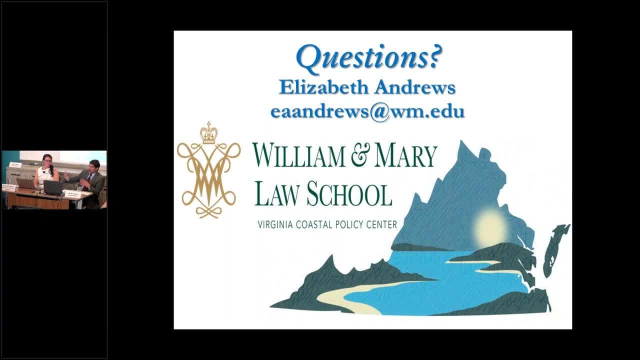 So we basically provide a survey. The EPA provides either a survey or an application. Okay, The EPA provides either a survey or an application. We've relied upon the individual or corporate entity to provide truthful information, accurate information, And the state or agency decides whether or not to issue a permit based on that. 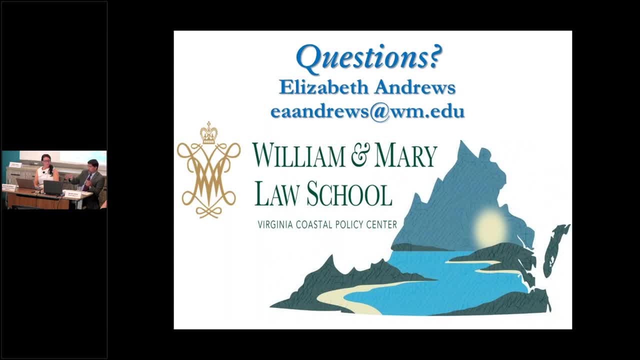 That triggers certain not only requirements in terms of following what you're saying, but also reporting requirements, And it can be onerous depending on how complicated the facility is, If you're dealing with a nuclear power plant, for example. though nuclear power plants are 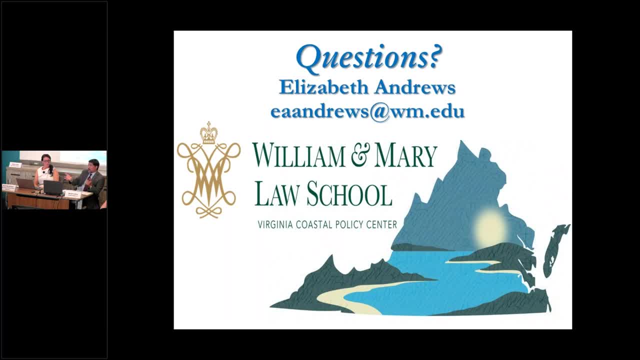 probably regulated by a different facility, but let's say, a pretty large wastewater treatment facility which will require a number of procedures and outflows and, depending on whether you go to the Chesapeake Bay, it may take quite a number of months before you get a permit. 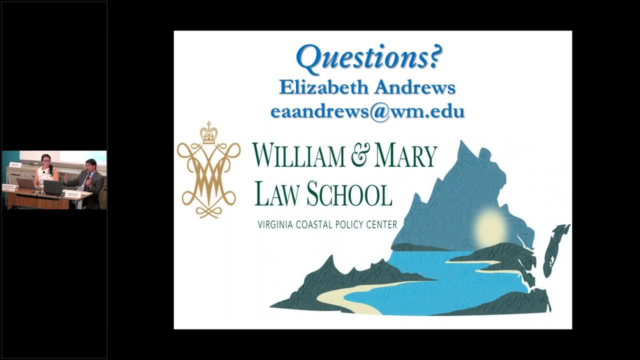 It may require some sort of working together with the agency. The things that you thought were going to work are not working, for example. there are ways to address that as well. I do not know how many permits are actually rejected. It's a great question. 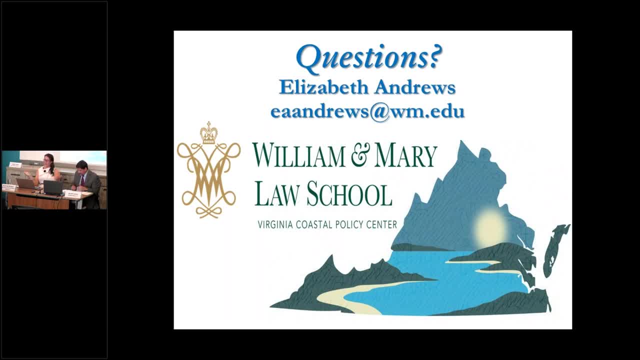 I don't know whether you have any experience on that. Well, if they're rejected, they're violating the Clean Water Act, So they're seeking a permit. if it's for a future activity, What happens is like in the 404 context, you've got somebody going out to propose to. 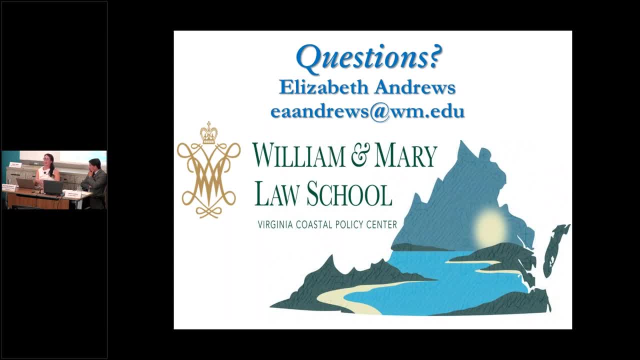 develop a plot of land, say they're going to build a house or a building, They apply for a 404 permit if there are jurisdictions And they can't begin construction until they get that permit. And in the 404 context I know that that was one of the biggest complaints and why initially. 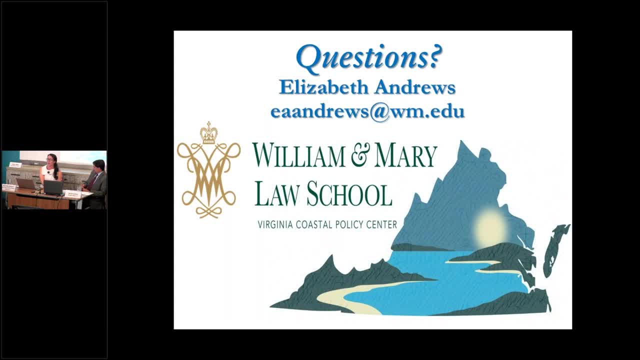 even the ones who now challenge the WOTUS rule wanted there to be additional clarification because the permitting was taking too long. It was taking years for an individual permit- 404 permit. When you're looking at the big traditional POTWs and big industrial dischargers, they've 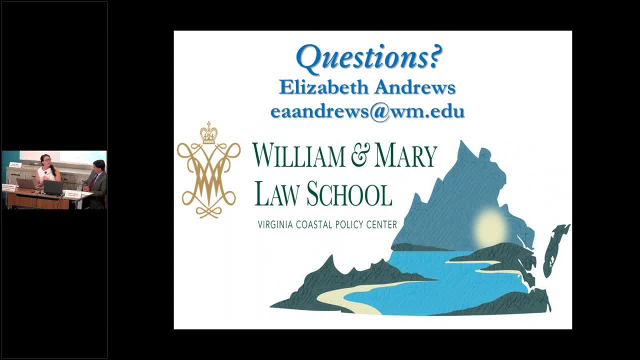 had permits forever. So you're in the renewal process, So I don't know. when you get rejected, then you either can't do something, but if you're already discharging, then you should have had a permit already, but in violation, yeah. 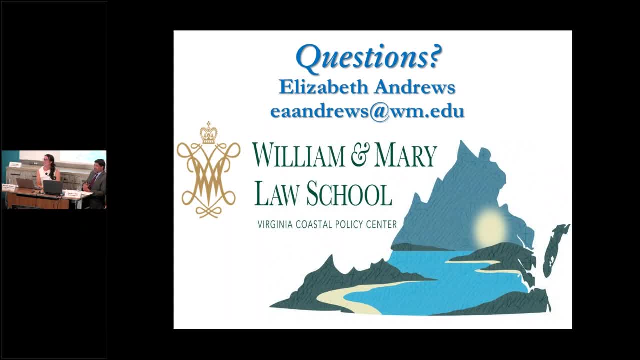 And you do want everybody who's discharging to have a permit, Right. This is Kathy. I'm sorry, Go ahead, Kathy. Oh, thanks, David. I just want to lob in here that there's a footnote in Rapanos that was based on a study. 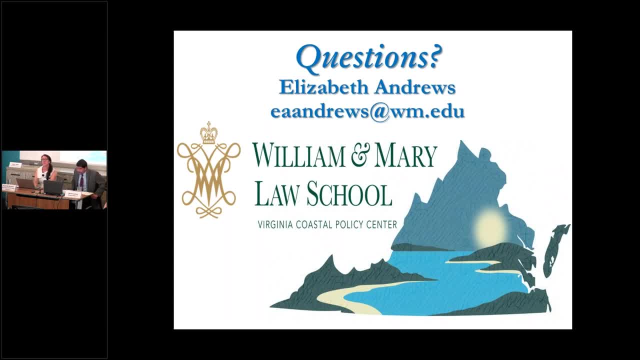 that David Sundin wrote. Yeah, David Sundin, who's a professor at Berkeley, did that, said in 2006,- and this is under the 404 permitting program, not the NPDES program, that an individual 404 permit was. costing. let's see here. Here it is. It was costing $271,596 and taking 788 days to get the average permit, And I'm not sure we touched upon this in great detail. but there are also a set of nationwide permits that one can apply for. 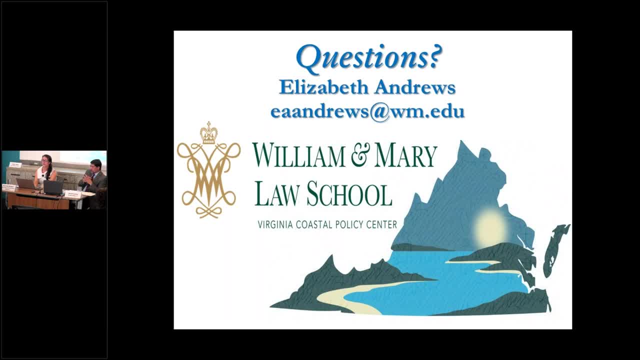 And if you fall within it, This reduces the time and the cost. you know they've just issued generic permits And if you fall within the qualifications of the nationwide permit you can reduce the cost of that. But even the average applicant under 404, under the Rapanos decision in 2006, was estimated. to spend 313 days And $28,915 on the nationwide permits, So there's not an insignificant cost in timing, And I don't have any data on the rejection level or acceptance level of permits. Great, Thank you. Anyone else? 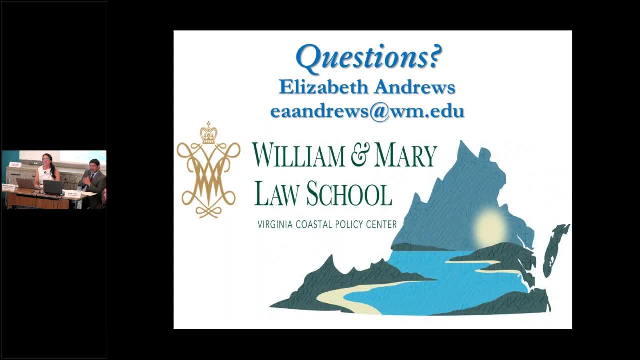 Hi, so I work at an historical research firm and will often work for law firms trying to figure out and identify like which parties were releasing pollutants into the water and like what type of chemicals they may have been releasing. So my question for you is: do you do like? does any of that historical activity matter? 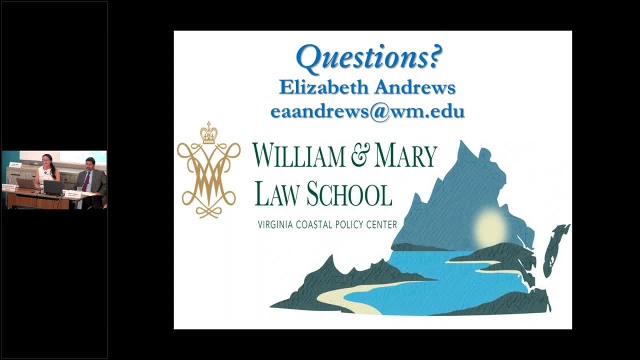 in the work you do, Or are you mostly focused on like present day discharges? So you're looking at some an entity that has stopped its legacy? pollutants- Yeah, Mostly I'm looking at pollutants from like the 1800s, 1900s and that's like been ceased for probably. 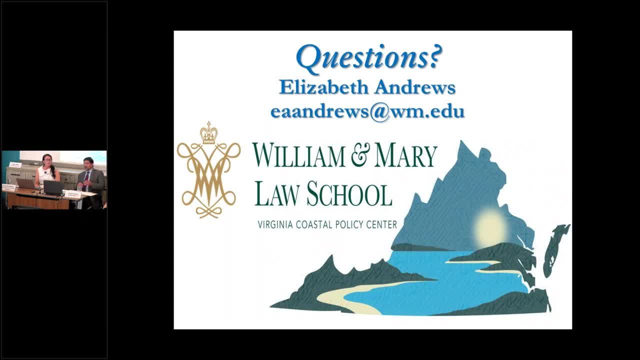 decades at this point. So I was wondering if that plays a role in what you do or not. really Good question. It probably would not be as much of an impact in the kind of work that I do in the criminal, because harm is not necessarily something that we need to prove. 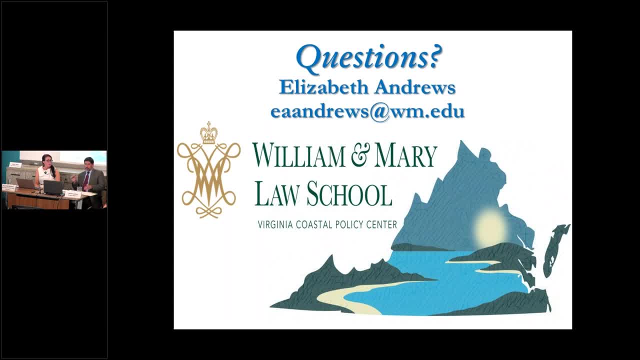 I can see how it would create a problem if you're trying to make somebody liable for pollutants And particular cleanups, which would be an additional cost, And particular cleanups which would be in a different program than the Clean Water Act. It is, though. 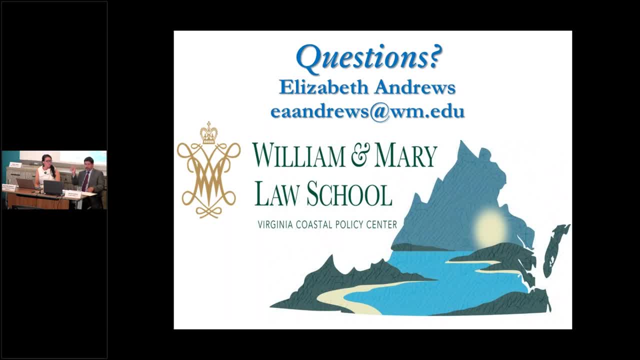 So we do consider, for example, if somebody is discharging and you're a down discharger, whether or not you're, some other individuals are contributing into the same watershed and are sort of: how does that affect the water quality standards? So I think it was Elizabeth who mentioned this idea. 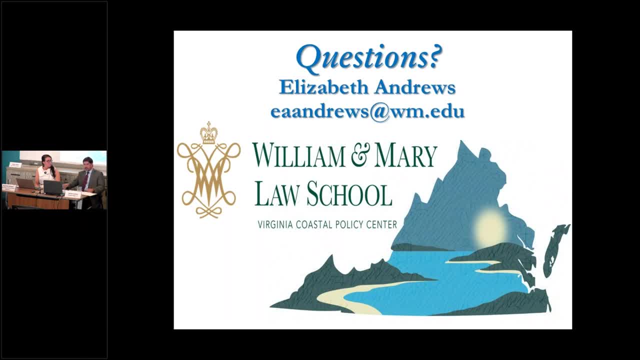 Yeah, I think this idea of whether discharges are affecting the water quality and whether we can bring in enforcement- I can see how that would make- could be an impact, because you need to address who else is polluting and how significant my discharges are in comparison to others. 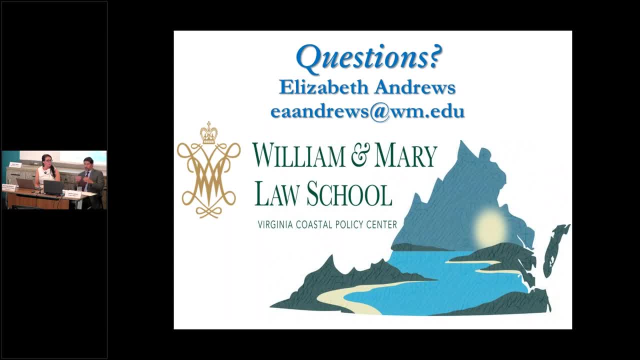 You're up from a significant, categorical industrial user that pollutes, that sends toxics to the particular watershed, and you're only dealing with somebody who's as much Smaller polluter- perhaps only does a small amount of pH, lower pH, or something like that. 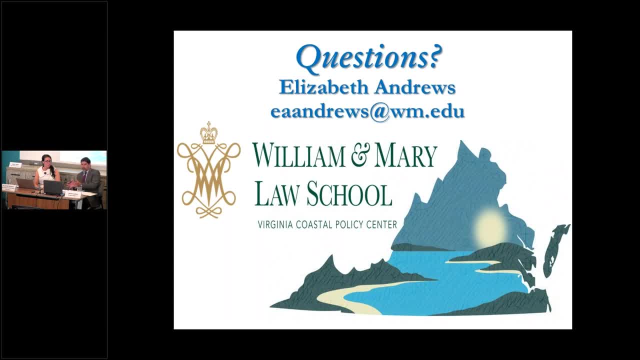 Or then it's kind of unfair to treat this individual different without considering whatever everybody else is contributing. If it, historical though it's, I'm sure we have the analytical data and it's something that the agency is probably looking at, but mostly to make sure that we don't degrade. 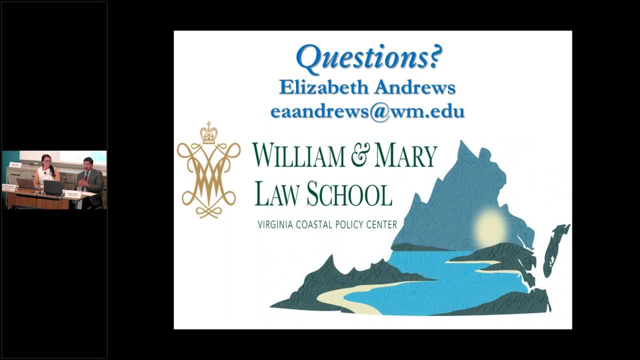 the particular watershed, Probably more. I'm sure scientists would look into those in order to consider how, what kind of impact you would have because you have certain background levels. But other than that, not in the kind of enforcement that we do, because we deal with the polluters. 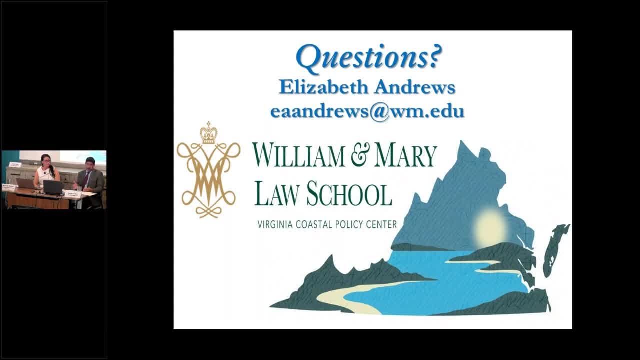 that are discharging- I mean we, sometimes, many times, we do historical cases because we bring an enforcement action, The individual stops polluting, but we still, they're still liable for those discharges that were unpermitted, Knowing or negligent. 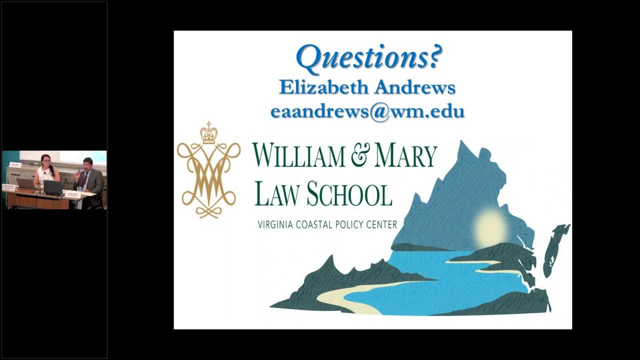 And then deciding what kind of fine we would address or if we recommend for the judge that may be an issue, or a defendant can bring an issue- that the owner is unfair. You know, I do not deserve a bigger fine because this watershed was already polluted. 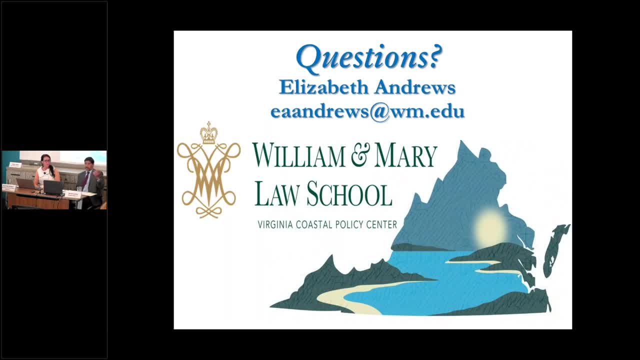 And we've had those arguments before in many cases where they say it's it's such a big day, It's already polluted, Why is it such a big deal? And our argument is absolutely precisely: because it's already polluted. It's already polluted because it's a big issue. 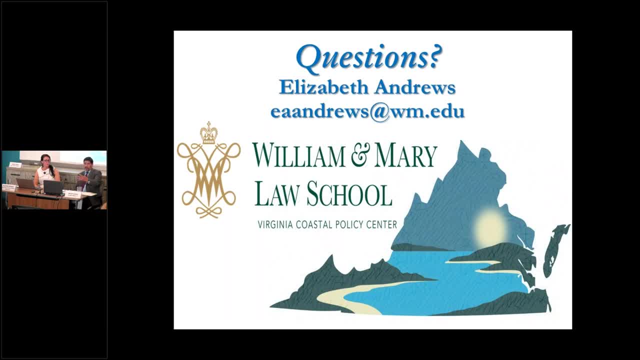 You're doing. you're actually doing more harm. But I can see how they can argue to the contrary, saying you know it's unfair And then you address it with a judge. ultimately, or either a consent decree or a plea agreement. 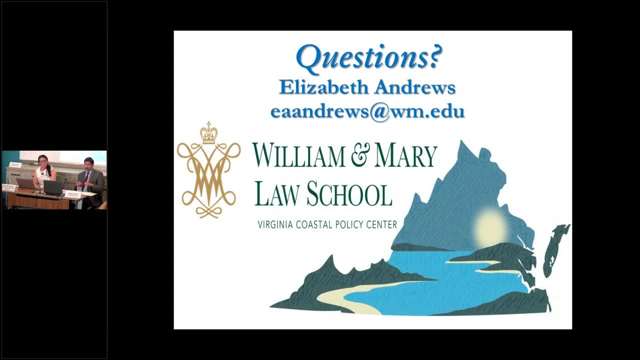 depending on your civil or criminal arena. And I can- I'm sorry, I can. I can give you a case study from the municipal perspective. It's New York City, So they have the Gowanus Canal. It's got legacy pollutants. 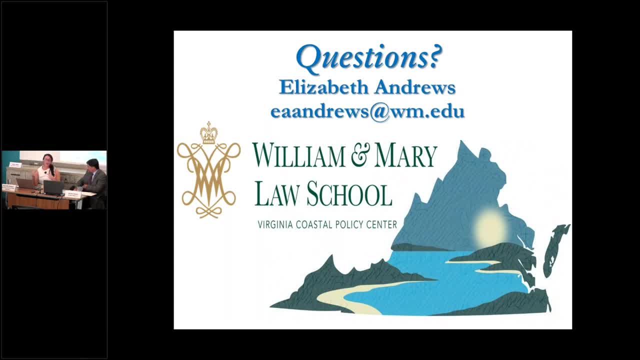 I'm not sure what's in there, but it's a. it's a Superfund site. So they're dealing with Circula and a different office of EPA to deal with that, because they're a PRP Potentially Responsible Party. And then they're dealing with a clean water side with their combined sewer overflow reduction. 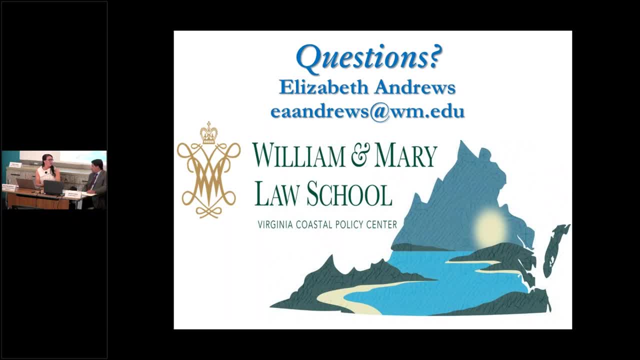 projects And the requirements don't always like advance the common purpose, So they're spending money here, spending money there. So that's where it would come up for for cities if if they're dealing with these legacy pollutants that they could be potentially responsible for. 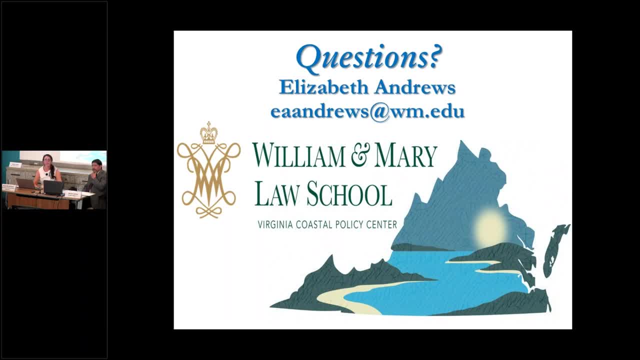 And they'd have to then consider that as part of the Circula cleanup Right. I think that's probably the more better context. Anybody else? Great, Thank you. Okay, We'll take one more question from the site and then we have a couple of questions online. as well. I I worked for a consultant firm that is helping a Maryland agency with complying with their NPDES MS4 NPDES permit. that's issued By the Maryland Department of Environment and approved by the EPA. So one of the requirements of their permit is when MDE issues a new TMDL for the state. 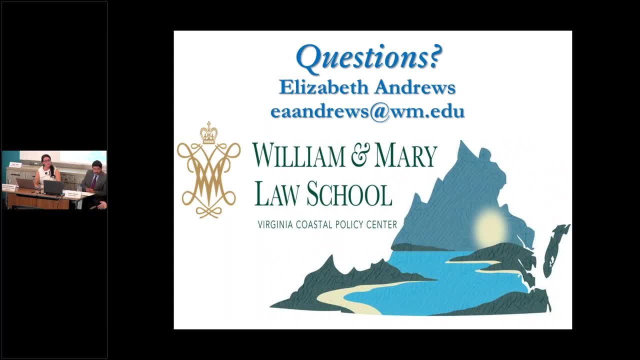 of Maryland and EPA. when EPA approves it, the agency has one within one year, according to their permit to write a plan for that TMDL. So what I find difficult is part of our Okay. So this is looking at the TMDL. sometimes MDE will write their TMDLs and define their 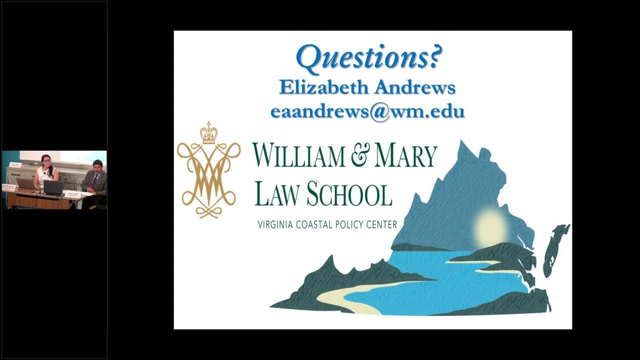 watersheds based on their own eight digit watershed system. So that's how. that's how Maryland puts it. Each one's an eight digit. you know, Bush River is eight digit. this you know, and other times they'll flip and they'll do one that's written to the segments based on the Chesapeake. 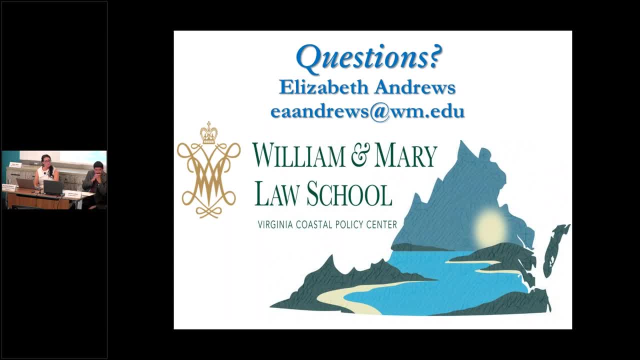 Bay, I believe- program And I'm wondering: is there- and I re what I'm thinking is the The reason why the segments were put into place? that system was so all the states that are tied to the Chesapeake Bay TMDL could have a uniform way of referring to them. 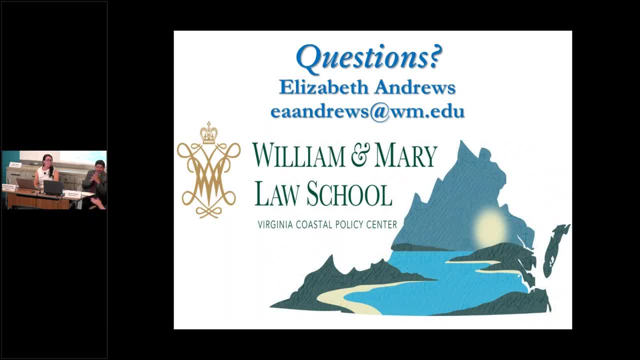 Is that correct? Okay, I just wondered why they flip back and forth. and is the is the movement to try to get maybe MDE eventually? maybe some of the not so much for their watersheds out like west, that they don't, that aren't tied to the bay necessarily, but for the ones around it are. 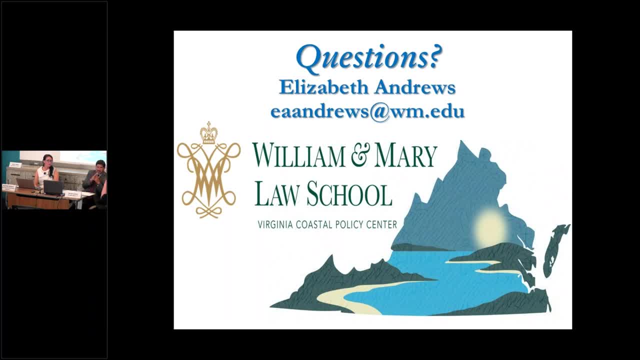 they trying to go to just writing towards the segment scheme. So then all the states understand: versus this eight digit. Okay, Yeah, It's a way of delineating it differently. Yeah, Right, It's because when they're looking at the HUC, when they're looking at the watershed, 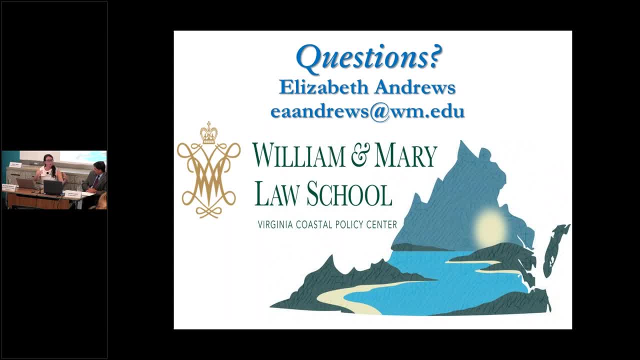 that is, that is typically what I've seen and that is the best way to do it, because you're looking then at: well, that's intrastate water body where they can look and control all the pollutant sources with the Chesapeake Bay. 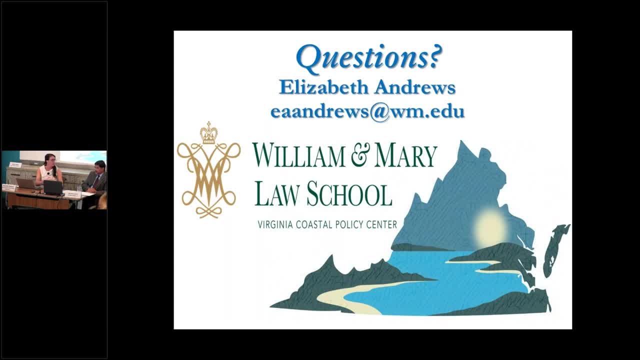 You're dealing with many states interstate waters and so maybe they're they're just doing that for So it's consistent with other states on Chesapeake Bay, But what I've seen is that you'd have it on a watershed basis, sort of that. that's how. 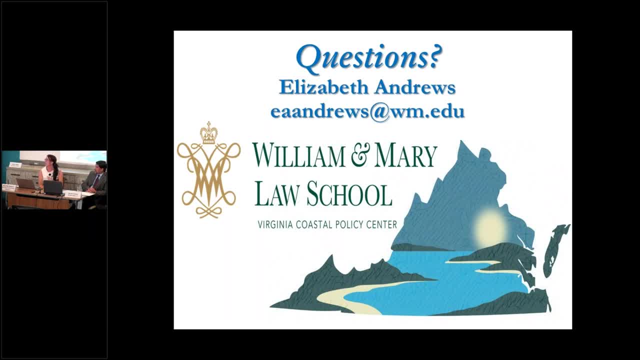 you would make your determinations, but, Elizabeth, I don't know if you know more about how Maryland is doing there. No, I'm not the pro on Maryland, unfortunately, but I will say that I think that at times they do try to echo the segments as set forth in the Bay Team Deal overarching requirements. 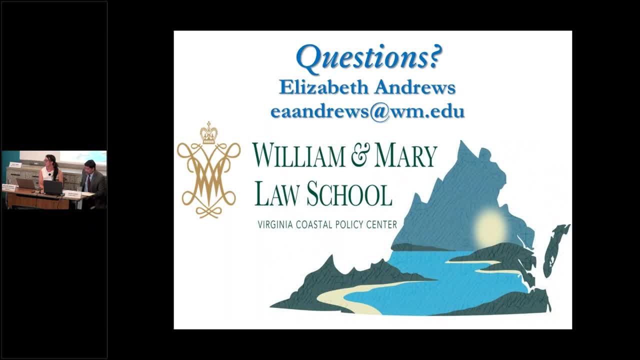 but sometimes a situation can be driven by state code, Like the eight-digit HUD code. if it's talking about trading in the stormwater context, you know, or nutrient offsets, that kind of thing, then sometimes that can be driven by a state. 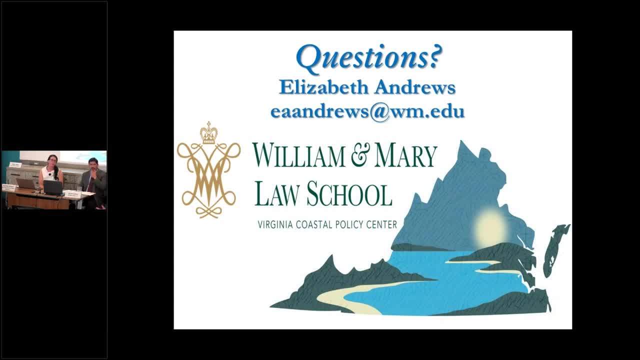 code provision as well. In the end, it really doesn't matter, because what we do is we take a look at the actual area, Whatever's in that area, whether you're this watershed, that you were part of an eight-digit, or whether you're part of the segment, what we call the segment shed, the watershed associated. 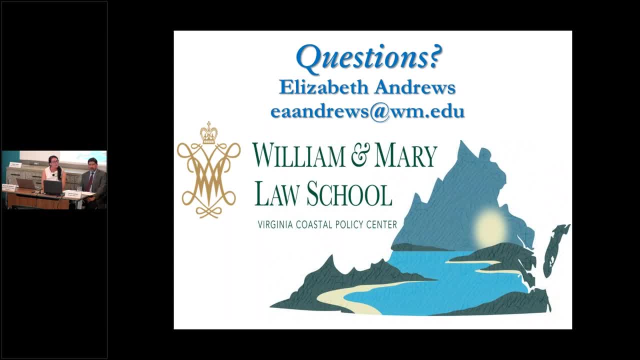 with the segment. It all- yeah, it all comes together Right. It's just interesting. What I would say is: Nolan, it's a great question. I think it's something that you want to post to the Maryland and to the EPA in a narrative. 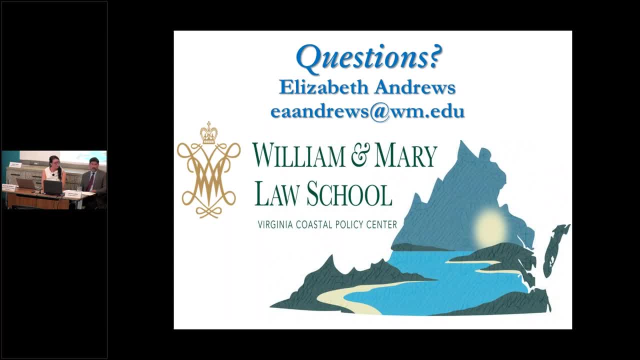 way so that you can actually address the issue and they actually are responsible to- and this will be sort of somewhat of a FOIA request, if you will, but the idea is that it's important for the agency to know your concerns and I think it's a legitimate question that you 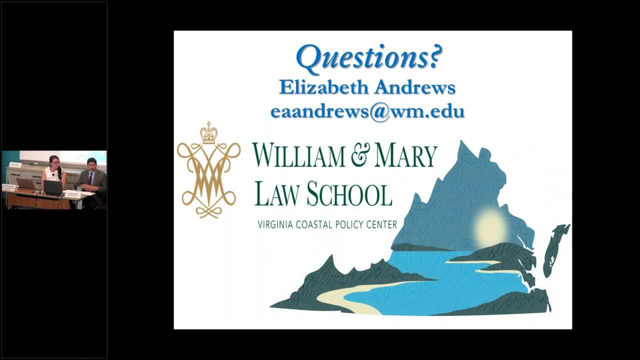 should get an answer to. Yeah, I'm just more curious, Right? If you just ask them the question, they'll just be like: oh yeah, we do it this way because of X. Right, Then I'll understand, Right, right. 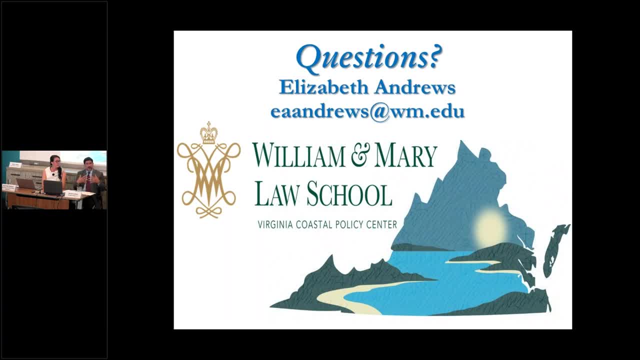 It's just more of a curiosity. It may be that they're not looking at it if you're looking at it from a different perspective. they're not looking at it from you. want to have them put themselves in your shoes and say, wow. 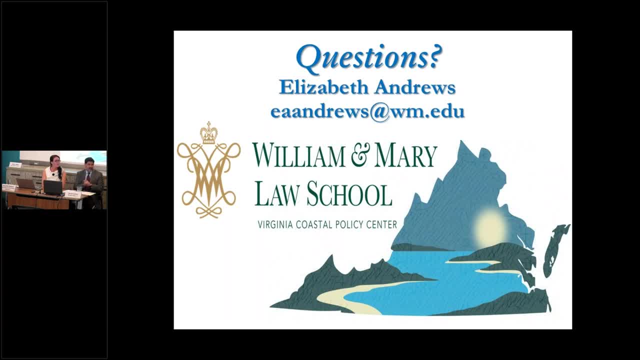 Right, having to figure it out, Right? Yeah, It does have meaning to you and it should have meaning to them. Yeah, Yeah, That's a good suggestion, Except they'll do it by FOIA. Good suggestion: Working for Tuesday days. we'd rather you just call and ask the question. 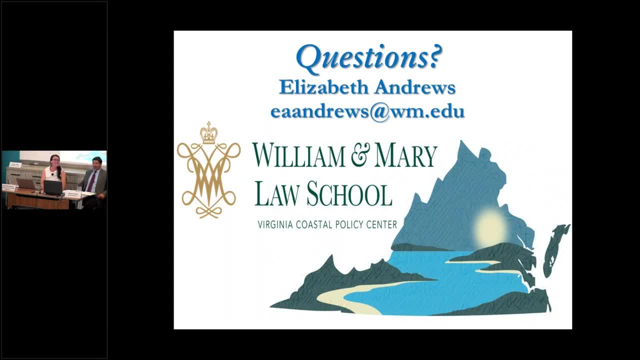 Yeah, I was going to call, I was going to. yeah, Thank you, That's a good suggestion. Although our questions are always addressed, Any question will be addressed as a FOIA question. so, yeah, it's yeah. 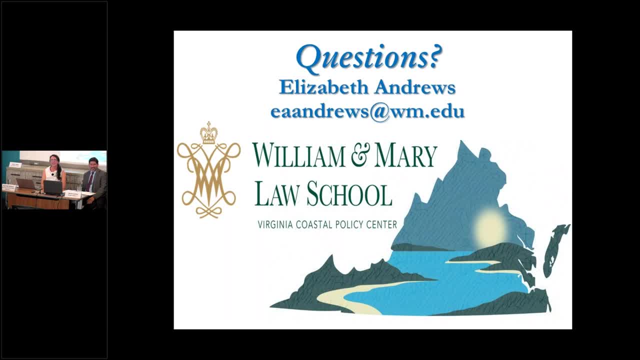 Okay, Thank you Great. Thank you so much, guys. Next we'll move on to some questions from the web. One second, All right. So do the panelists have reflections on or experiences with potential additional complexities of interstate water quality management initiatives such as the Chesapeake Bay? that might also 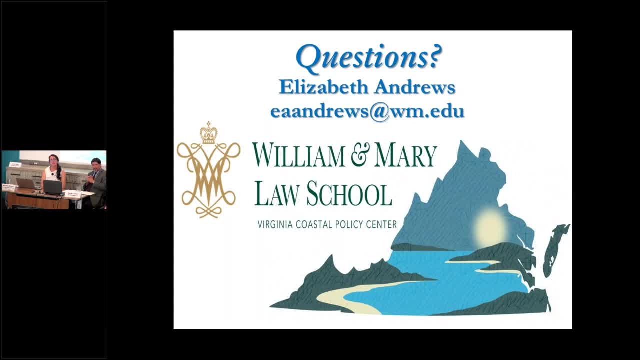 involve tribes with treatment as state-dependent. Yes, Okay, Elizabeth, would be the one. Elizabeth, we're hoping that you can answer that one. This is totally unfair. I'm not there to defend myself. Well, we in Virginia are lucky to have a number of tribes that just were federally recognized. 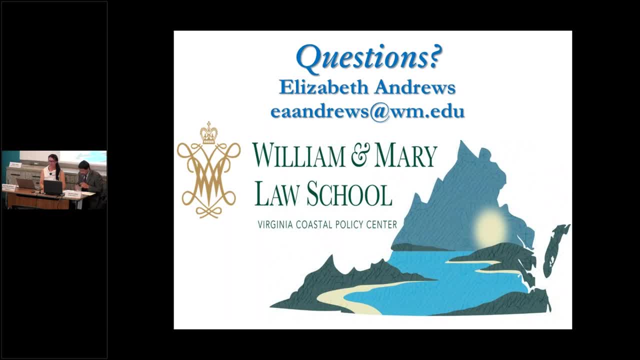 so I'm thinking- that's why you lobbed that over to me, probably- And I would say that right now, honestly, a lot of people are trying to determine what exactly that means and how best to work with the tribes. Okay, We have two tribes with traditional reservation grounds. 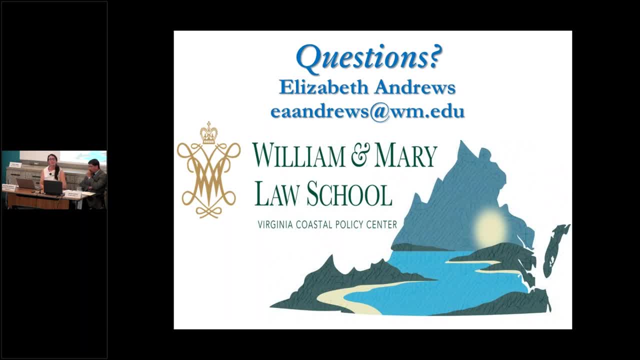 So they are. I believe- and David could speak to this better than I, but I believe they're speaking with the EPA about the water quality permitting in those situations, but separate from the state. But yeah, I think that dealing between states and tribes that have been federally recognized, 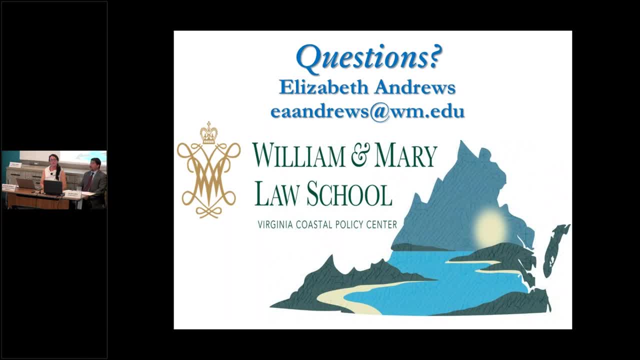 is going to have to be an effort that is similarly creative and flexible as it is with the interstate Chesapeake Bay agreement. But we're just at the very beginnings of those discussions, Right, And I do believe we have communication with the tribes, certainly in Virginia. 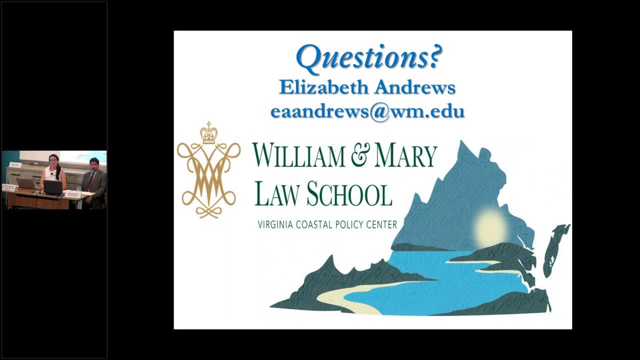 I'm not familiar with what the communications are, but I am aware that they are communicating with it. Okay, Great, Thank you. One more question from the web, from Jess Walker. Could you briefly elaborate on how TMDLs for pollutants are developed and then reevaluated? 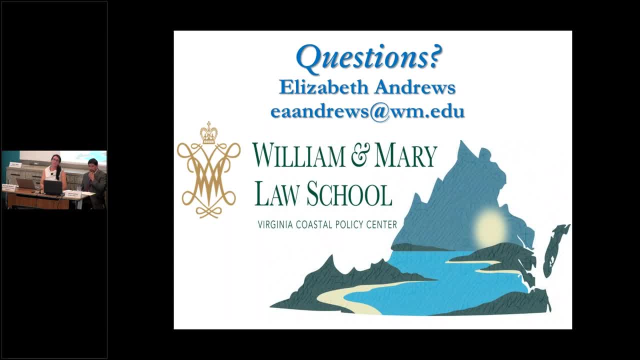 and updated, And specifically how frequently? How frequently are they updated? Good question: Yeah, Elizabeth, Yeah, Well, actually I don't. that's a good question. I'm pausing to think, if I can pull that out of my brain. 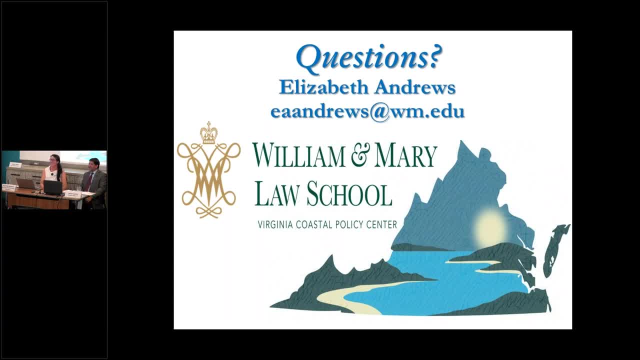 I don't know, without doing a little research on how often that they do it, but it has to be done periodically, in the sense that I will say this: that the waste load allocations- as I think it was David who first set out the formula, you know, the WLAs plus, LAs plus. 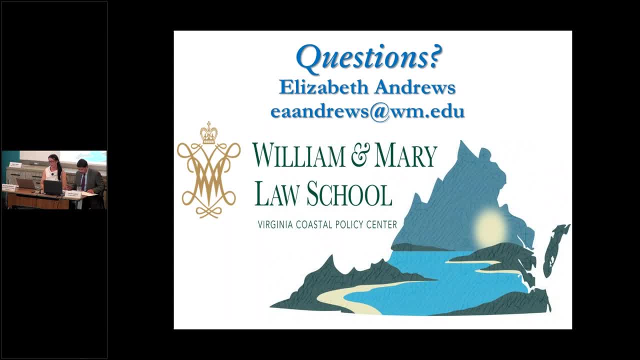 the margin of safety Right, And so you have. and we have that problem here in Virginia where they allocated fully the waste load allocations, for example for the James River, And then when new development comes, that's a serious issue. How are you going to accommodate that? 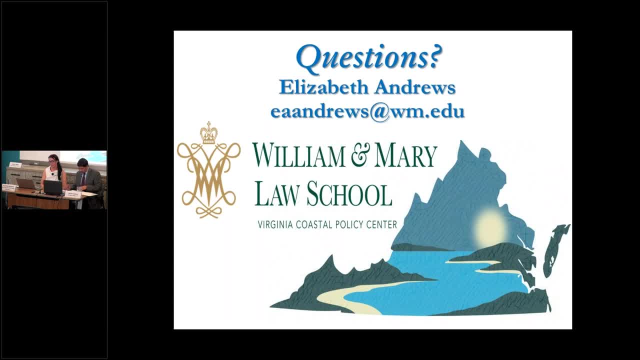 And the answer is: you've got to figure out whether it's a waste load allocation trading system and a or retraction of old waste load allocations that aren't used, but it is capped. There is a formula, But the There are other factors, such as climate change, that could probably change those original. 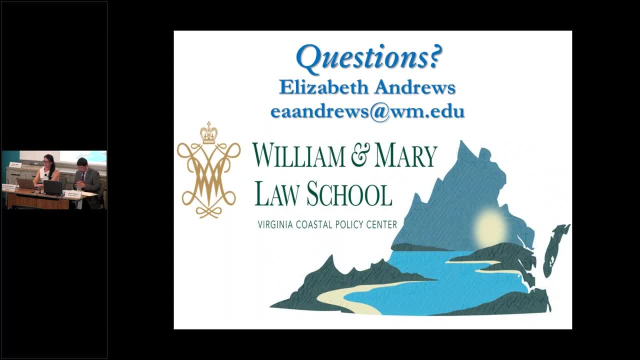 numbers, since they would have to be revisited periodically, but I'm not sure what the schedule is. I know for the Long Island Sound TMDL it's five years, but that was developed in 2000 and EPA has not yet actually reviewed and revised it. 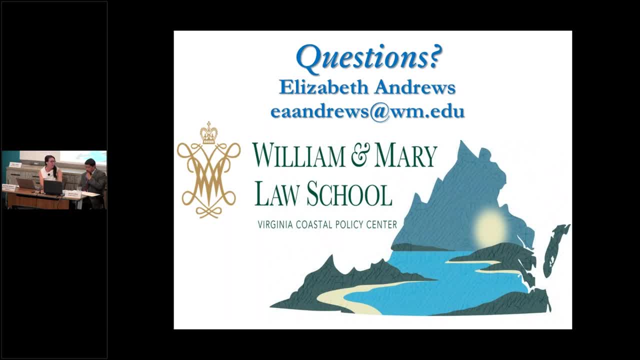 So there's no real. they say that they'll review it every five years, which it would be a good practice, But there's no real mechanism to force EPA to do it Right And EPA obviously has the enforcement or the oversight. I want to say there's a provision about two years that you have to provide in advance. 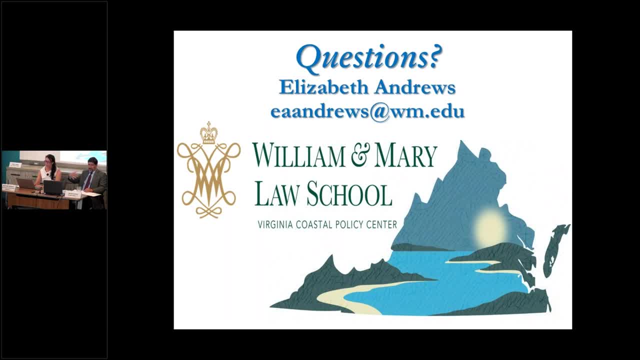 of when the TMDL is going to be implemented, but I don't know that there was a specific provision on the how many years would it be in and how it's revised. I was trying to look at the particular section. It's 303,, I believe.